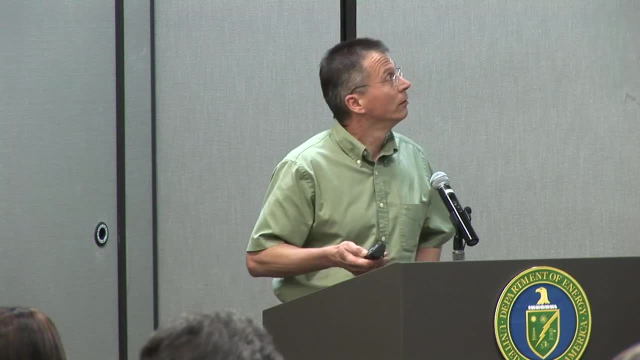 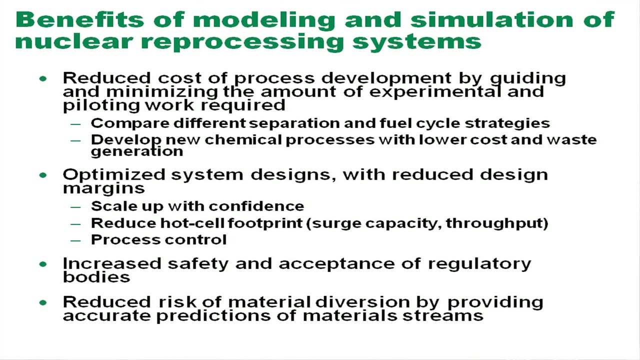 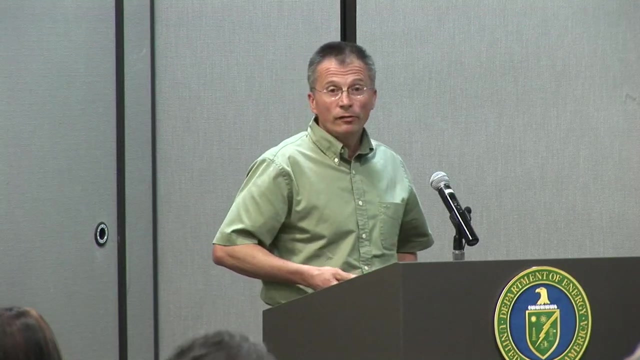 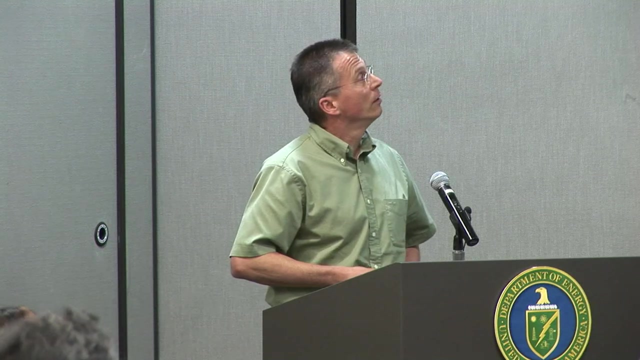 the development and implementation of these processes. Modeling and simulation can have many benefits: reducing the cost of R and D, for instance. minimizing the amount of costly experimentation by allowing you to compare different separation processes, different fuel cycle strategies. developing your chemical processes with lower. 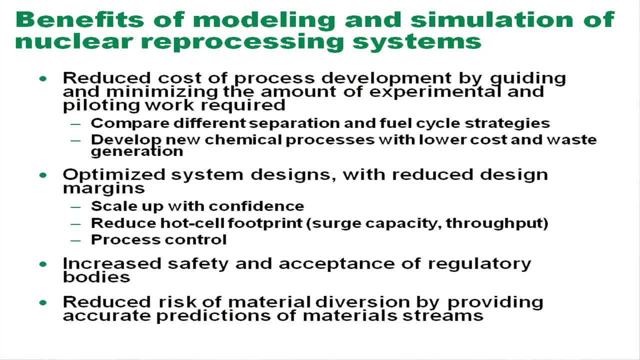 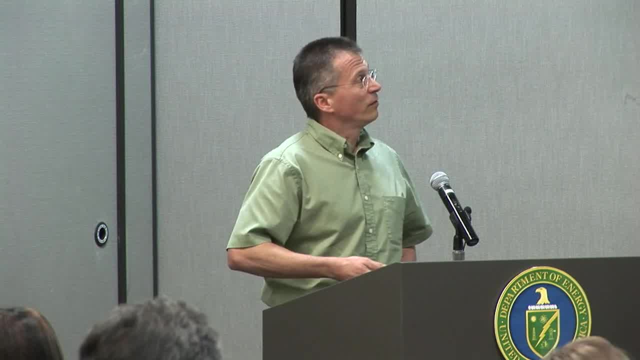 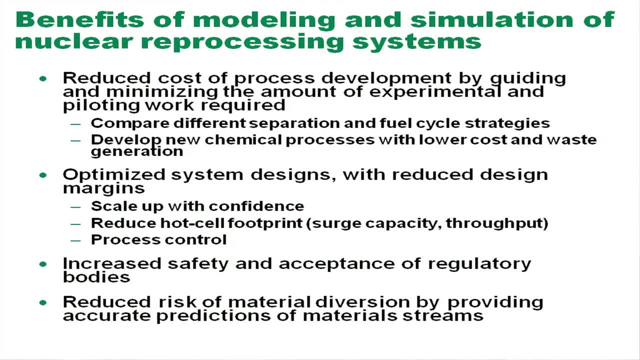 cost to accelerate the work. When you move on to system design, you could use models to help develop designs with reduced design margins, allow you to scale up with greater confidence and increase safety and reliability And perhaps acceptance of regulatory bodies if you can then fully explore different operating. 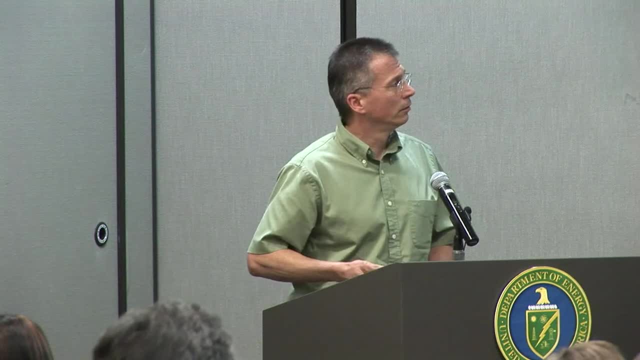 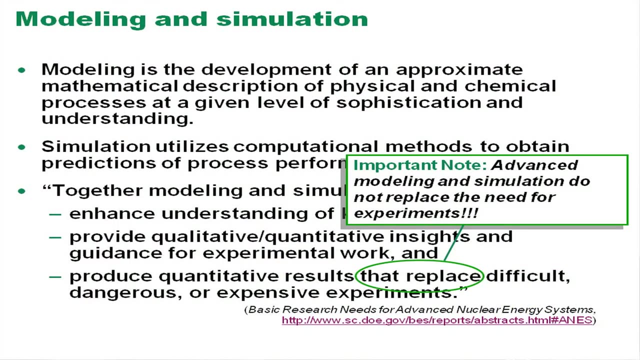 spaces with models. Okay, so just stepping back. What is modeling and simulation? You hear this a lot: Modeling. a lot of people do modeling. If you sit down and you do a little Excel spreadsheet, you're doing modeling because you're basing. 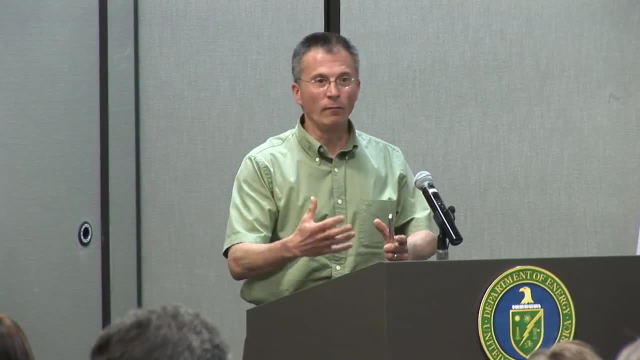 You're taking reality and changing it into some sort of model of the simulation, And you're doing modeling because you're basing. You're taking reality and changing it into some sort of model of the simulation, And you're doing modeling because you're basing. 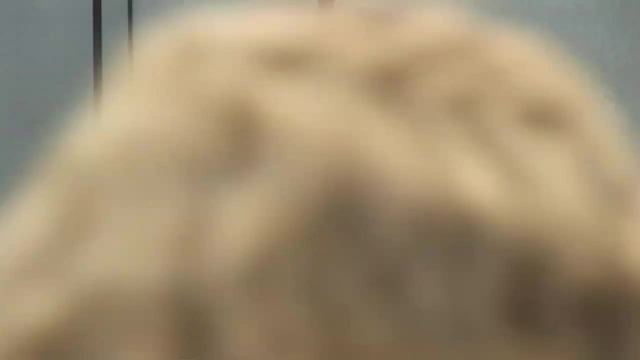 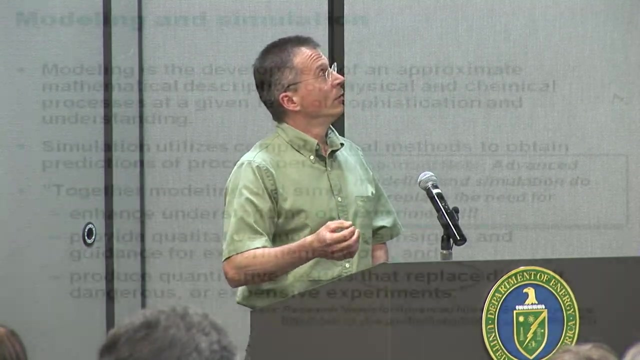 You're simplifying the system. You're simplifying the system. Modeling is developing an approximate mathematical description of something more complicated and then developing it at some level of sophistication that it's useful. Then simulation utilizes computational methods to obtain predictions of the process performance. 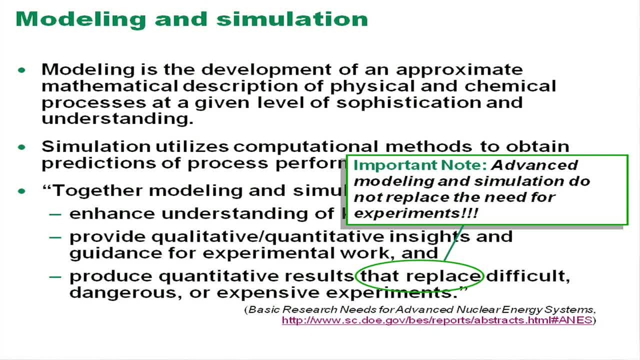 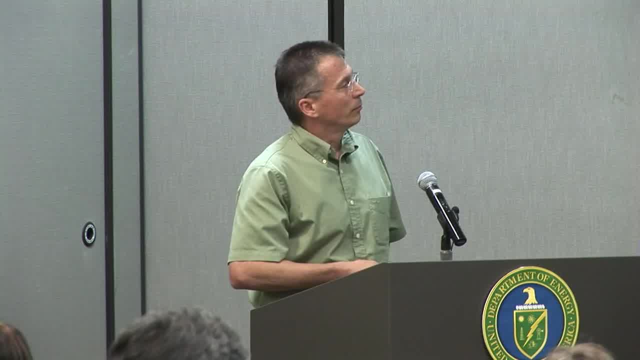 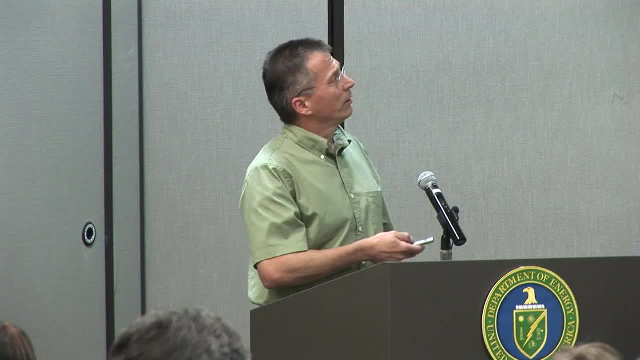 So a lot of people do modeling and simulation. Here's a quote here on the bottom from the ANES report, The BES report. This is a report on nuclear energy systems from a few years ago And they say modeling and simulation enhance our understanding of known systems. 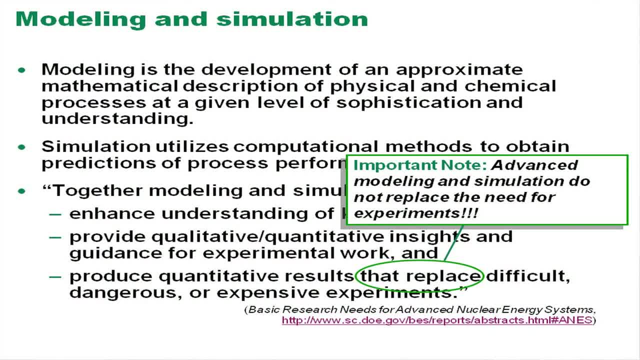 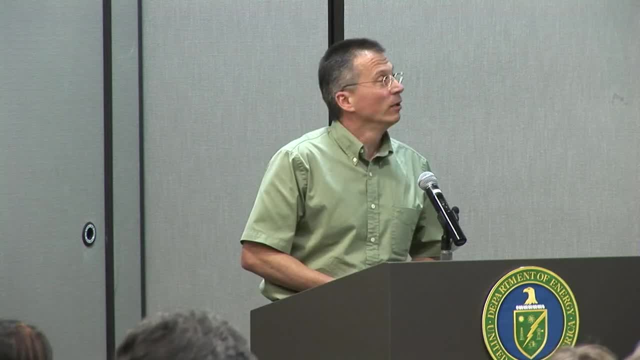 They provide qualitative and quantitative insights, guidance for experimental work and produce quantitative results that replace difficult, dangerous or expensive experiments. And this last bullet is a little bit dangerous, Very much want to say. advanced modeling and simulation do not replace the need for experiments. 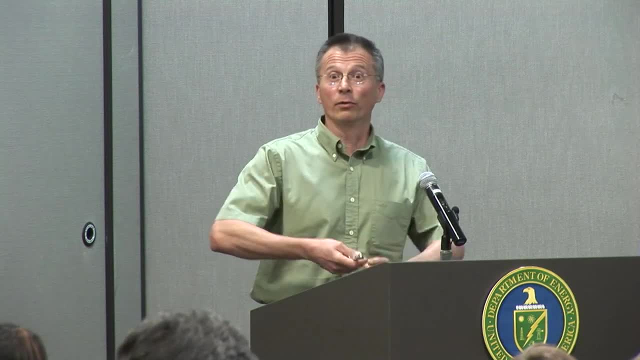 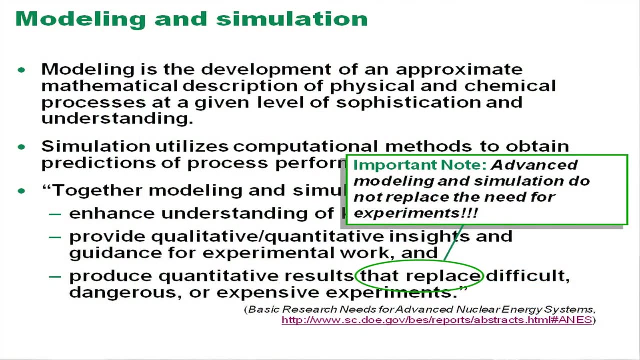 You will always have to do experiments. experimentation both to get the parameters to feed your models, but then also to validate the models. I noticed in the slides as we move ahead in the course- I saw the quote- that all models are wrong and some models are useful, and that's absolutely the case. 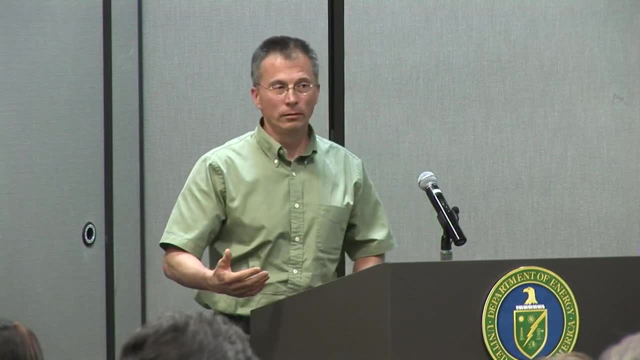 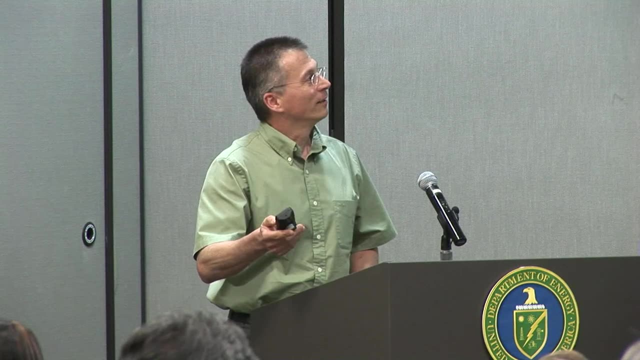 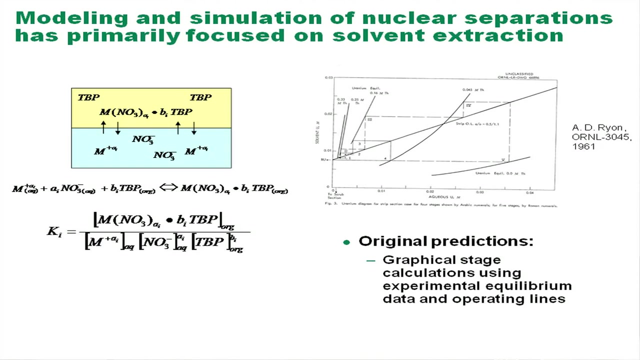 We have to keep that in mind. Models are useful tools, but they're not, you know. you still need real data for your modeling. Okay, so modeling and simulation of nuclear separations is primarily focused historically on solvent extraction, because that's where the bulk of the separations is in aqueous. 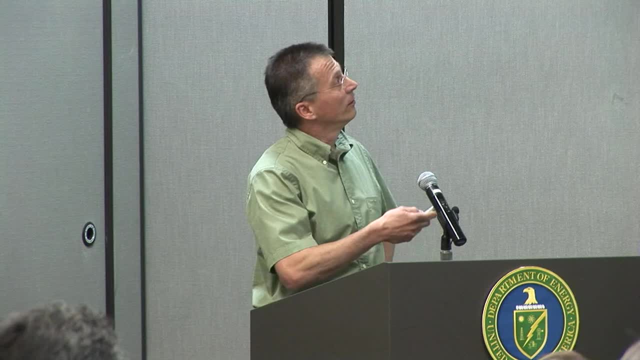 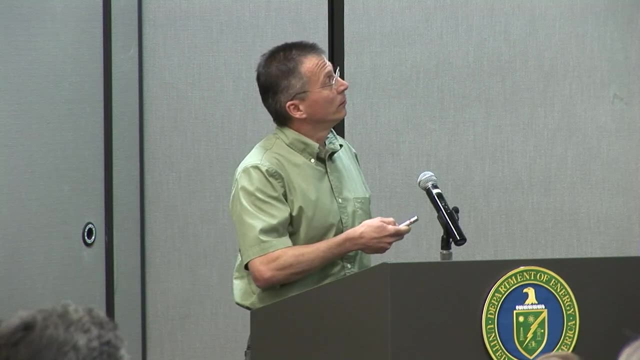 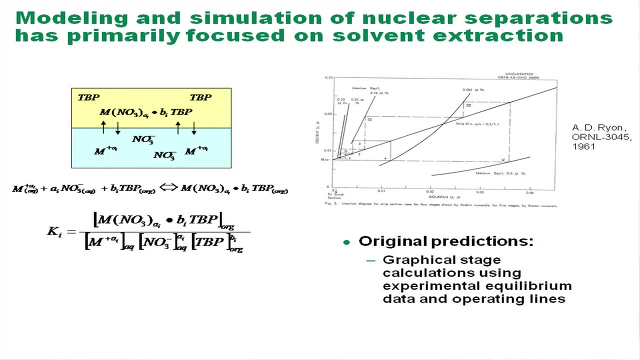 processes and you've seen, you know basically what happens in solvent extraction in earlier talks, where you're looking to take these target species and capture them in a solvent and you can write kind of mass action, You can set up equations for this process and then you can set up, you know, an equilibrium. 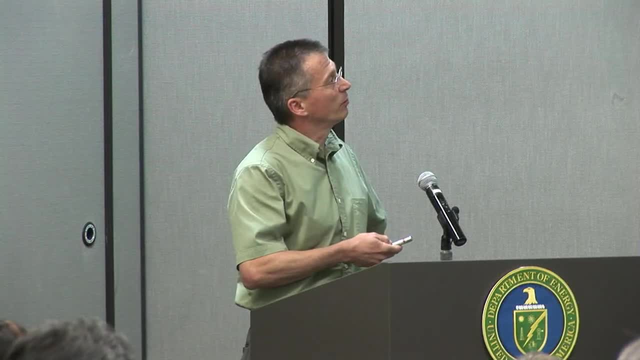 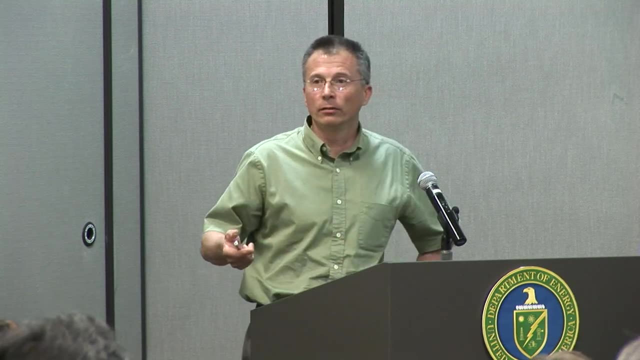 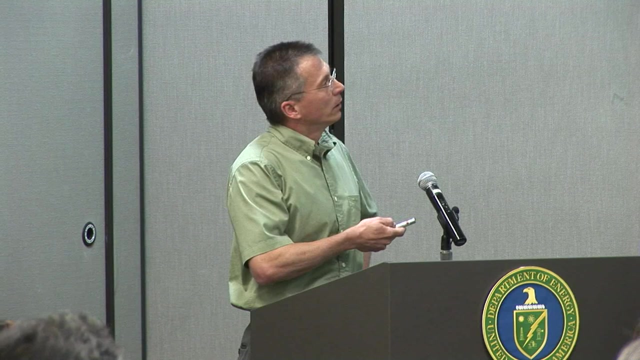 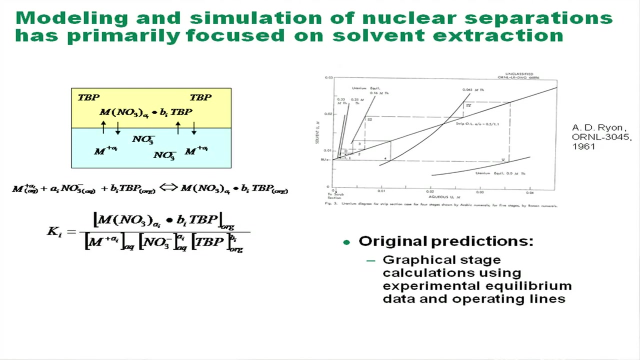 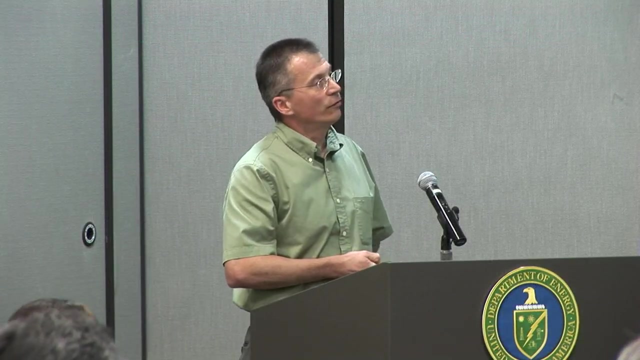 relationship, which basically products and reactants, and put the coefficient on each of these. you know, like you did in your chemistry classes, And so here this can be used to explain the relationship of an equilibrium in a solvent extraction process In the past. here's an example from the 60s where this was done. 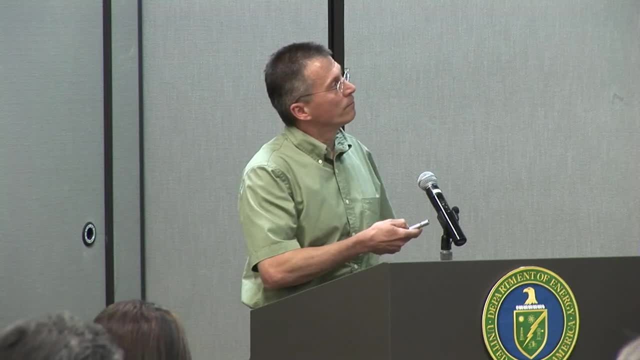 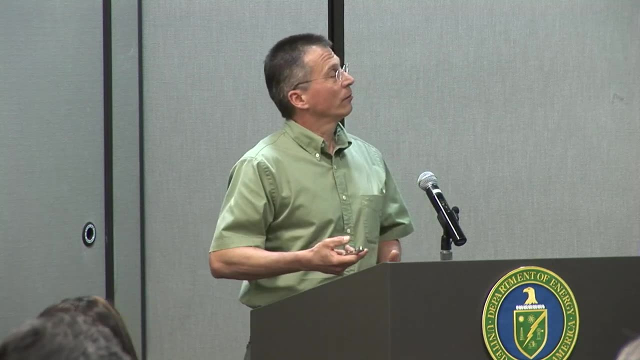 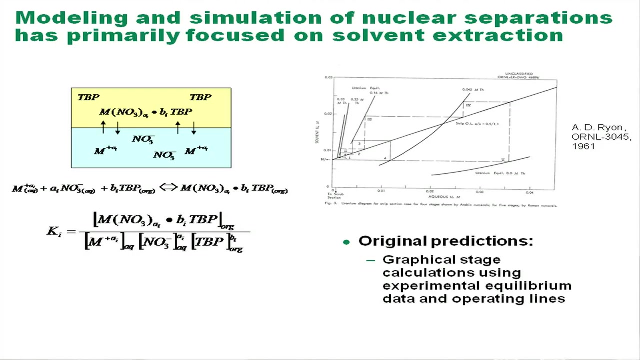 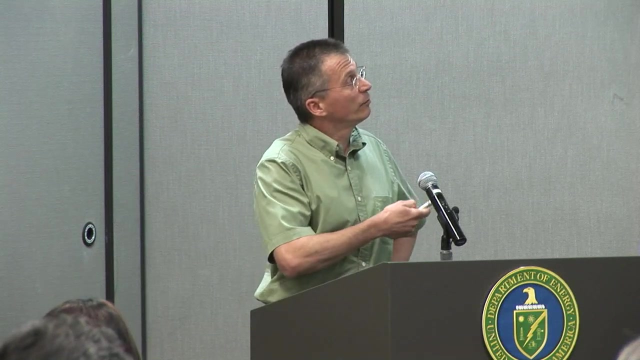 You get experimental results for the equilibrium relationships and then you have operating lines for your mass balance, And so originally the solvent extraction process is predicting how you're going to move the species in your system was done graphically, using just graphical approaches. 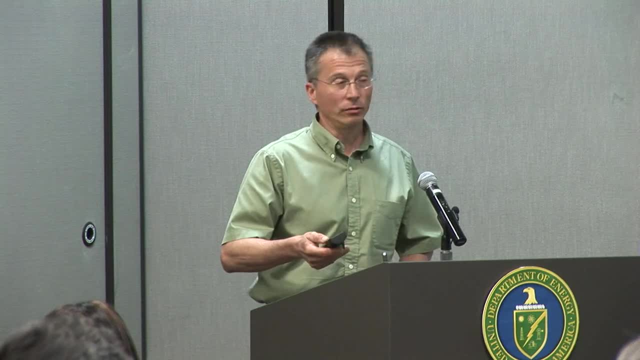 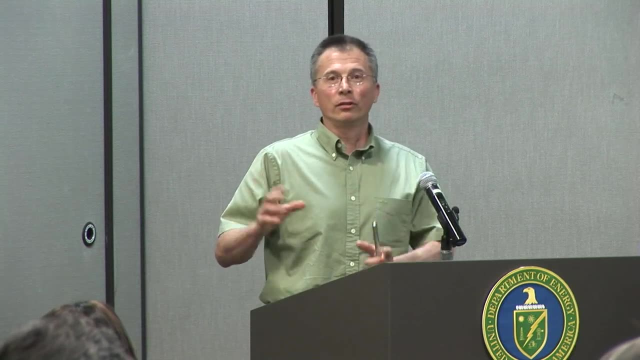 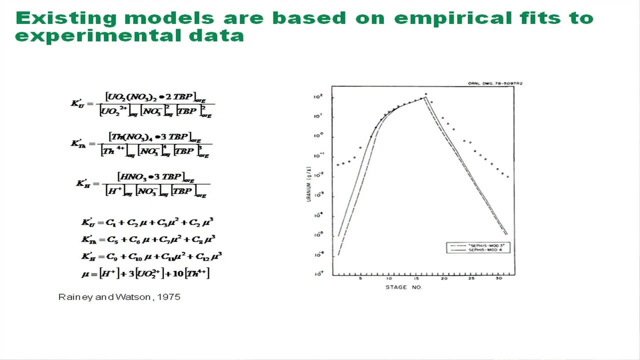 And then, since then, we've taken and translated this to computational approaches. Now, what complicates things are that simple equilibrium expression. Nothing is simple, Everything is non-ideal, And so if you move forward to, here's a model from the 70s where again they're doing these equilibrium relationships. 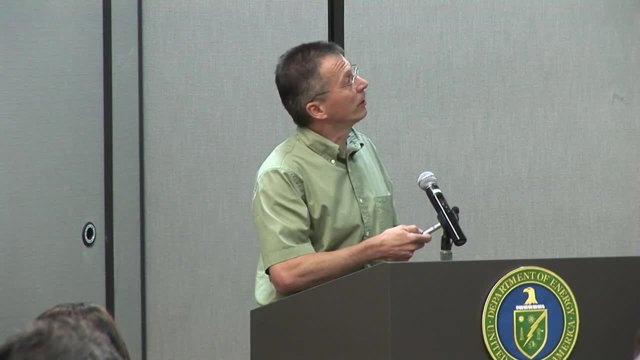 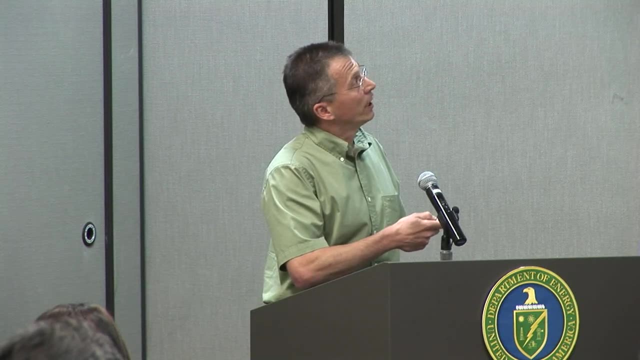 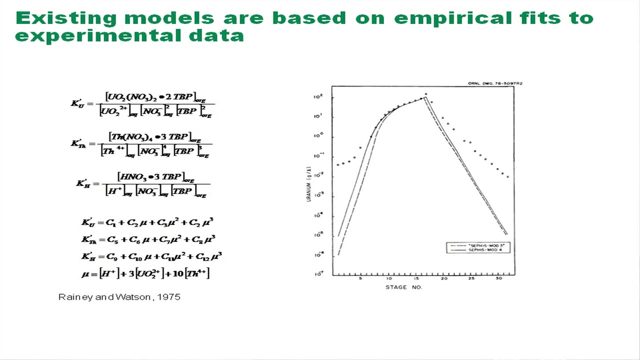 Here's partitioning of uranium, thorium, nitric acid. You can see that there are these equilibrium relationships, that are, you know, the product in the organic phase and then the aqueous organic phase, TBP, and then aqueous phase species. 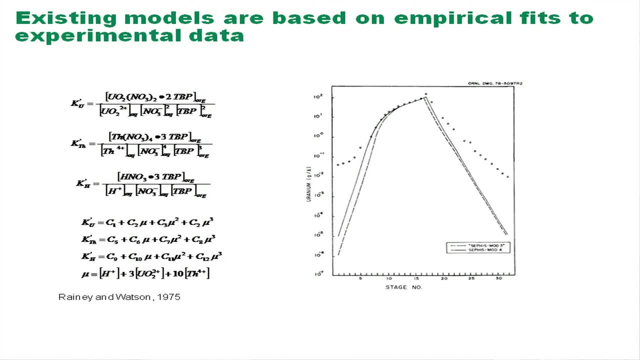 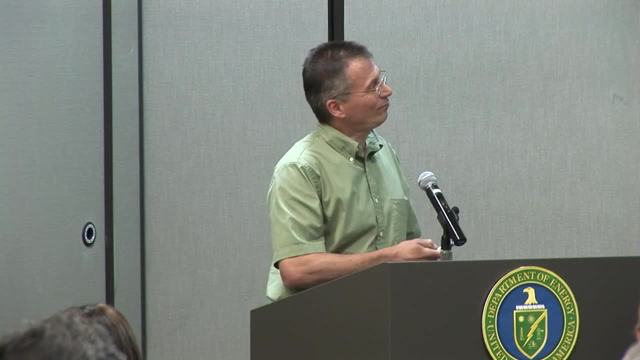 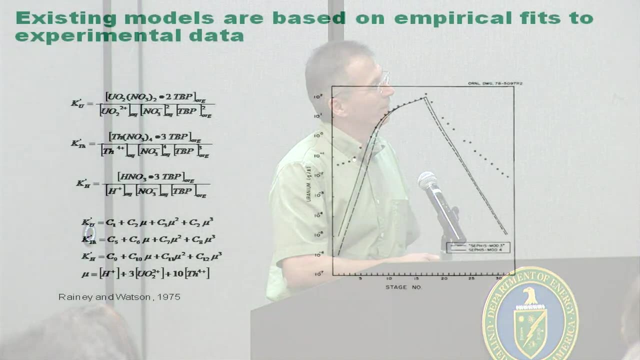 You can see that it's related to the concentrations of these species in those phases. But then, if you look these, these constants then actually are are functions that are complicated, functions that then depend on this Mu, which this Mu then is a is a function of the concentrations of species in solutions. 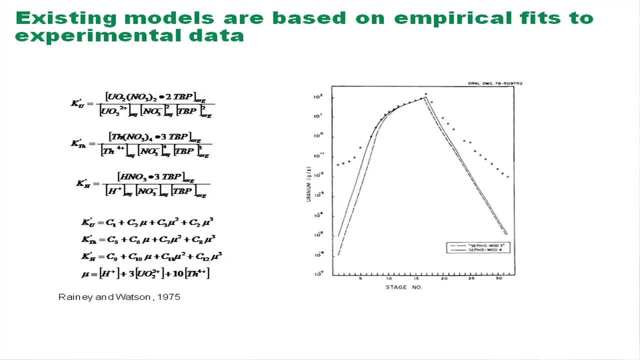 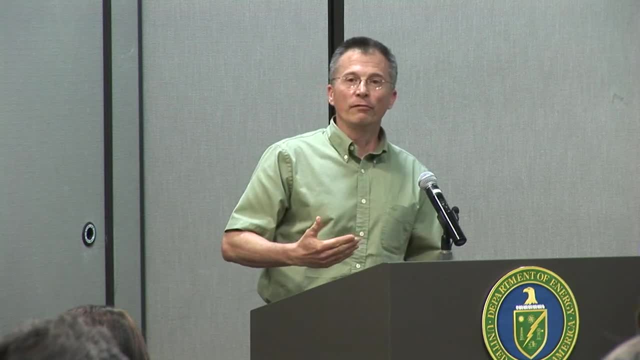 So, basically, this is a way to try to take into account the non-ideality of the system. Okay, so so this is an empirical fit which works pretty well. So, in just about every case, what you're going to find is: 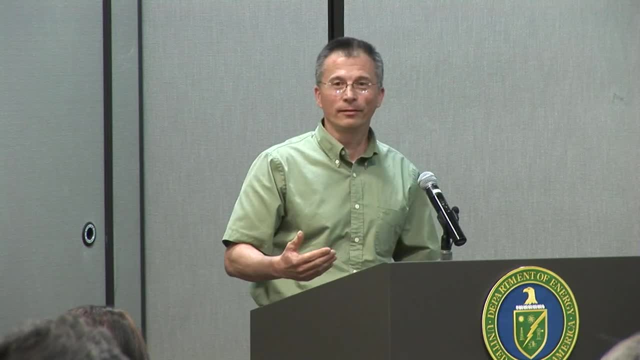 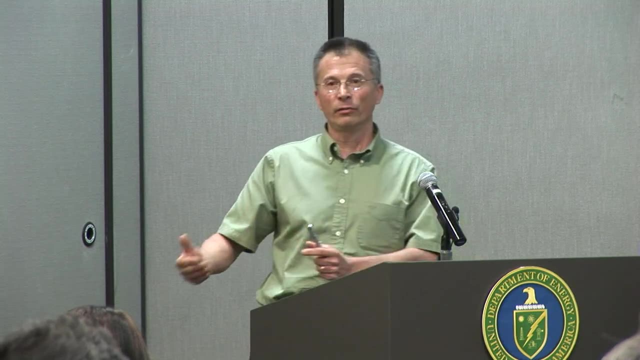 you have to take some sort to make some sort of fit. So if you go to a more complex thermodynamic approach, what you'll find is instead, now we're fitting a solubility parameter or something else, that's a more thermodynamic quantity. 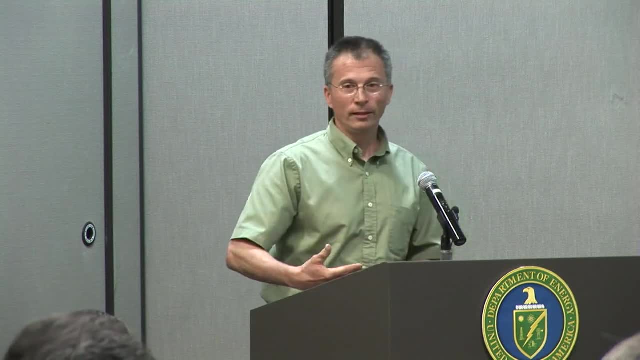 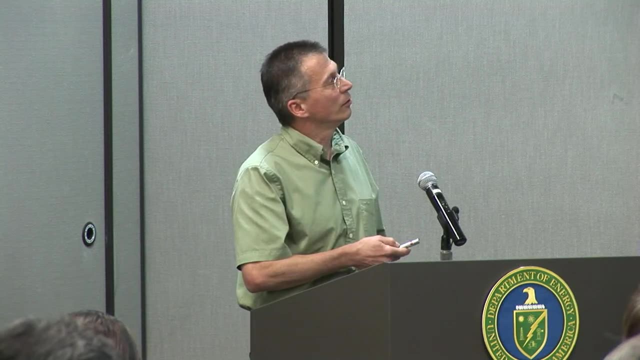 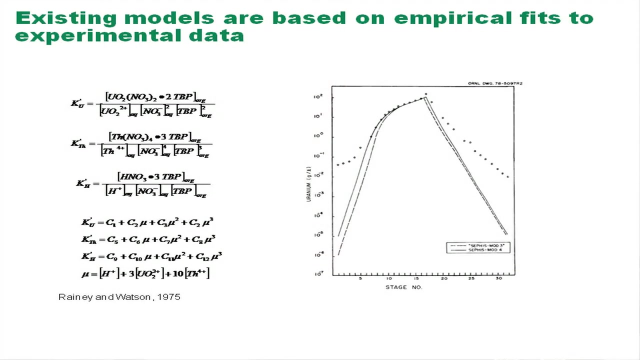 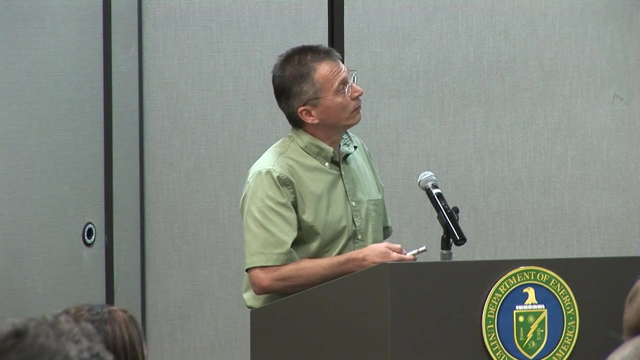 But still these aren't all fundamental quantities that you can look up. But looking back at these relationships, they do a pretty good job over the concentrations of concern for the target species. This is looking at the concentration of uranium across the stages of a solvent extraction bank. 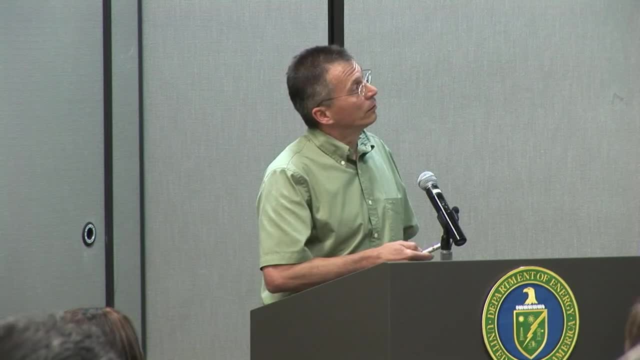 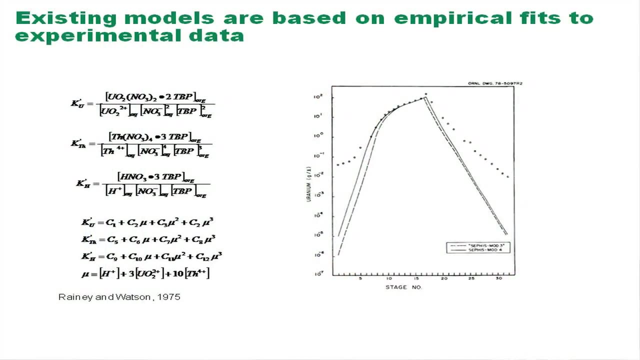 And you can see over several orders of magnitude. the experimental points match pretty well with the model And then you can see it deviates at the lower concentrations. And this could be for several things. It could be carryover of solvent, It could be analytical. 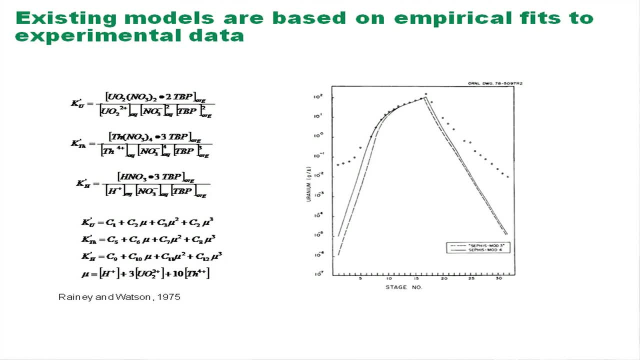 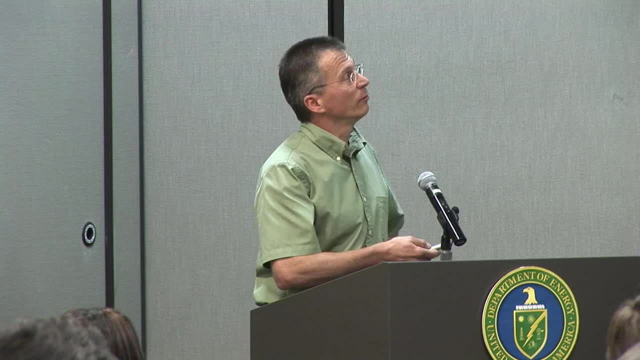 It could be analytical problems, But it also more likely is you've done these fits at the higher concentrations, where the species are in, concentrations where you're much more concerned about them. So if that's the case, then you're fit, not as likely to be as good when you're 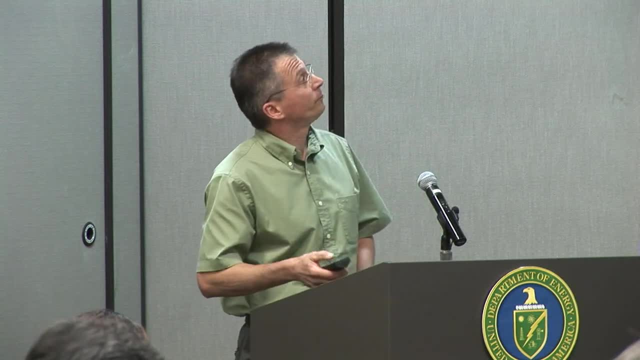 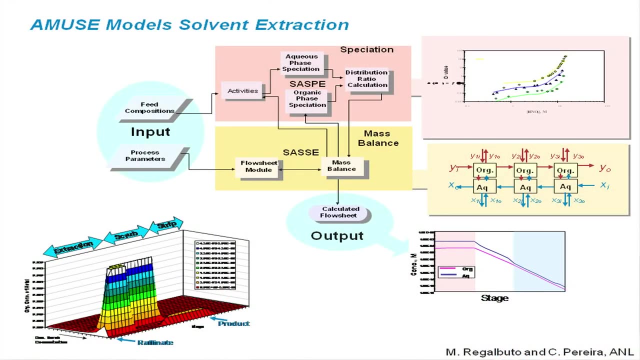 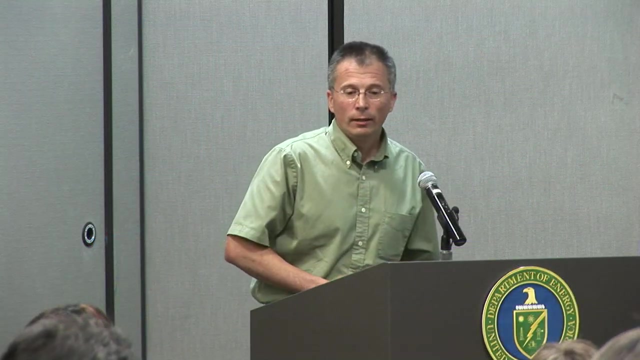 at the lower concentrations. OK, so, as we move forward in time, the generalized Truex model and then, following that, is the AMUSE model that we're going to talk about in a little bit, And the AMUSE model is a model that. 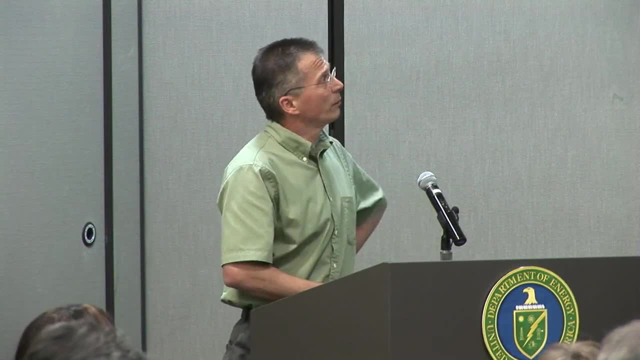 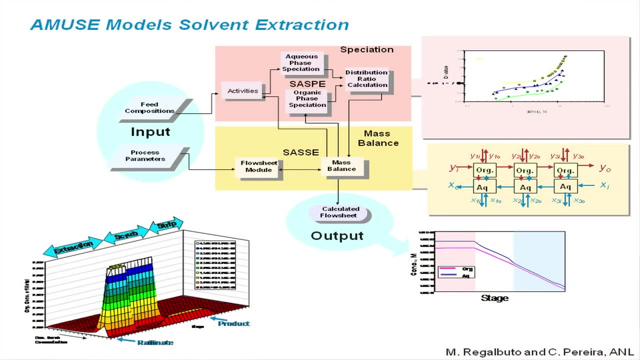 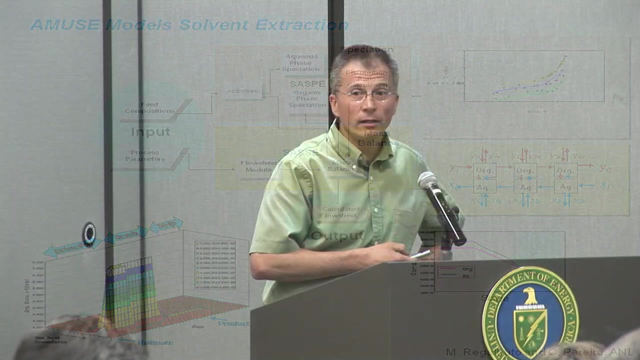 has been used to predict solvent extraction, And the AMUSE model is a model that has been used to predict solvent extraction, And the AMUSE model is a widely used equilibrium stage model, And so what it does is it combines thermodynamic relationships, So they do take into account some of the non-idealities. 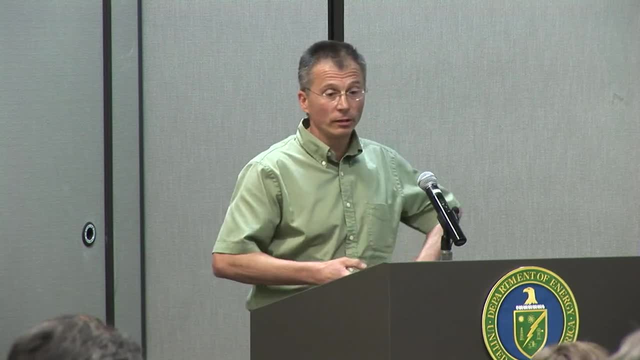 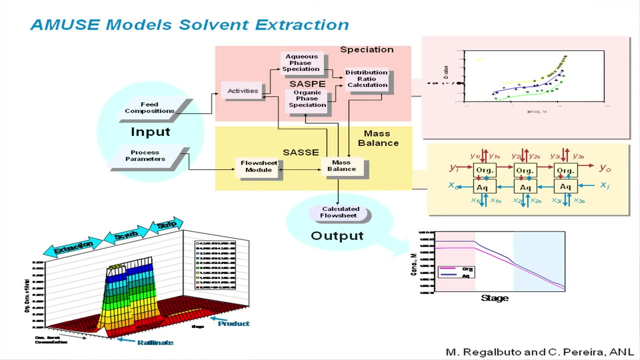 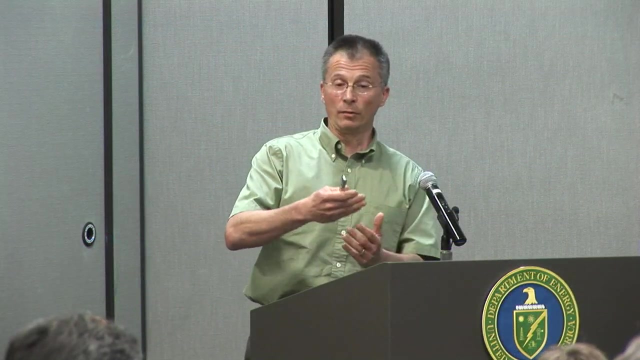 in the aqueous phase to predict distribution of species. And then they do a lot of math on experimental data and then combining that with a mass balance. So you do the mathematics of the phases- contact each other in these solvent extraction contactors, They reach some equilibrium. 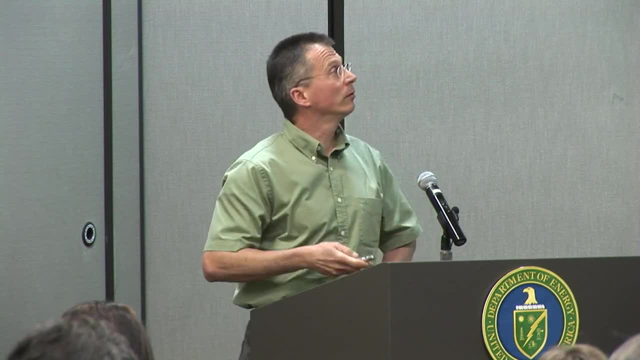 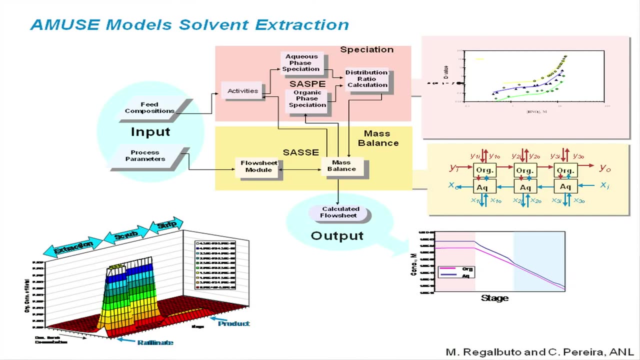 And then you pass those species to the next stage, And so it does the accounting for the mass balances, And so from that, if you do that accounting, then you can predict, and I'm losing my pointer here. you can predict, But if you do that then you can predict. 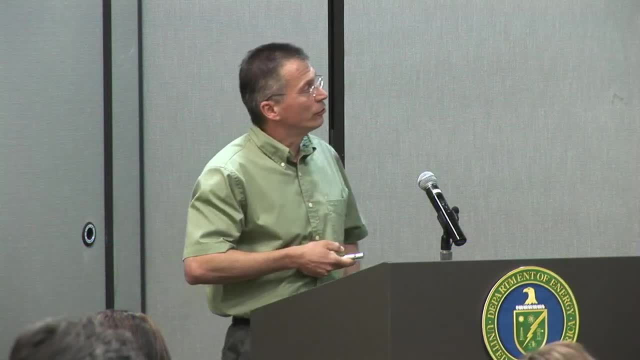 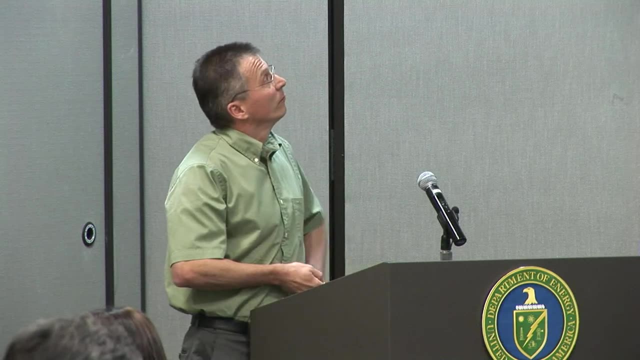 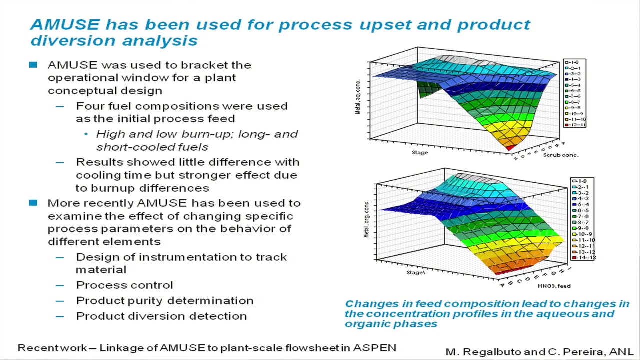 at what stages, what the concentrations of different species will be, And so this allows you to explore a number of different scenarios, basically, And so here's some examples Argonne has used to look at the design of a solvent extraction process And basically what they were able to do. 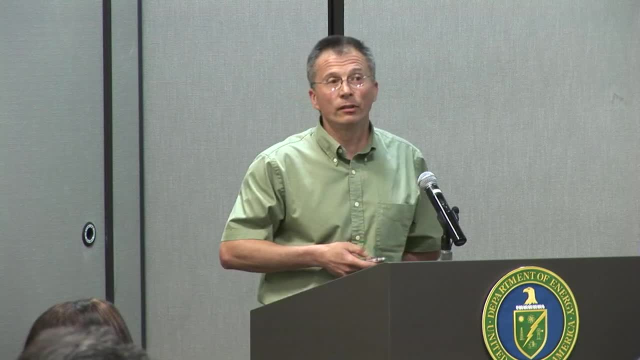 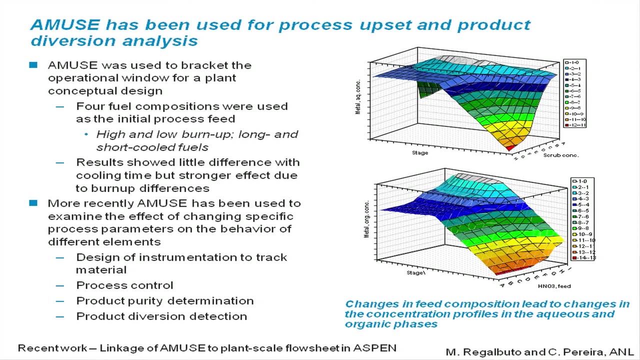 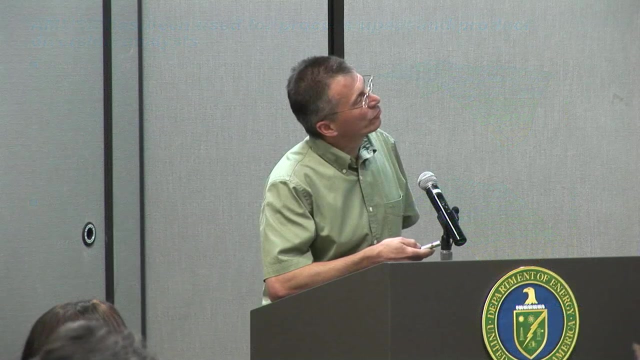 is look at a wide variety of basically operating parameters and not giving details on this. basically, But under a wide variety of conditions. what they can look at is the concentrations. Here's a metal concentration in the organic, for instance. You can look at one species in either organic or aqueous phase. 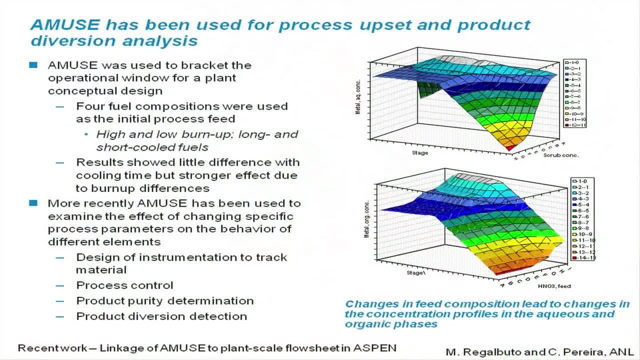 as you go throughout the system and then changing the parameters. So you use this model to look over a broad range of scenarios And they told me how long it took to do these, to do these simulations. It was quite a while because you have thousands of points here. 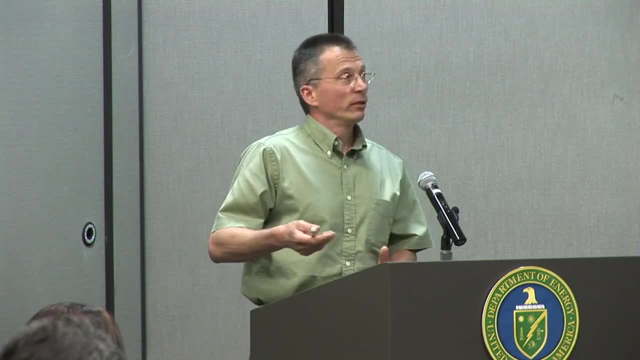 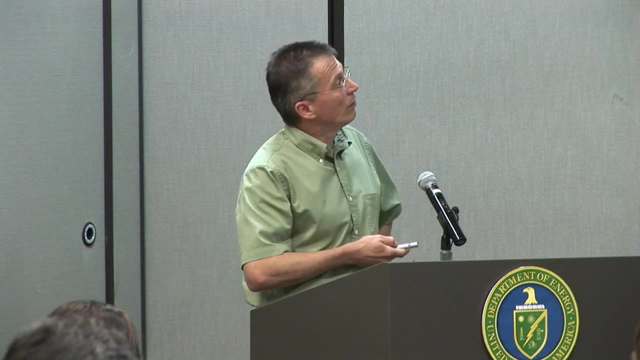 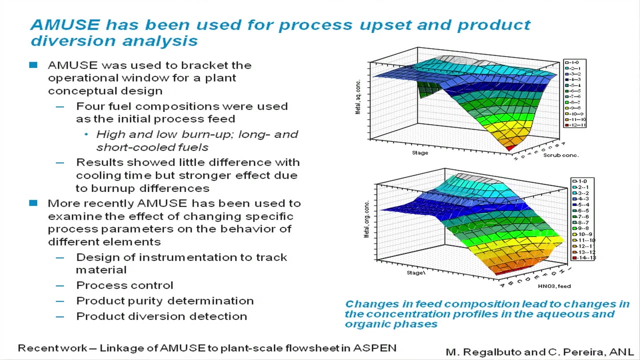 But basically, it would take you a whole lot longer to do the experiments, And so what this allows you to do is at least go explore the sets of conditions and see where you might be in conditions that you don't want to be. It allows you to design instrumentation. 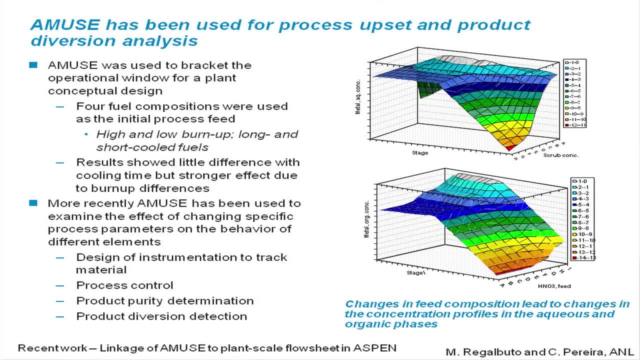 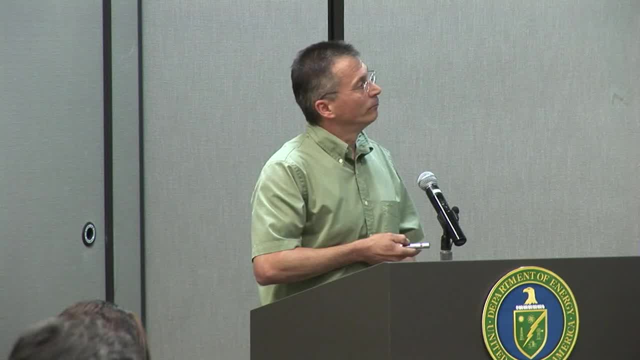 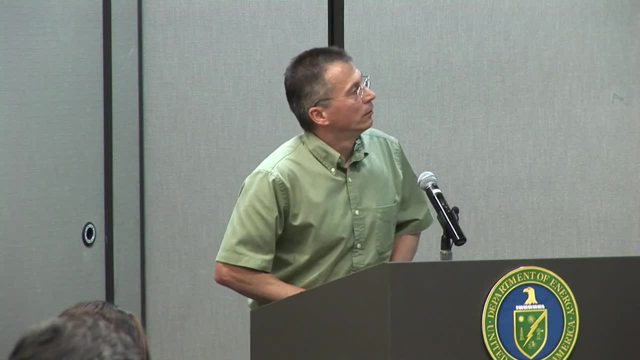 You can use this to go predict. well, the concentration is going to be in this order here. so we need this type of instrumentation. It could allow you to design a process control system And then it can feed into diversion detection type of analyses. 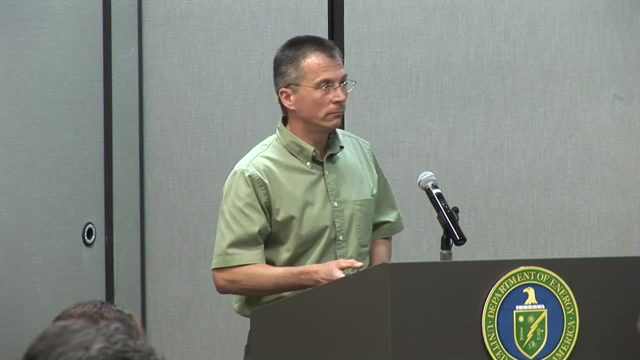 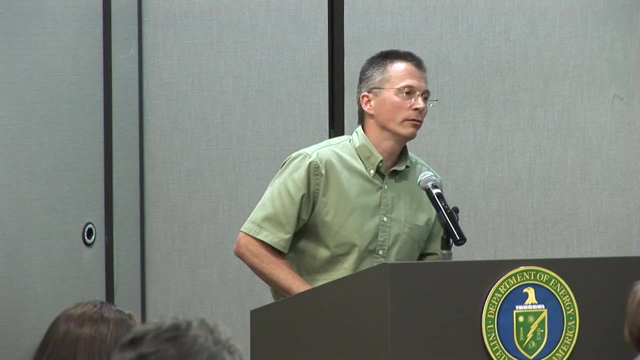 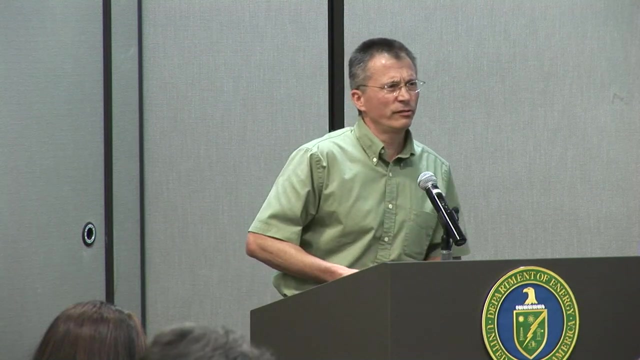 Is that similar to the acid-solid extraction That particular one? well, Amuse has several modules. I mean there's a Purex module, a Truex module, So there's several modules. Yeah, yeah, So there's probably six or seven different solvent extraction. 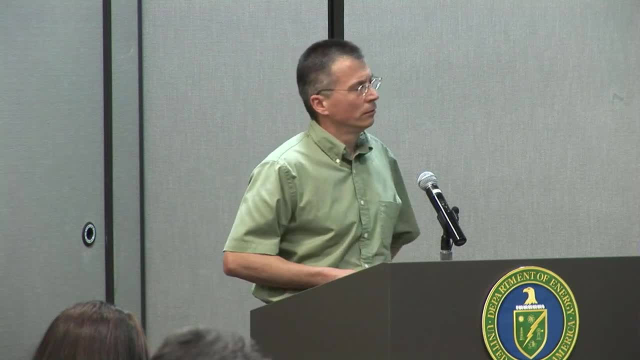 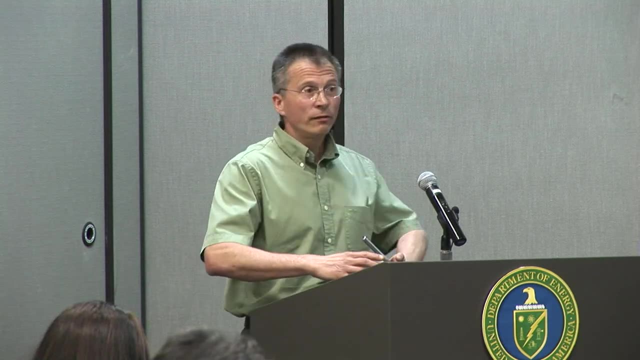 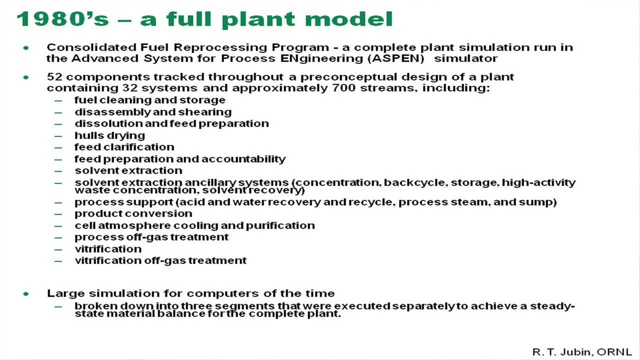 systems that they have. Okay, So now that was just the solvent extraction step. And now, if you're going to step up and do an entire plant, back in the 80s Bob Jubin and a team of his colleagues had done a complete plant simulation using Aspen. 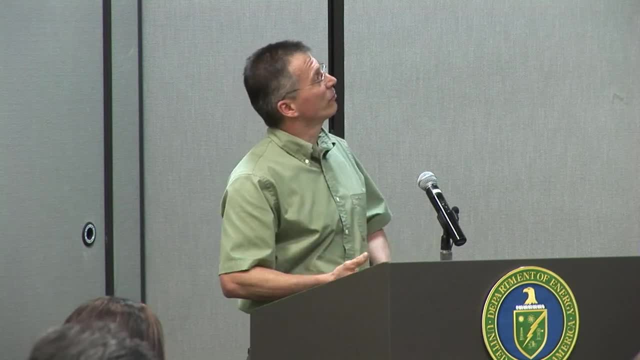 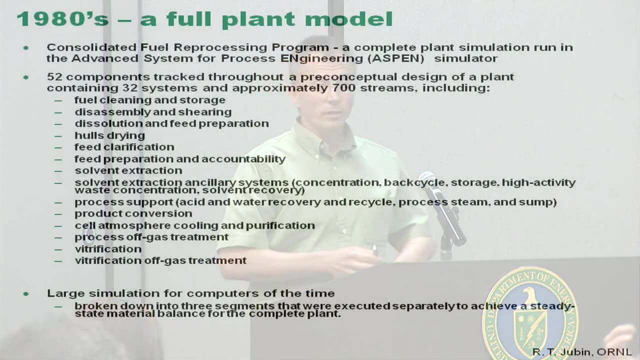 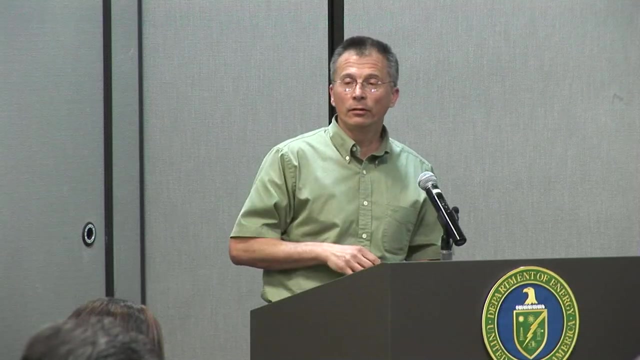 And this was, you know, 700 streams, 32 different systems. You can read the different types of systems that were put into this. So there were descriptions, simplified by necessity, but all the systems in an AQUIS recycling plant steady-state simulation. 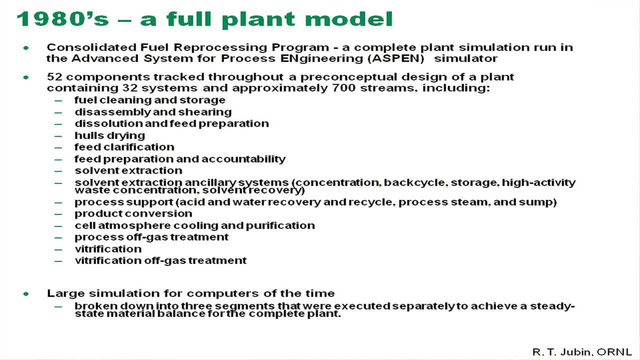 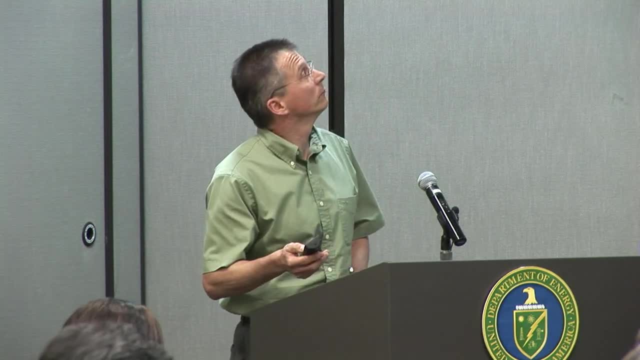 But this was a very large simulation for the computers at the time. In fact, they had to break down the plant into several segments just to be able to run the system. But very useful for basically getting a conceptual design of a plant. Okay, now moving forward. what can we do now? 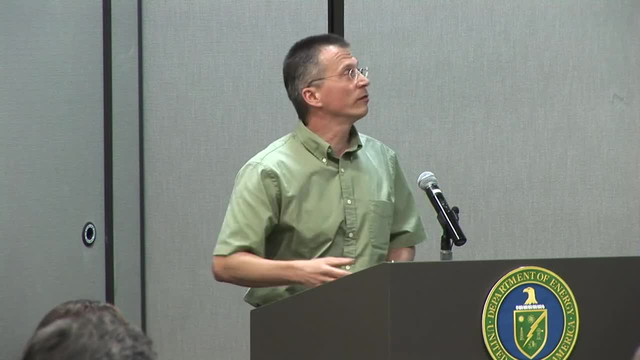 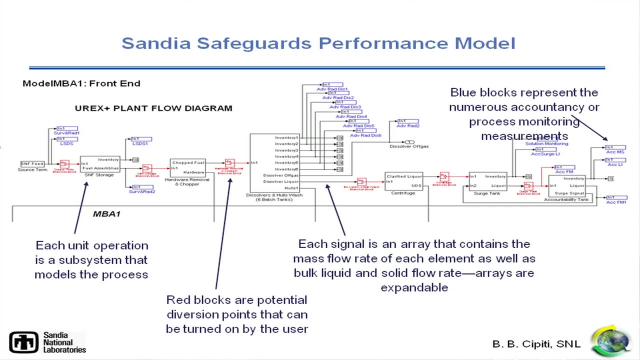 We should be able to do more than that these days with the way computations have gone forward, And I'll give you one idea of something that's currently being developed that looks very promising, And this is Sandia Safeguards Performance Model. Ben Cepedi is the main person on this. 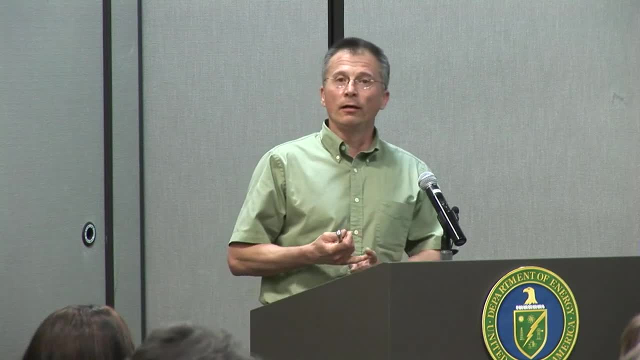 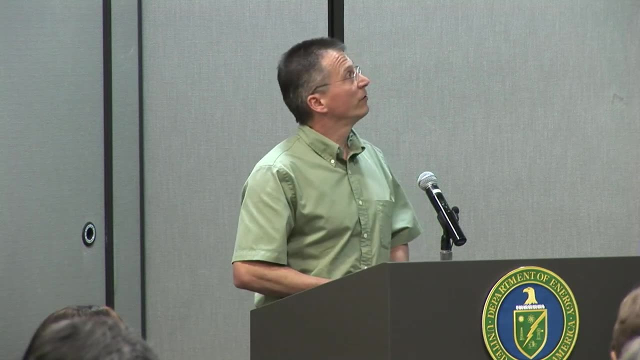 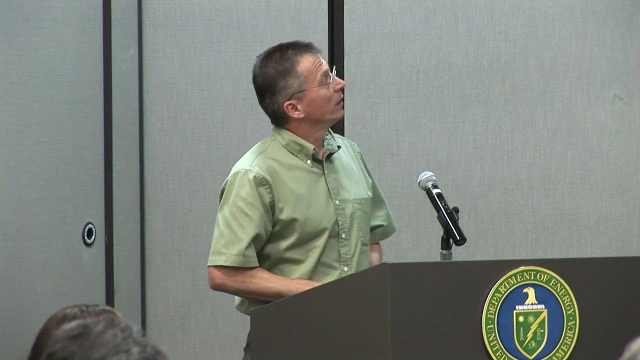 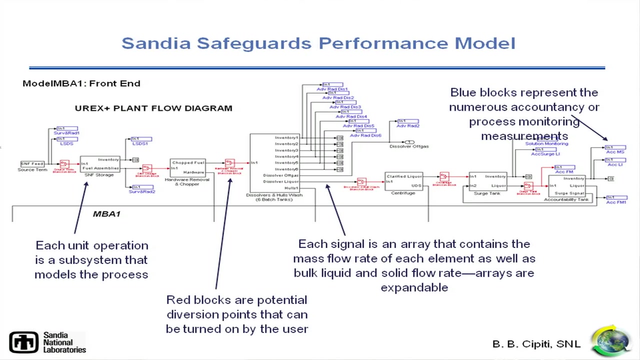 And what he's done is used MATLAB and Simulink to put together a model of a recycled plant and the instrumentation. Okay, so what it allows him to do is make the unit operations basically a box for each unit operation in a plant: Here's storage and then chopper dissolvers. 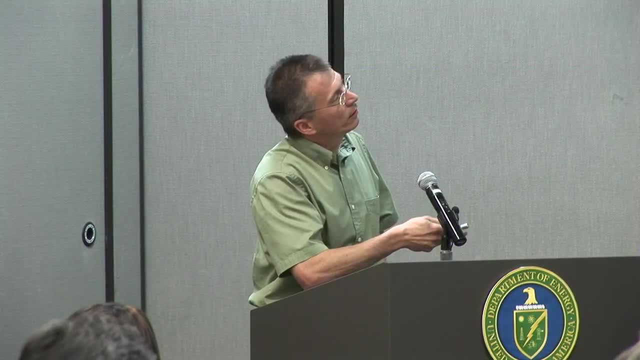 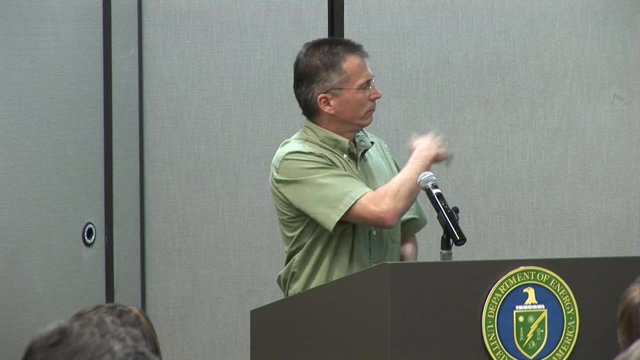 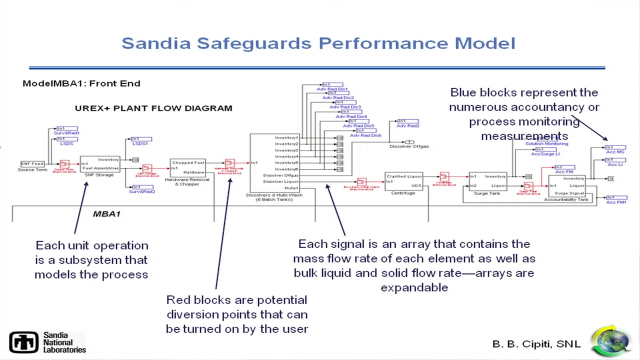 and hull washing, a centrifuge, a surge tank, accountability tank. Downstream here he has a solvent extraction system. He's Okay, All right, and so each of these is an operation. It gives some sort of description of the operations in the plant. 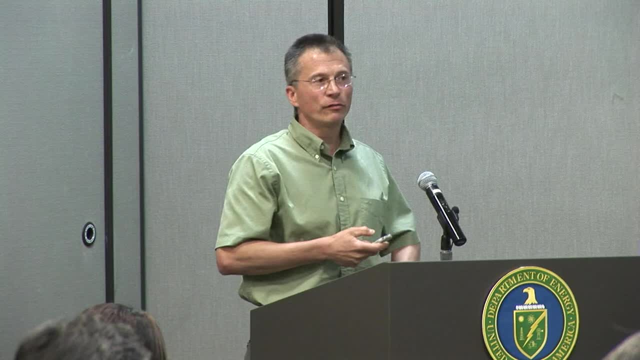 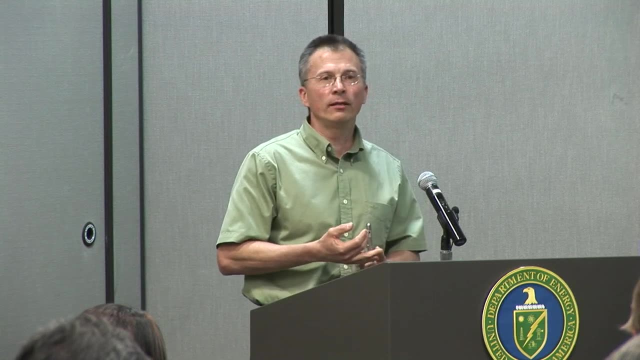 Now, albeit, these are very simplified And in fact, when you go to the solvent extraction portion of the plant, he's used just static splits from a muse and he's linked in a crude way to CFIS which allows a transient calculation. 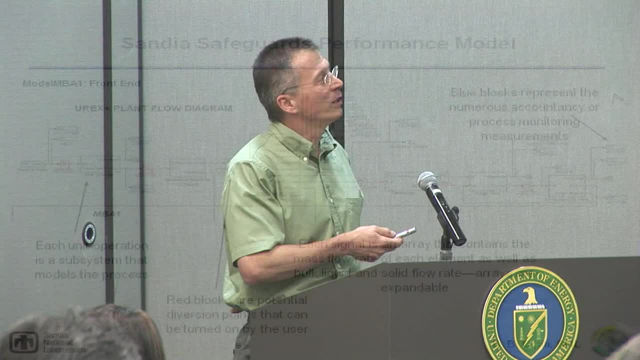 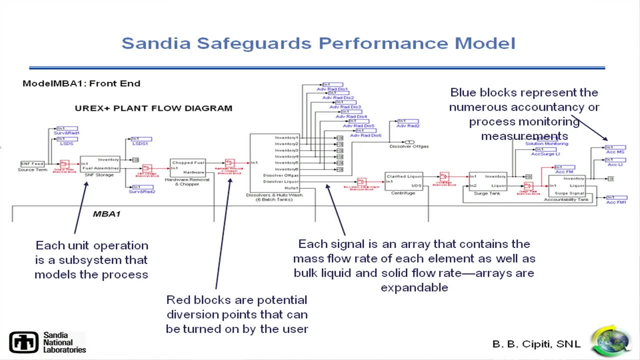 So a lot of work. A lot more work needs to go into this, to provide more rigorous description of the processes, But still, this is a great step forward because it allows you to then predict in a transient way. So you say, okay, let's go forward in time. 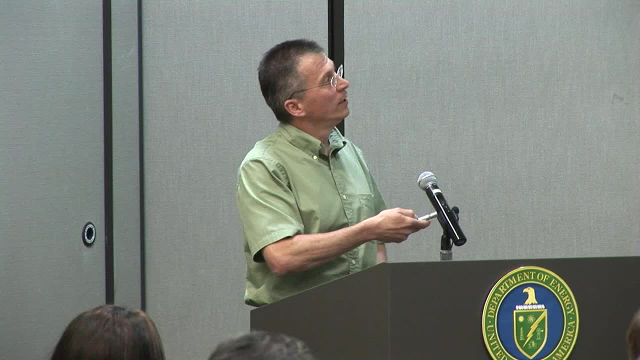 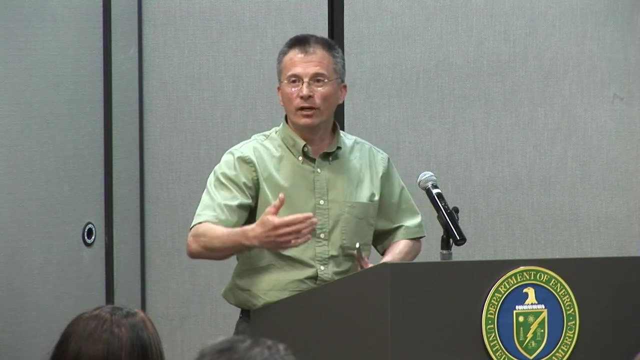 You can see what are the flows throughout this plant. You get the mass flow rate of each element and then the bulk liquid and solids flow rate, And you can set it forward in time and see what happens. Coupled onto that, then, are 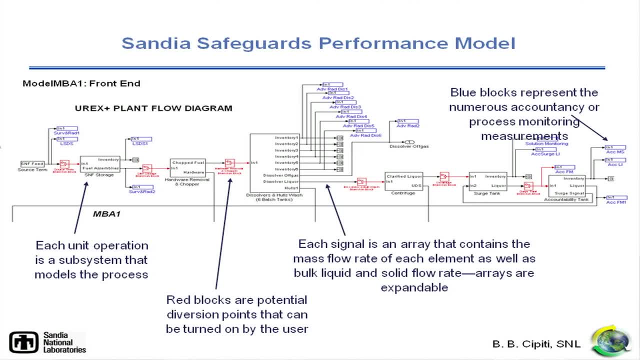 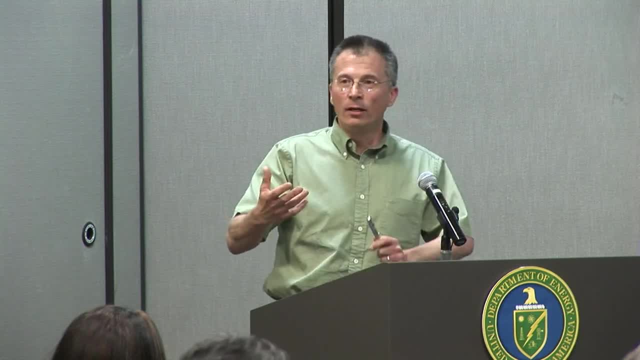 These red boxes are actual instrumentations that hooked up So he can say, okay, I'm going to put an instrument here and here's the characteristic of this instrument: It has, It's this accurate, It has this much noise on the signal typically. 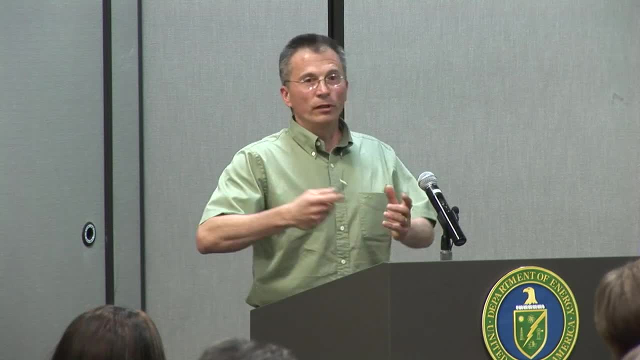 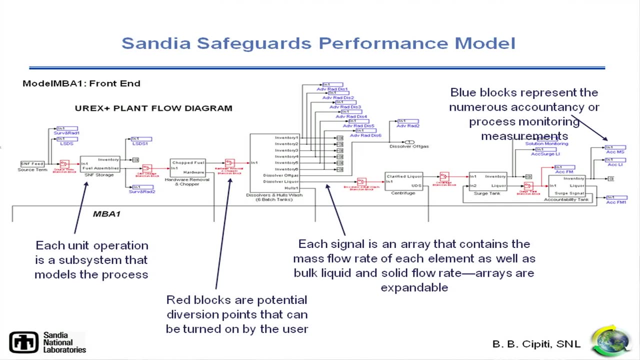 And then Can then set up different accountancy scenarios, let's say, Let's say what if I, What if I put this set of instruments around here, What will I see, And then allow the system to move forward in time. 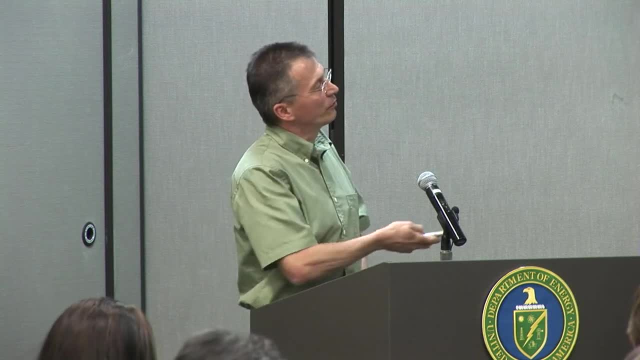 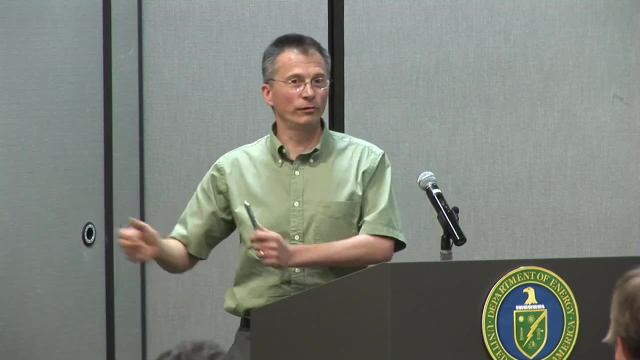 Okay, and Oh yeah, the red block, The blue blocks are the instruments, Red blocks are diversion points. He can tweak on and off. What would happen if somebody turned a valve here or changed this flow rate or did something else? 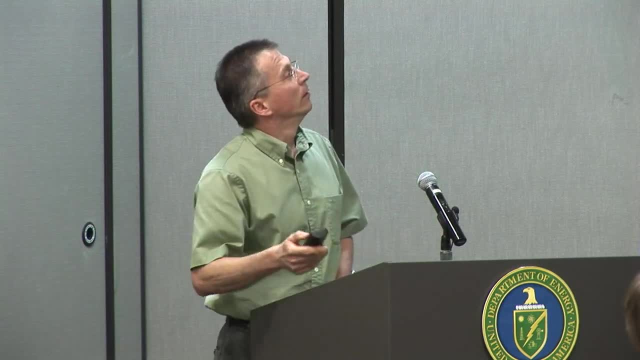 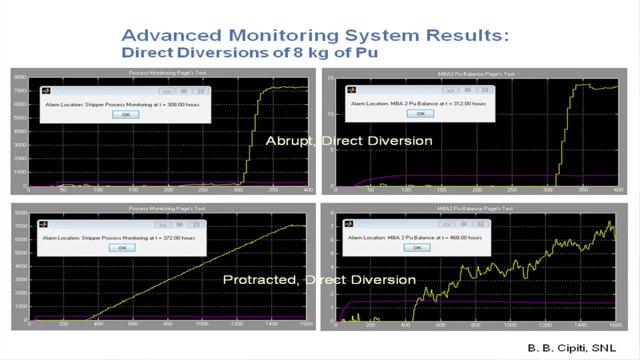 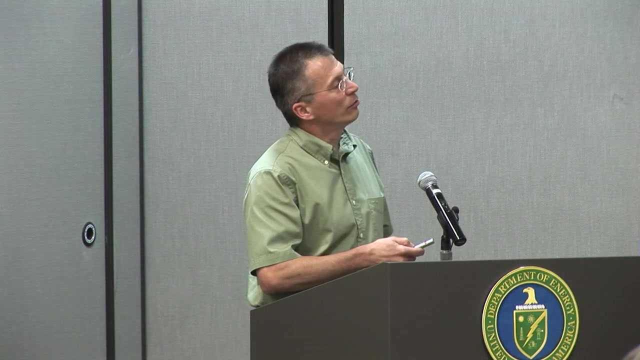 What would you see? Okay, And so then you can run through different scenarios, And then this just shows some examples of an abrupt direct diversion and a protracted direct diversion. And here is some measure of the inventory or the uncertainty in the inventory. 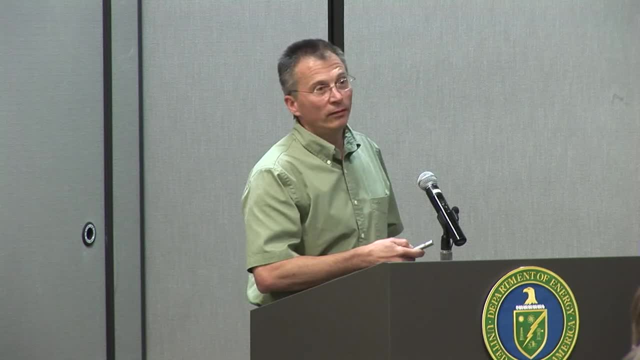 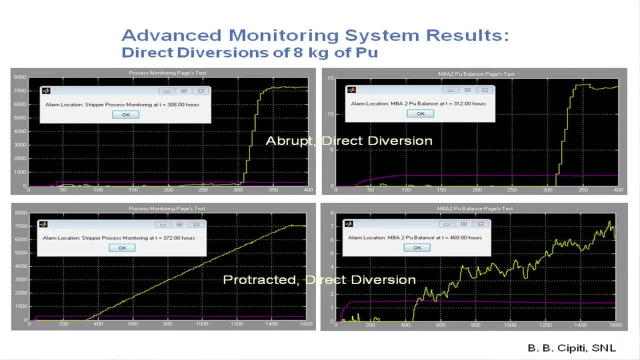 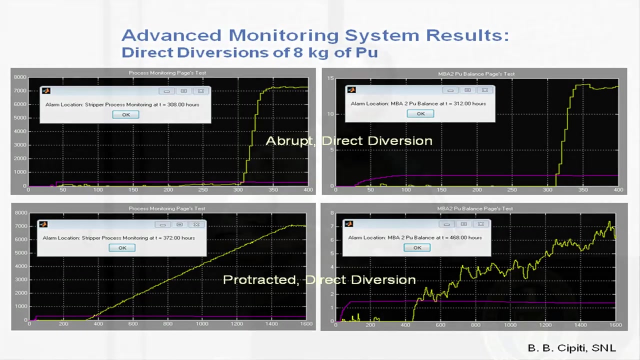 The purple is the expected result, and then the yellow is what is seen by the instrumentation, by using the instrumentation that he set up, And so he's shown in some of his simulations that, yeah, if you put instrumentation at certain parts of the point, 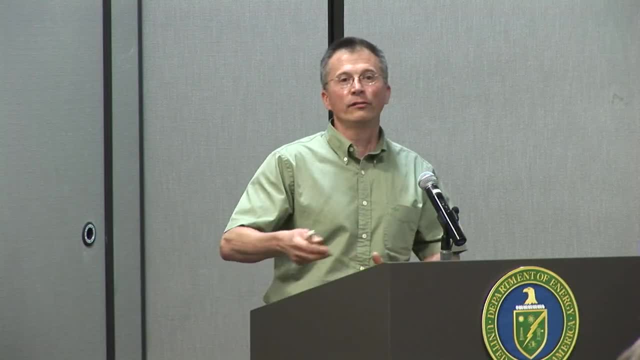 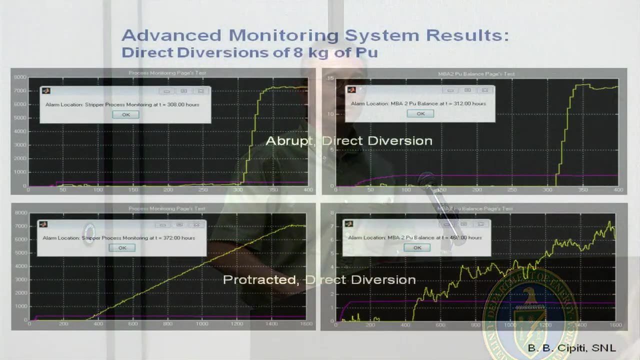 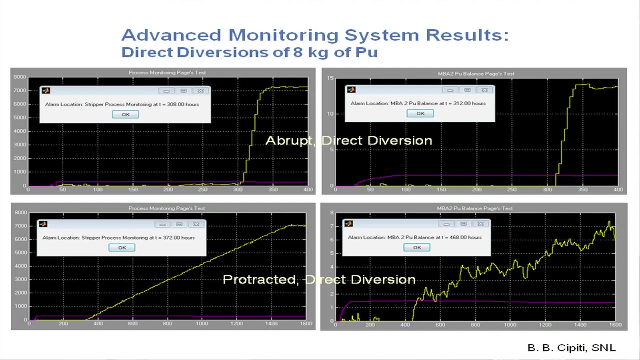 you can do kind of improve your real-time accountancy, or in principle you could do that. So this is a useful concept. It's limited somewhat by what you can do with MATLAB and Simulink and it's definitely currently limited by the amount of rigorousness. 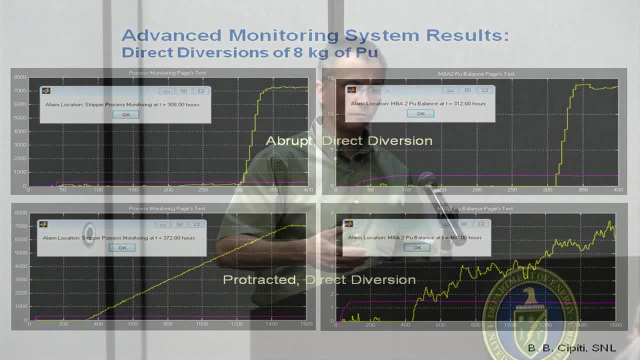 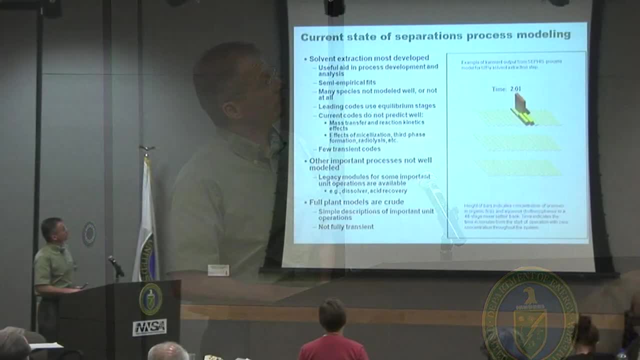 or sophistication in each of those unit operations models. So there's certainly a lot of work that needs to go on to make those models. So there's certainly a lot of work that needs to go on to make those models. Okay, so basically, where are we in process modeling? 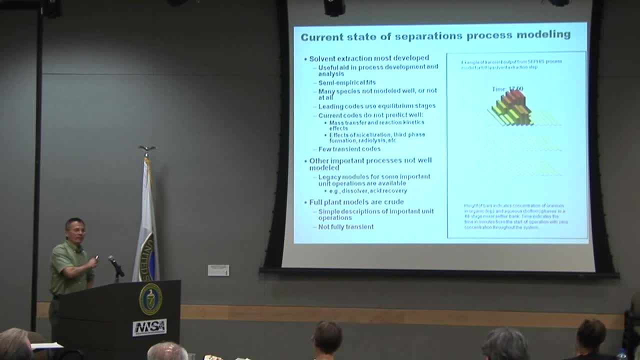 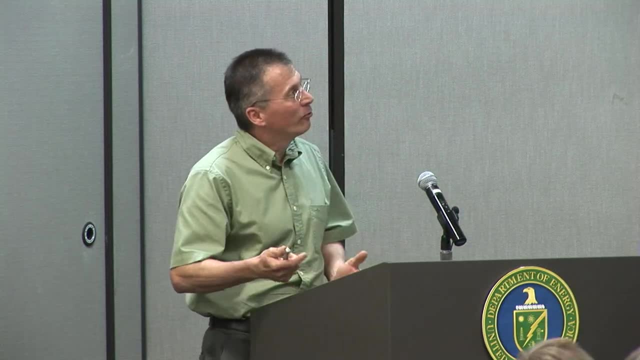 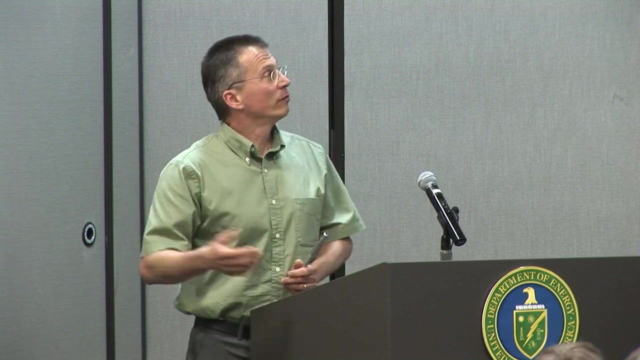 And I guess I caveat this- This is the state of process modeling for open programs, codes that are available. I'm not talking about industrial codes. I'm not talking about proprietary codes or codes that are used internationally that we can't get our hands on. basically, 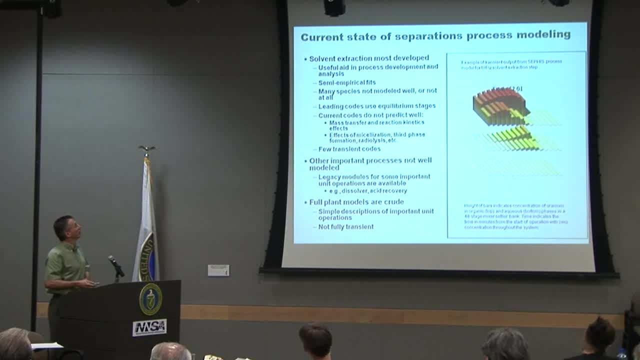 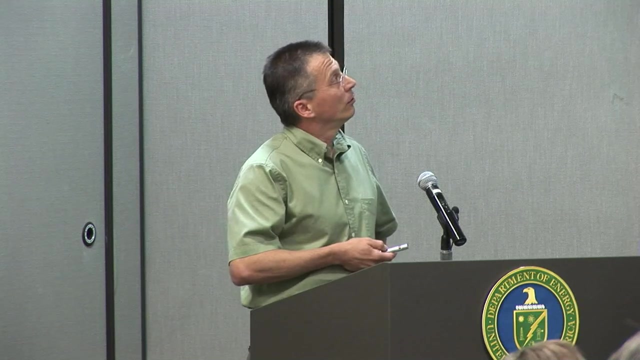 This is what people in this room could work with. Solvent extraction obviously is the most developed because most attention has gone there. It's been shown to be a useful aid in process development. Every solvent extraction code currently has some sort of empiricism in them. 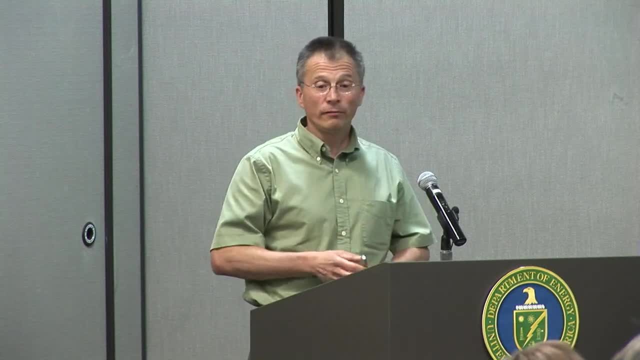 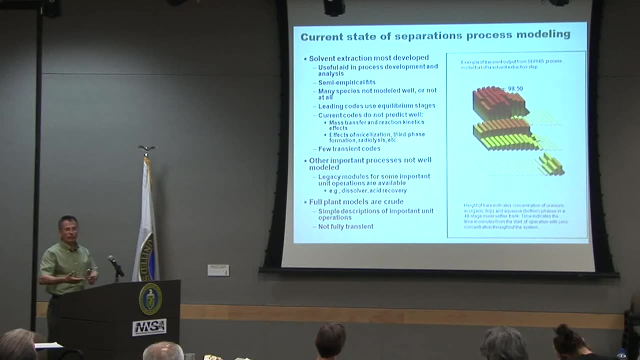 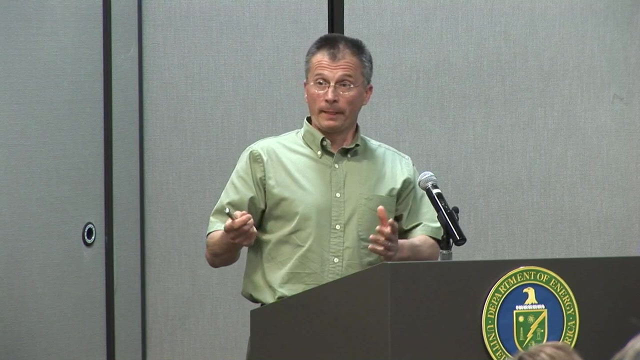 Many species are not modeled well or not at all. I mean, obviously, you'll see, the key components are modeled, but then trace species and some other species are modeled approximately or just not modeled at all. The leading codes use equilibrium stages and this is a good approximation in most systems. 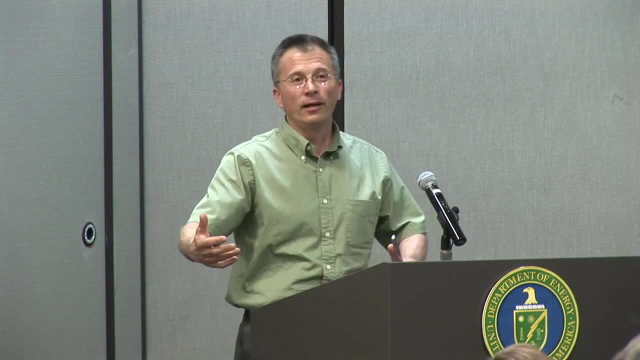 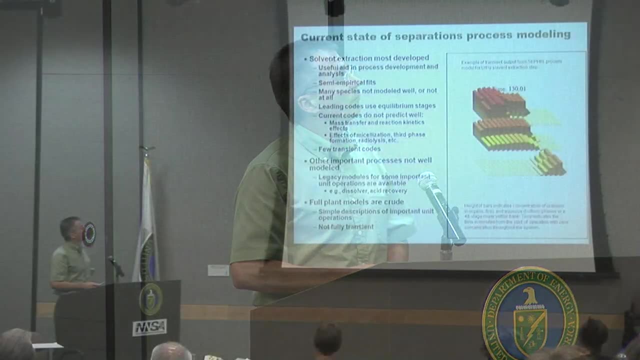 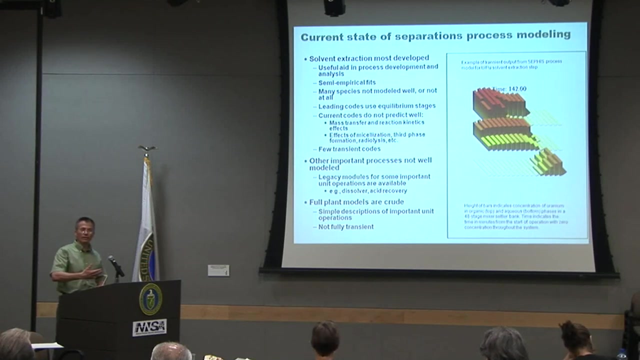 If you're talking a mixer settler with long times, so the kinetics don't come into play and the hydrodynamics are not so much of a concern. that's probably a good approximation. But as we move towards centrifugal contact, centrifugal contactors with short residence times- 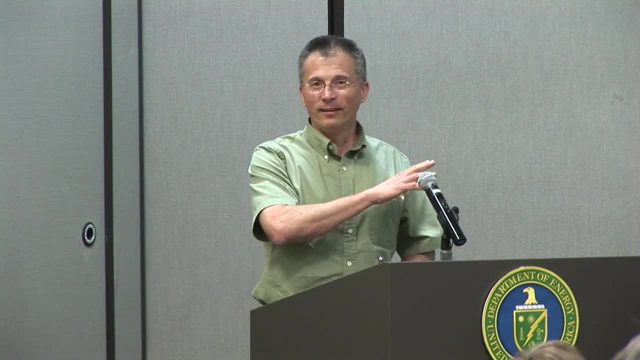 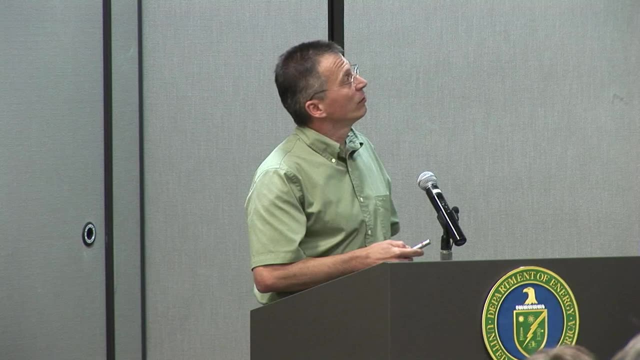 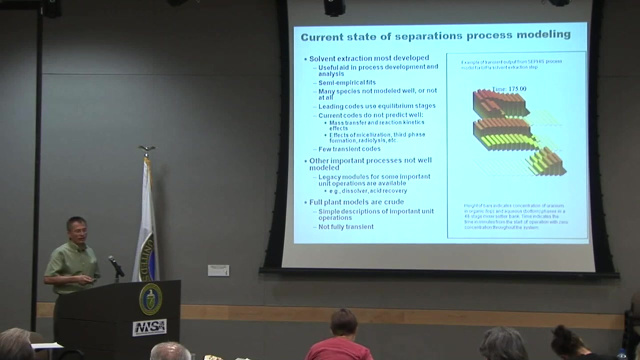 and more complex hydrodynamics that may or may not be accurate enough for some systems. Current codes do not predict well mass transfer, reaction kinetics effects, the effects of mycelization, third phase formation, radiolysis is taken into account in a few ways in an approximate way. 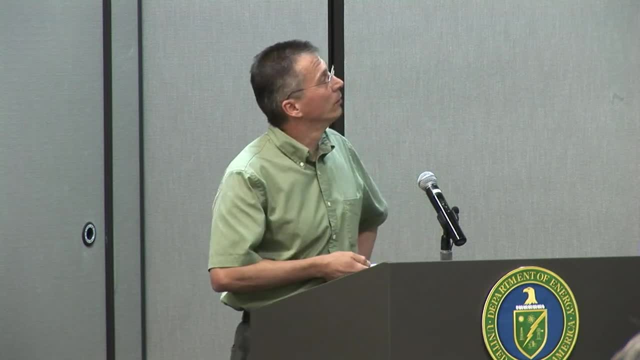 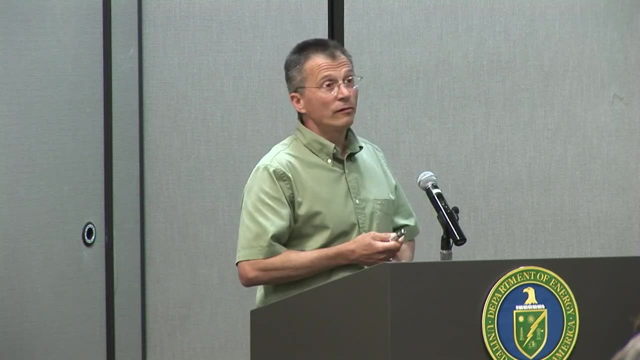 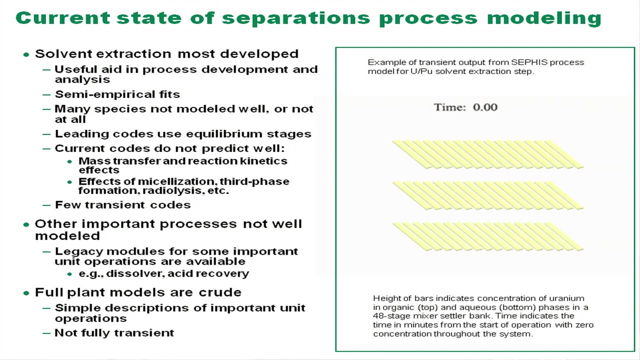 But there's not a fully rigorous way to deal with that And there are a few transient codes available. Other important processes are not well modeled. There's a few legacy codes available from work in the 80s, For instance dissolver and acid recovery from off-gas. 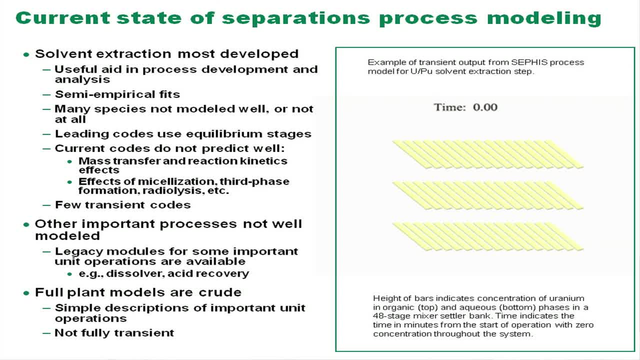 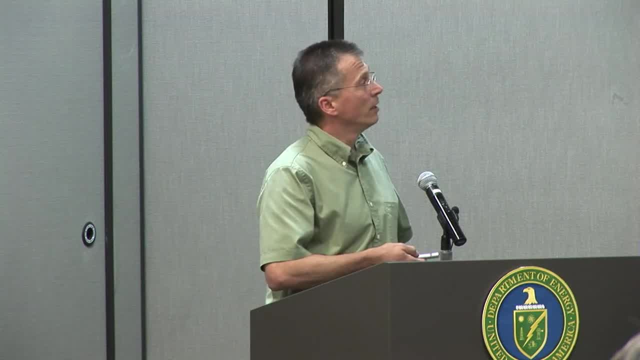 Those are. there are some codes available and actually we're making use of them now and trying to turn them into hook them up with our current plant level code models And for the most part the plant level full plant models are crude. 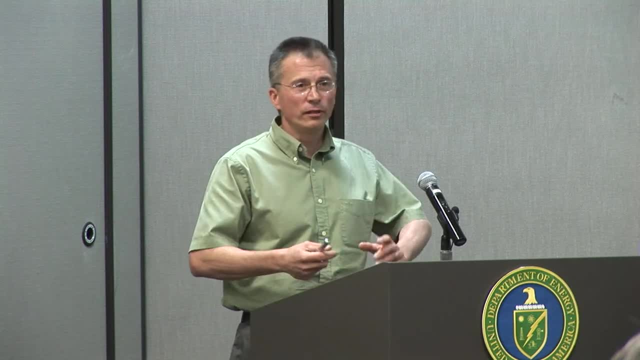 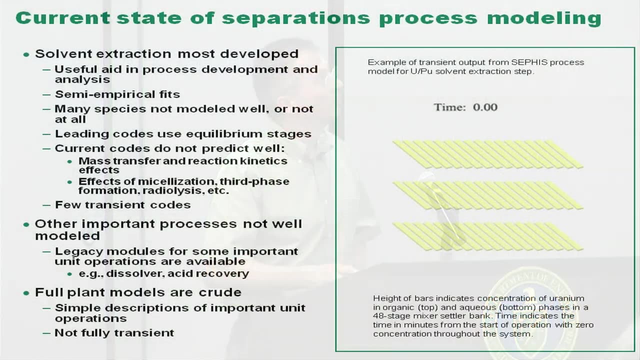 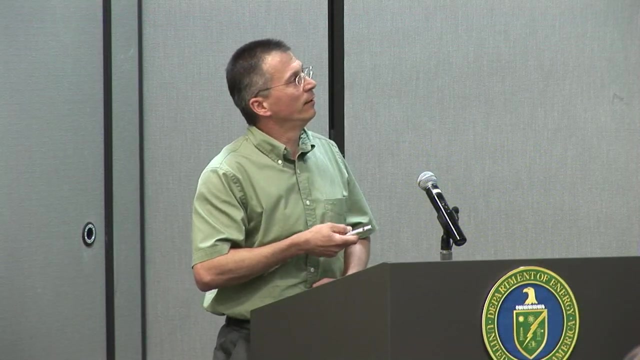 There's, they're not fully transient and the descriptions of each unit operation is simplified. And this animation that's been going on over on the right side, that's basically just a visualization of the what CFIS process model will do, showing concentration. 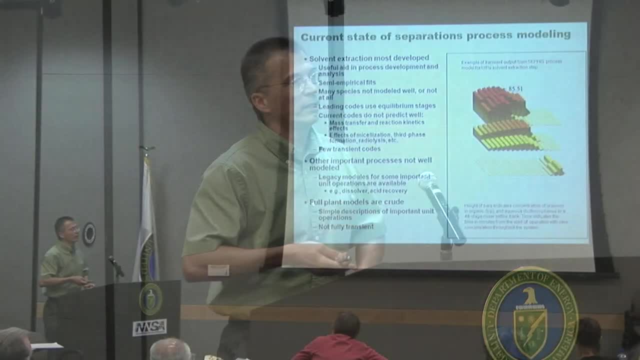 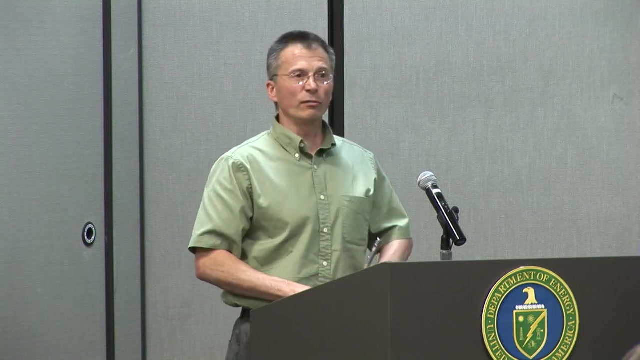 both the aqueous and organic phase of uranium, starting up from no concentration in the entire solvent extraction banks and just filling up with feed. So it's showing the types of data that you would like to be able to have. So if there was a process upset, 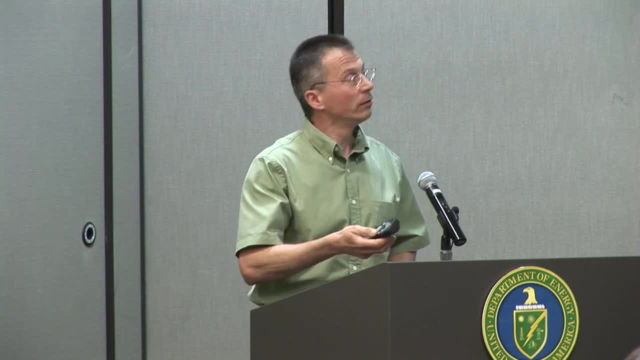 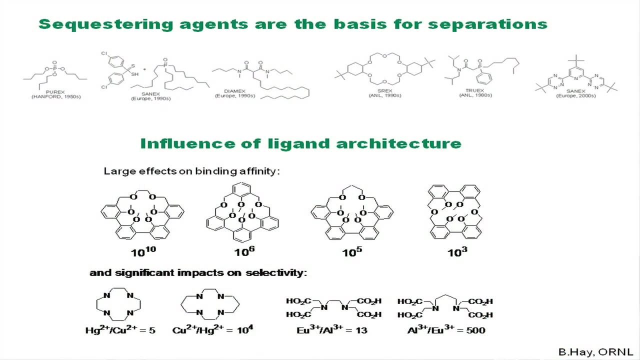 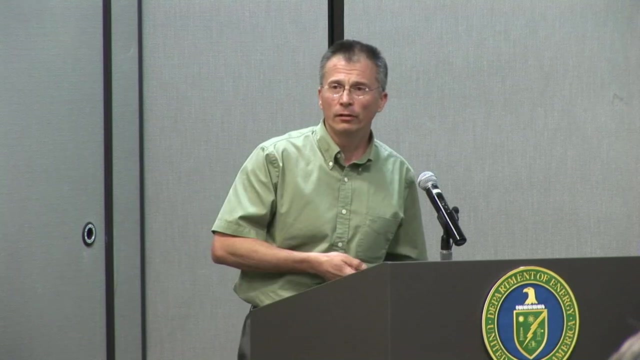 how does that propagate through the system? Can you predict that and see it? Okay? moving forward from the plant level, unit operation level, down to molecular modeling, How's molecular modeling going to be useful? Well, one place it has been useful is in guiding the design of solvent extraction separating agents. 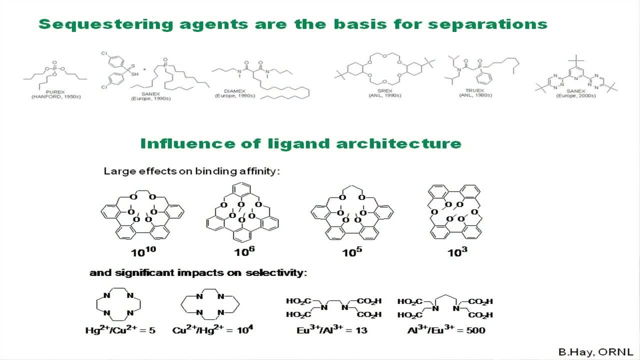 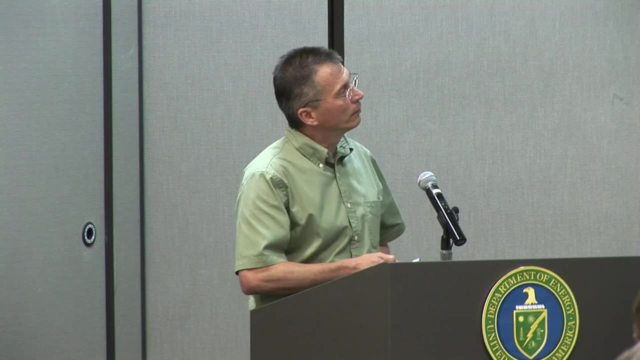 Here's a number of the separating agents that are used in different processes. What you find is the structure of these molecules have a huge effect on how well they perform. You look at these very similar looking compounds and they have the same very similar looking structure there. 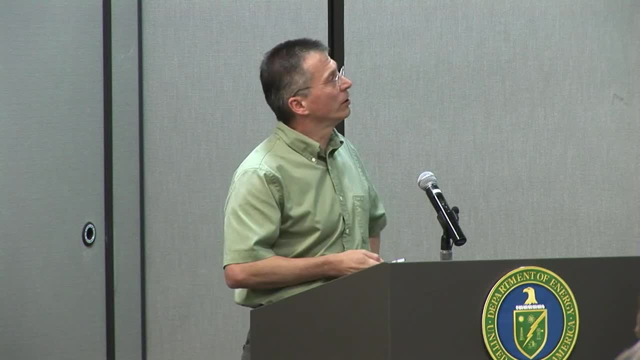 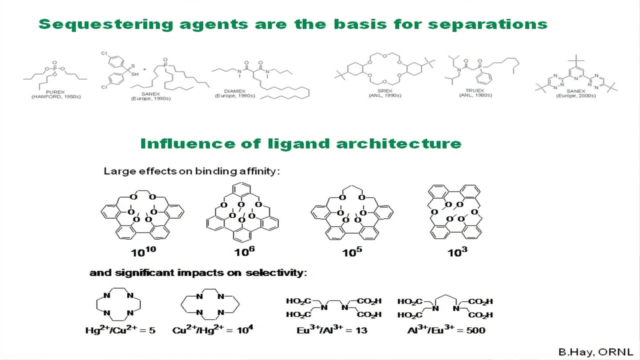 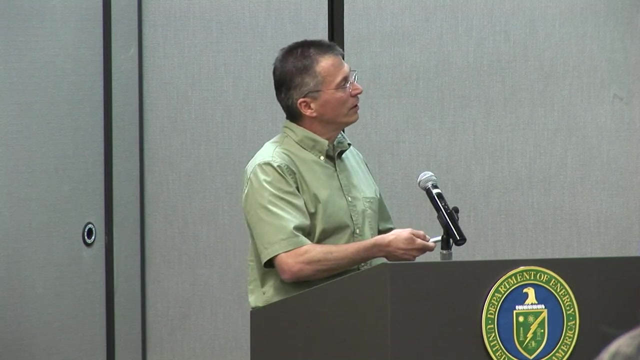 but just minor changes in the architecture have a huge effect. Here's binding affinity. You can see it varies over seven orders of magnitude in this example. Go down to the bottom here and also see impacts on selectivity. You can see here very similar compounds. 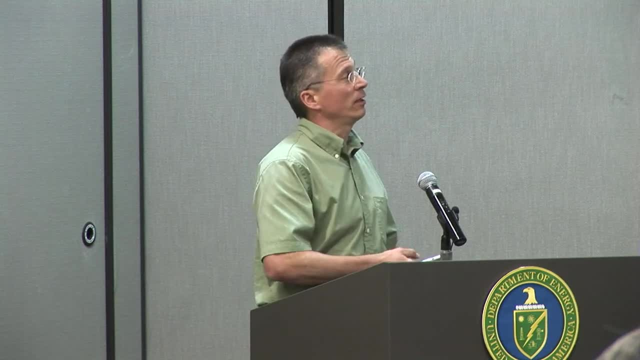 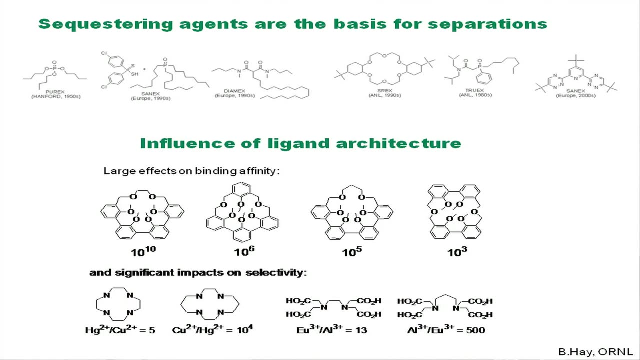 but they change four orders of magnitude and actually change the relative affinity between mercury and copper just by a slight change in the structure. And again over here with europium and aluminum: Again just minor changes in the structure. Here the only thing that's changing. 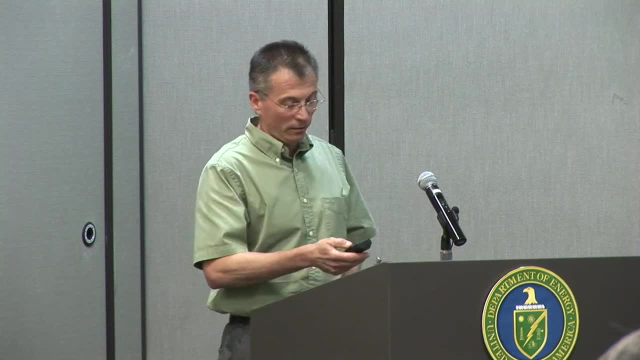 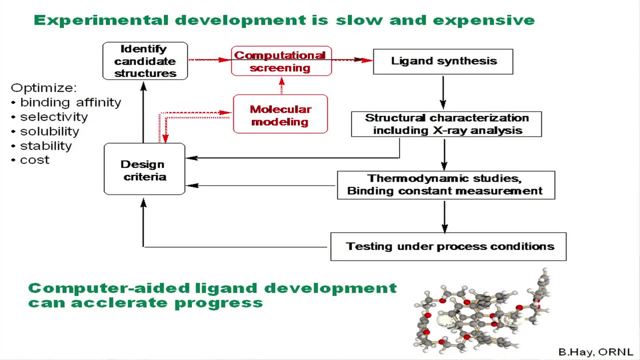 is the length of this linkage between these two nitrogens Okay. so if we could understand that, then maybe we can design molecules more quickly. So before people like Ben Hay started doing this computer-aided ligand development, what you had to do was: 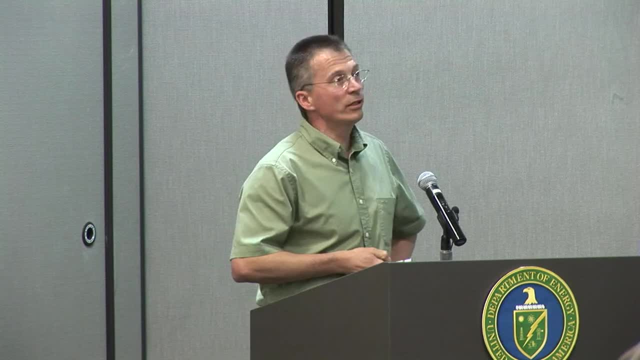 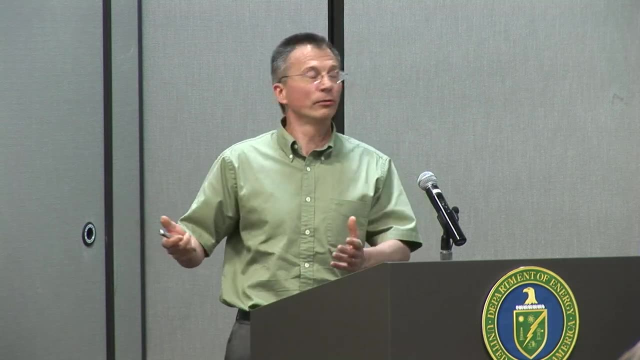 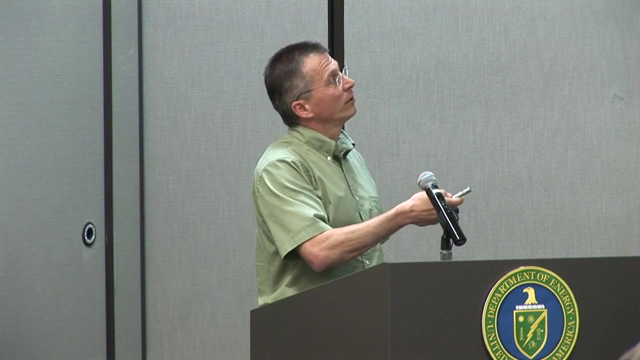 just through the intuition of smart chemists, they come up with some candidate structures, And this is not in any way to downgrade smart chemists. They do a great job. However, you're going to identify hundreds of candidate structures and that's all right. 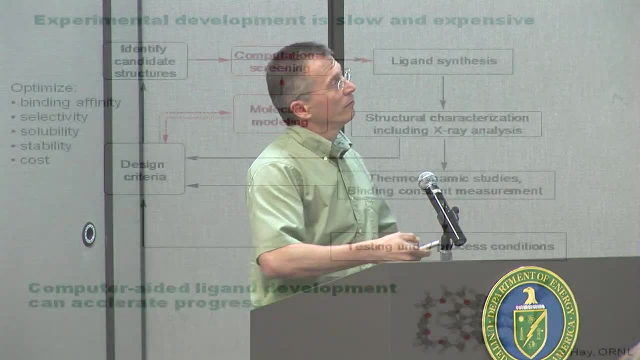 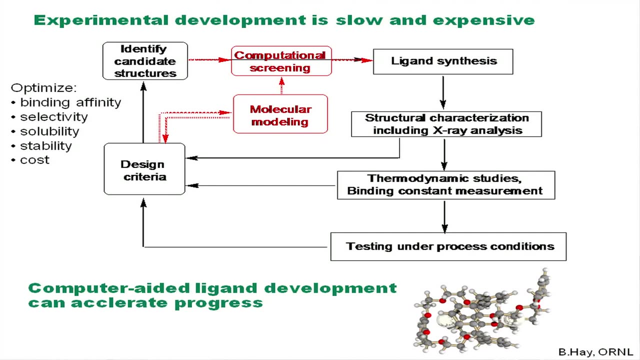 but then you have to synthesize them and characterize them, and then you have to do a bunch of studies, and all this takes time and effort, Okay. so is there a way to accelerate this? And so the idea is: can you do some computational screening here? 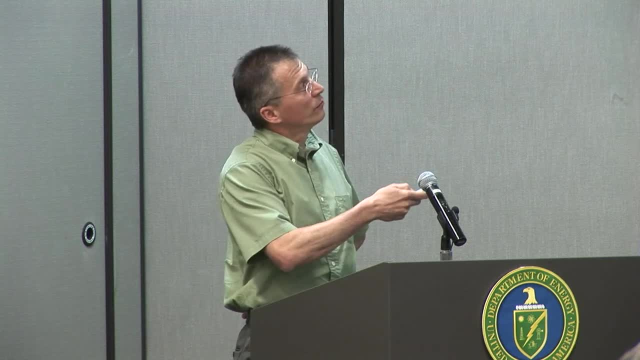 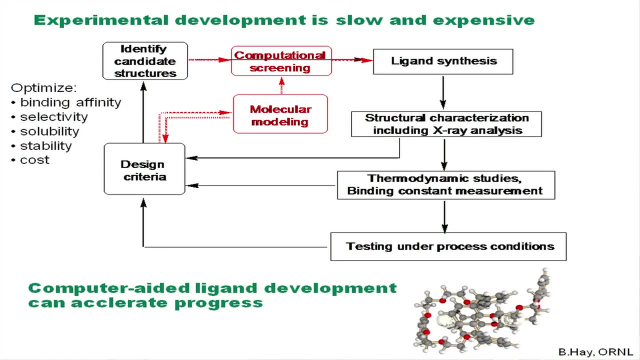 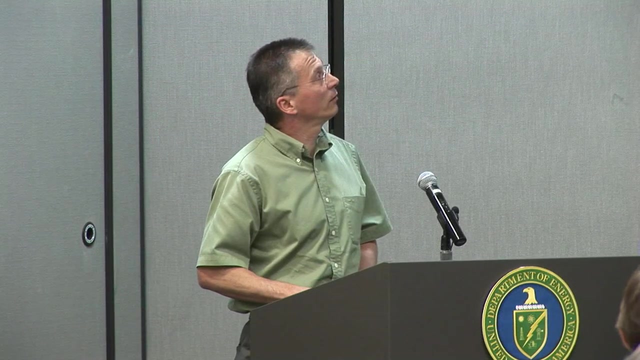 to cut down the number of candidate structures and then actually use some molecular modeling to help you even more accelerate that. Okay, so you can optimize on binding affinity, selectivity, solubility, stability, cost and, primarily, what's been done to date. 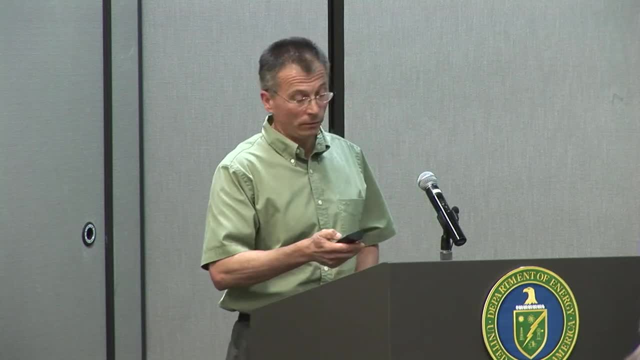 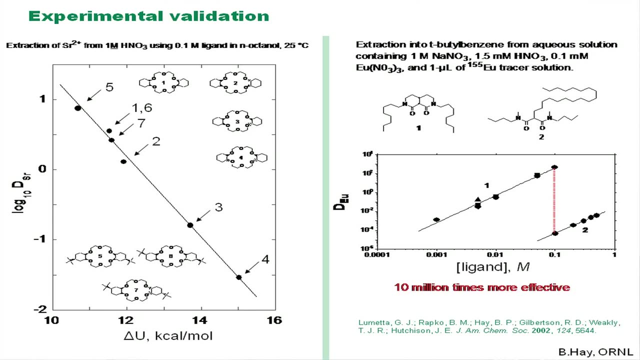 is optimize on binding affinity and selectivity, And here's some examples. You know Lumetta et al at PNL proved this. Okay. so what you're looking at here is on the x-axis, you're seeing the actual free energy change. 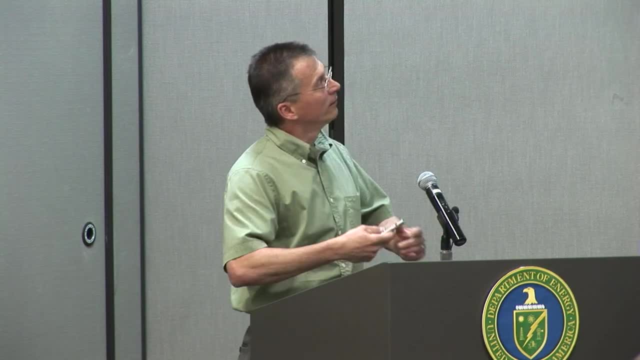 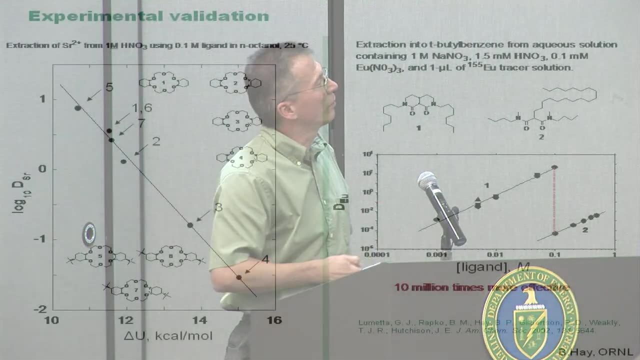 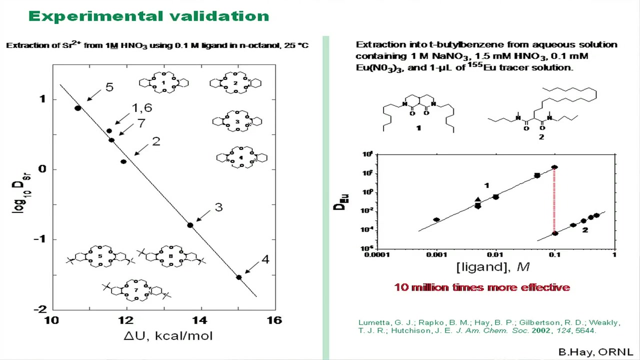 when you occupy the bind, the target metal, in this case the strontium. This is computational on the x-axis, The y-axis is experimental. Okay, and so you can see a very good relationship between: hey, if we have lower energy. 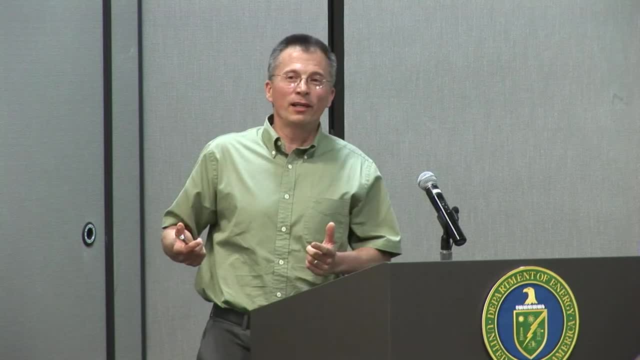 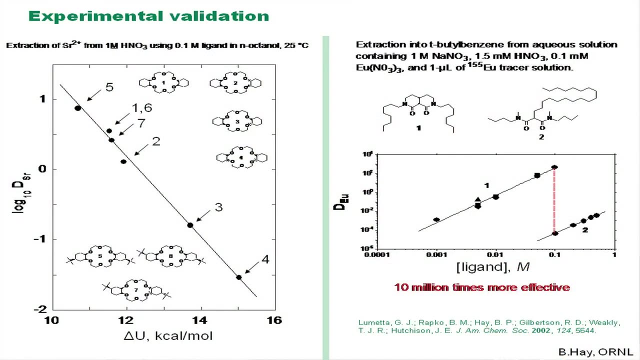 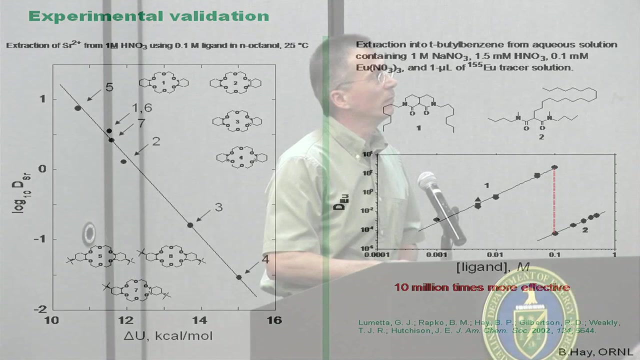 we get better distribution coefficient. This is good. These models can't predict distribution coefficients, but they can provide ideas of trends. Okay, these computational models do these binding of metals in a vacuum? Okay, they're not in a solvent, They're not going to get a number of the effects. 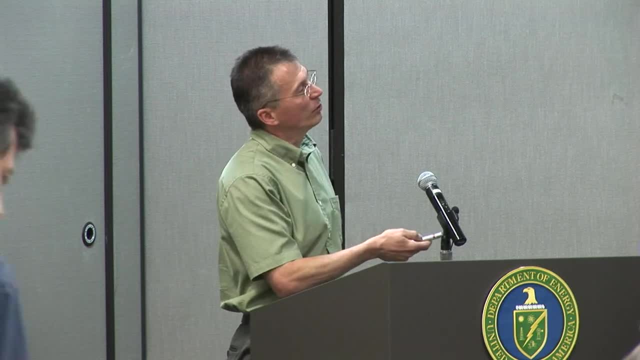 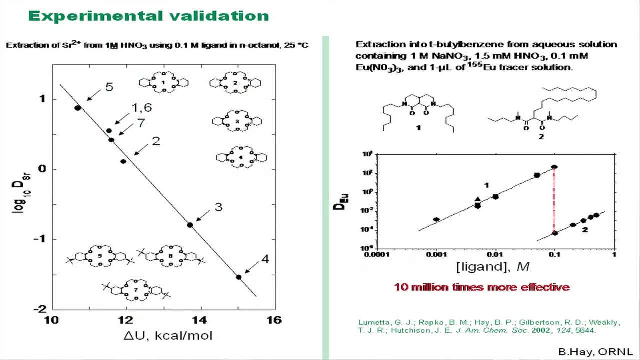 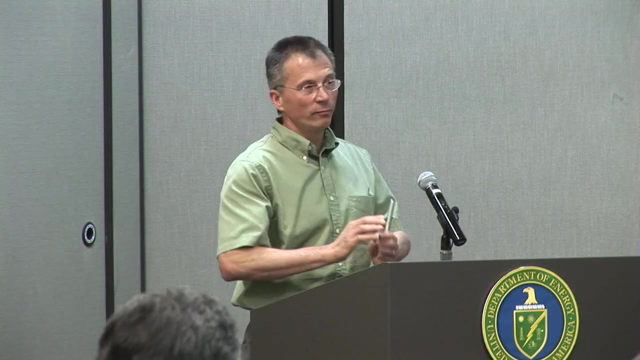 but they do help focus the work. Here's another example where you see a molecule that's 10 million times more effective by basically just by- Well, right here, by putting this structure here, it makes the molecule much less flexible, and so then it binds. 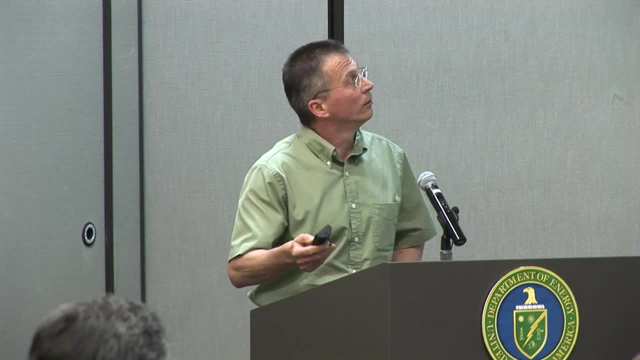 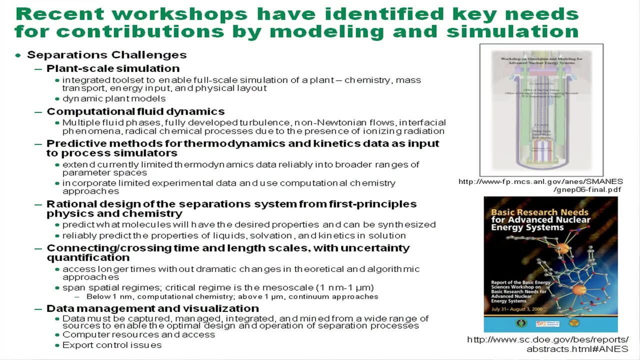 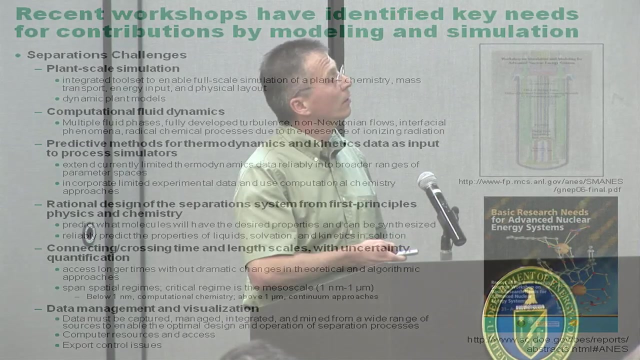 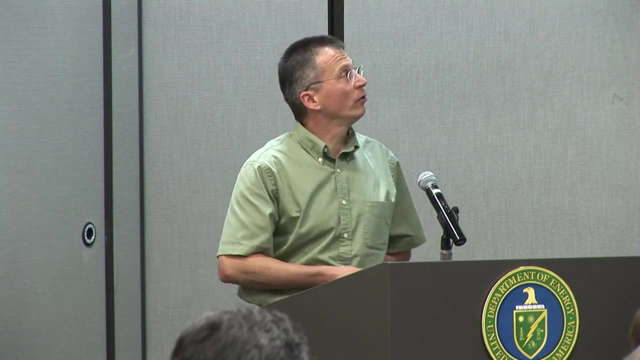 It's prearranged to bind the species. Okay, This is kind of historical. Where were we? Recent workshops have indicated the need for, or the opportunity for, modeling and simulation. I won't read these in details, but it is given in your handout. links to these reports. 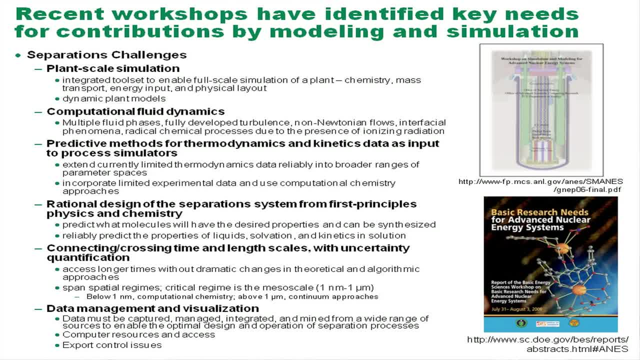 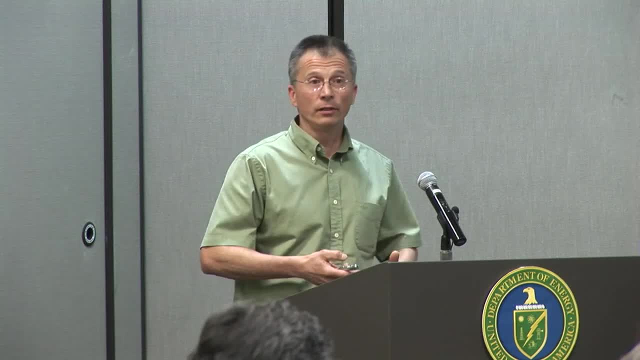 But basically they point out there's several places where modeling and simulation can help. A plant scale simulation, dynamic plant models, are seen as really useful, primarily in the near term. I think it's more useful for kinds of a safeguards analysis than it is for plant design. 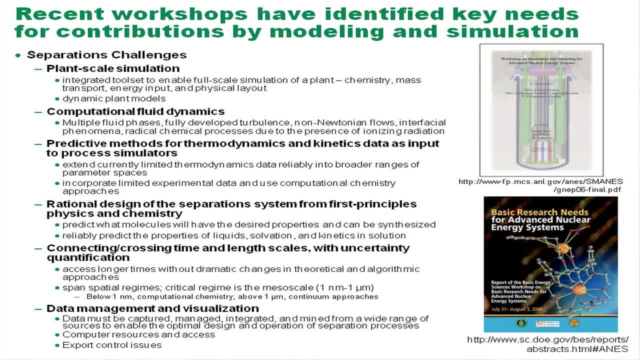 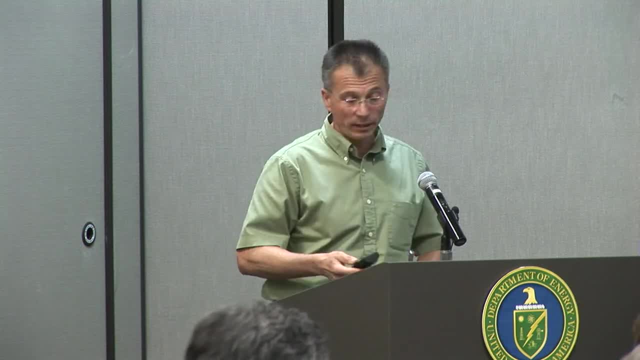 But down the road, when we get to designing plants, it'll be useful. Computational fluid dynamics- we've seen in previous talks that the fluid dynamics is vital in these contactors- Predictive thermodynamics and, as we move along, data management and visualization. 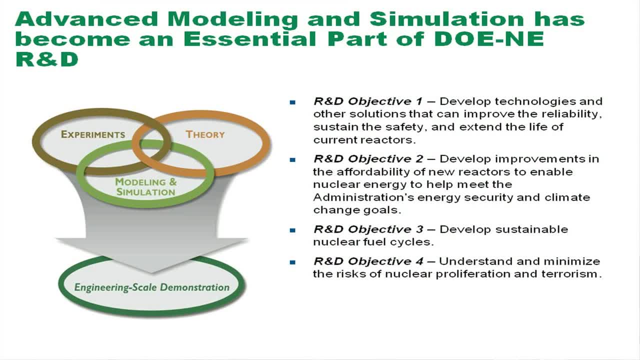 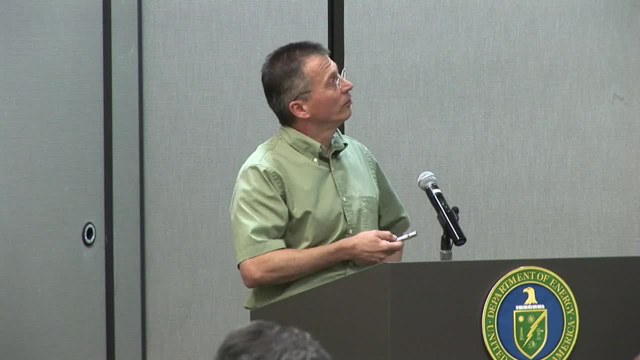 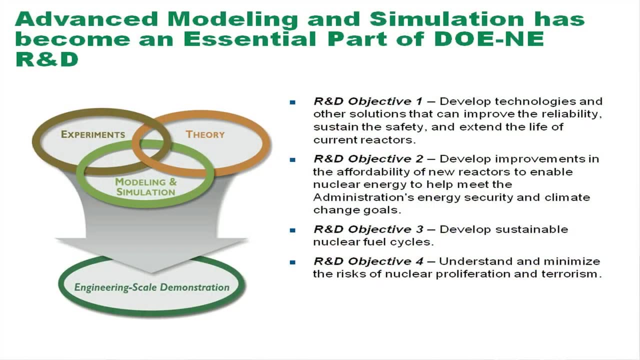 So a few years ago the Office of Nuclear Energy recognized the need for advanced modeling and simulation And actually now, if you look at the nuclear energy roadmap, you'll see that modeling and simulation is given an equal footing with experiments and theory. 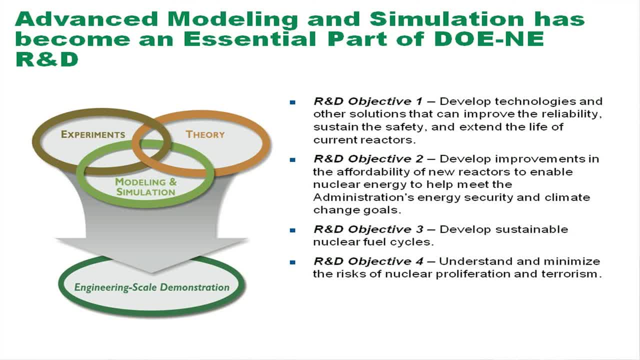 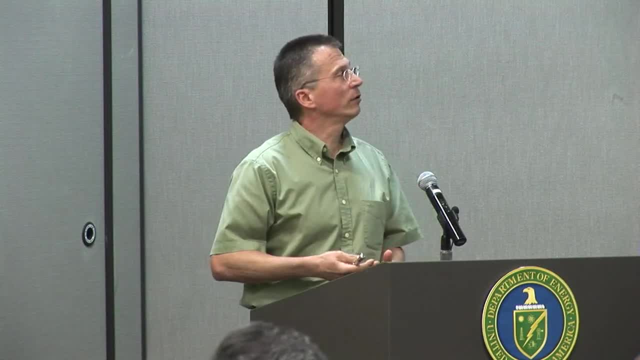 And what we've been doing in the safeguards and separations portion is focusing on R&D objectives of NE, both in Objective 3 and 4, which is sustainable nuclear fuel cycles, but also designing tools that could be useful for safeguarding systems of the future. 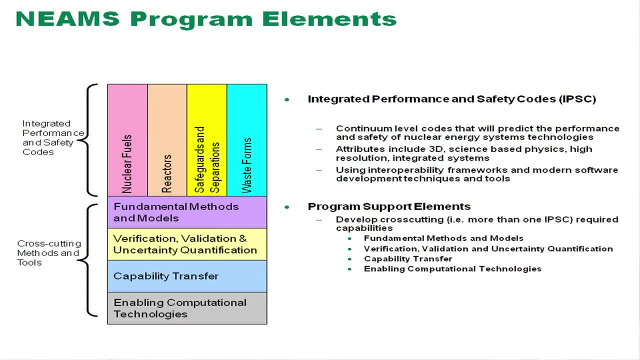 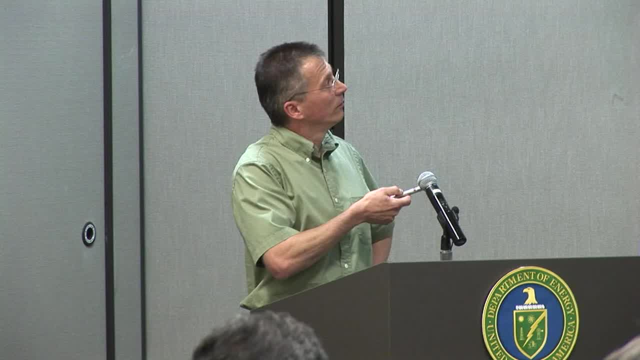 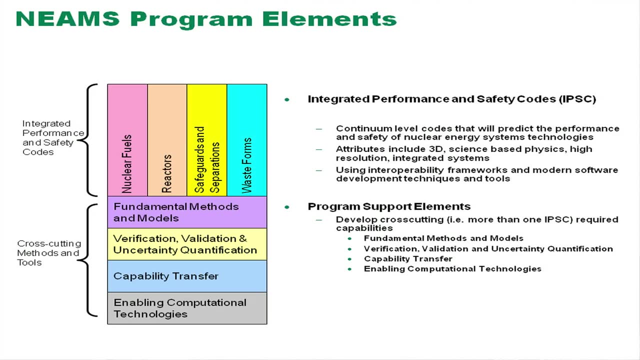 And so the NEEMS program, the Advanced Modeling and Simulation Program is looking at, has four code efforts or has had four code efforts: reactors, fuels, separations and safeguards and waste forms, and then some cross-cutting efforts. 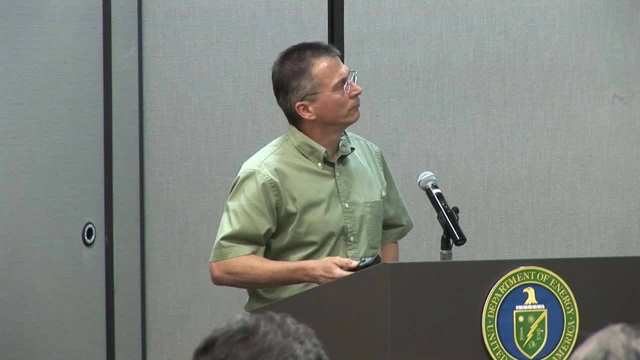 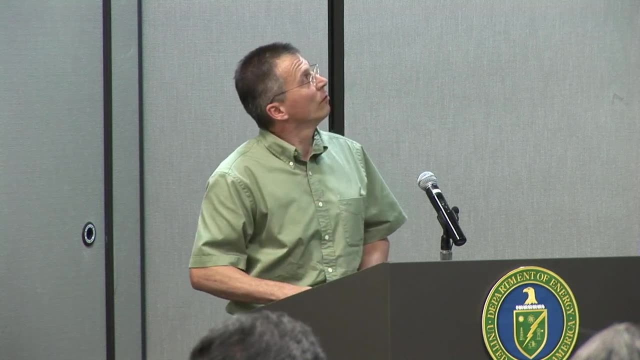 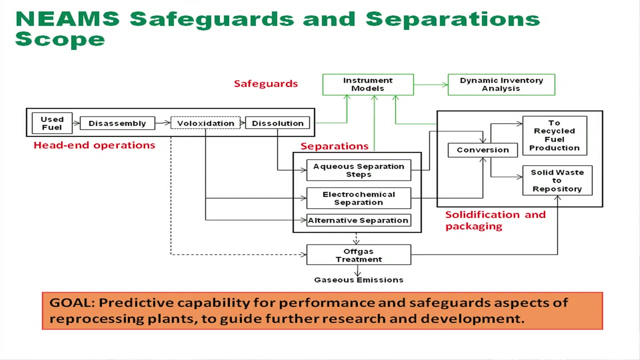 on computational cross-cutting capabilities And so, within the safeguards and separations scope, what we've been looking at is developing an overall plant-level code. So we're looking at the scope, the head end, different separations processes, including aqueous, electrochemical. 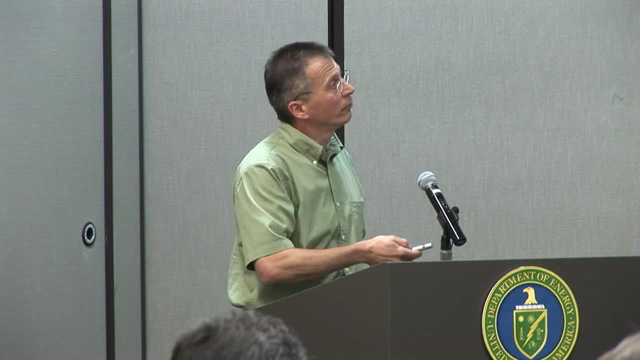 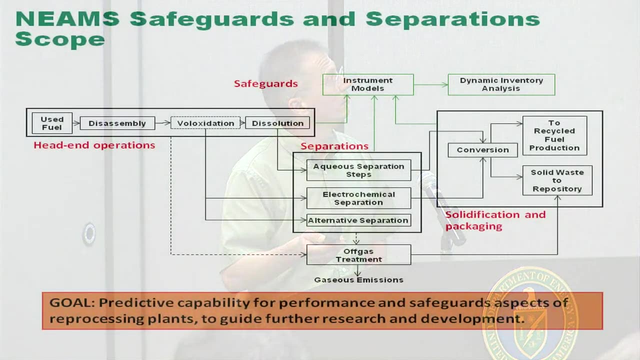 and then alternative approaches, integrated off-gas treatment, and then the solidification and packaging of the process. Integrated with that, though, would be safeguards, So instrumentation models, and then dynamic inventory analysis, So developing the tools such that those people that will be designing 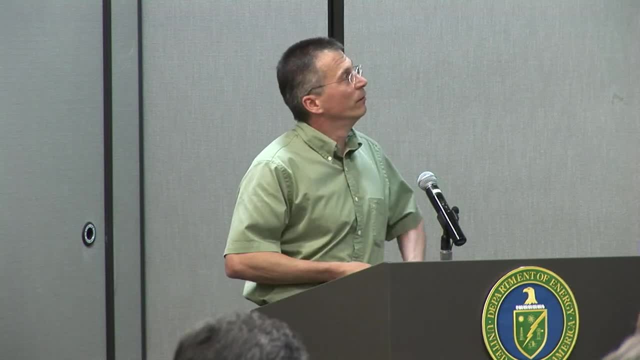 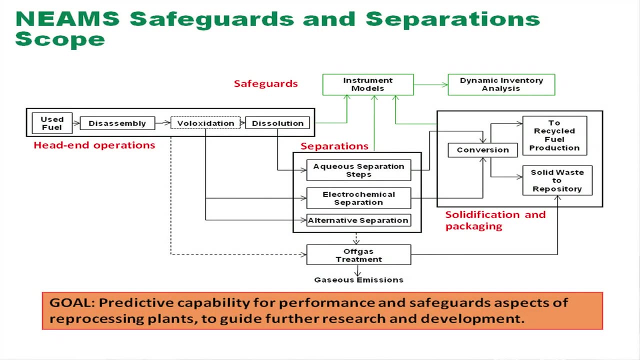 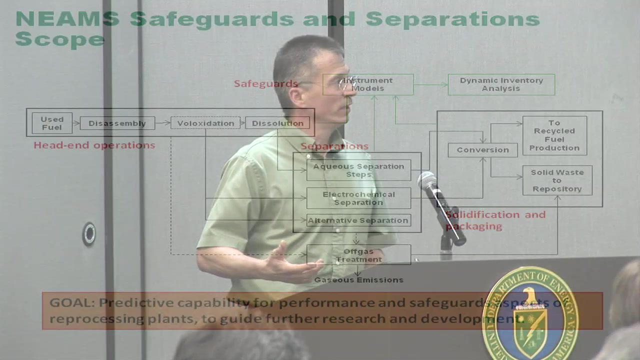 or considering different fuel cycle options, will have a toolkit at their disposal where they can mix and match the different models and allow them to compare, And so the goal of this effort is a predictive capability for performance and safeguards aspects of reprocessing plants. 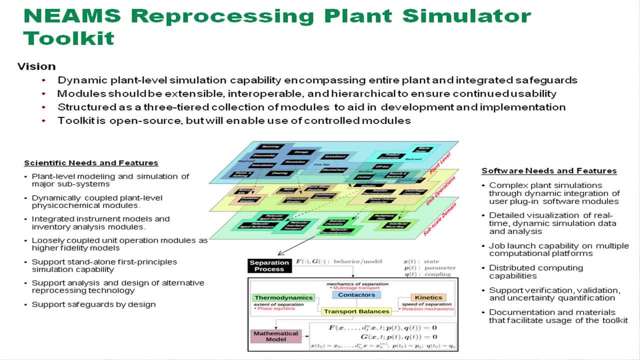 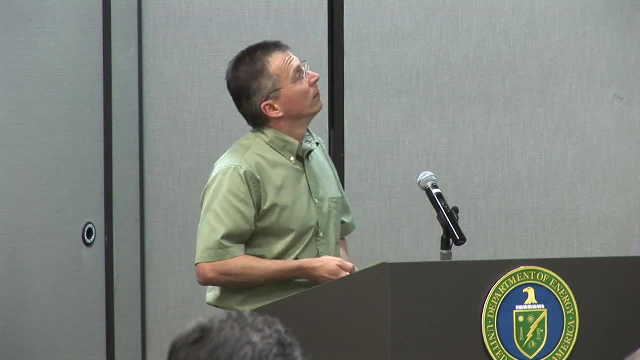 Okay, so the vision of this is a dynamic plant-level simulator, and so that's kind of depicted by this blue tier. Okay, this is a plant-level model that encompasses the entire plant and its integrative safeguards, or a portion of the plant. 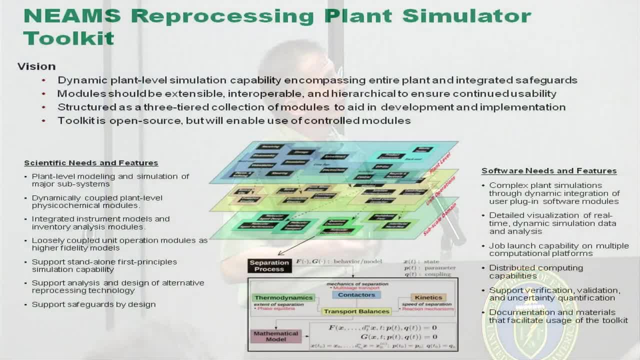 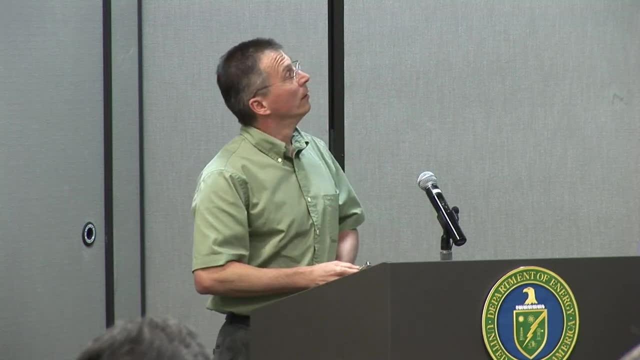 One of the key points here is: these models should be extensible, interoperable and hierarchical. Basically design them today so that you can use them in many different uses for the future. Design them with where is computing going to go, not make them very limited. 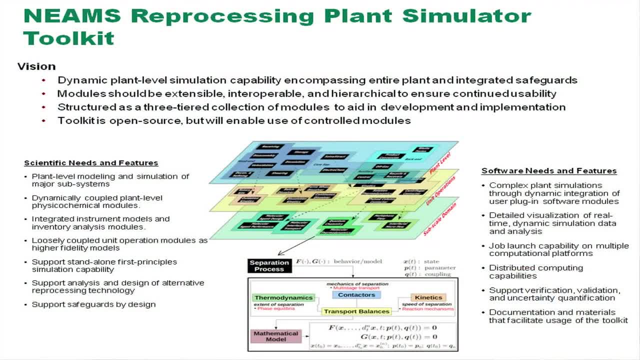 Open source toolkit rather than some sort of proprietary licensable approach, But enable the use of controlled modules. So the idea is okay. we'll develop this overall toolkit, but if you have a special program that you want to link into it, you can. 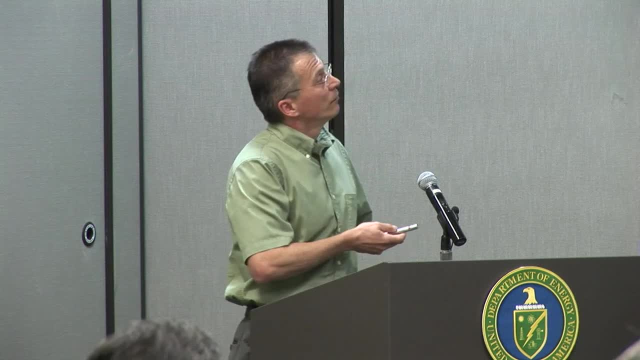 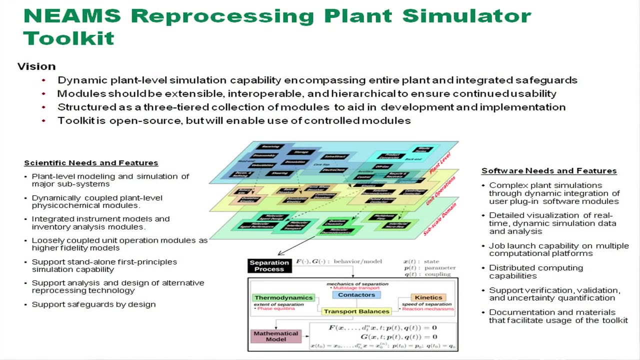 And keep it proprietary. So the idea is an overall plant toolkit, but where you need it, then you have more detailed models. So these would be models of specific unit operations at a more detailed level and then down at this bottom tier. 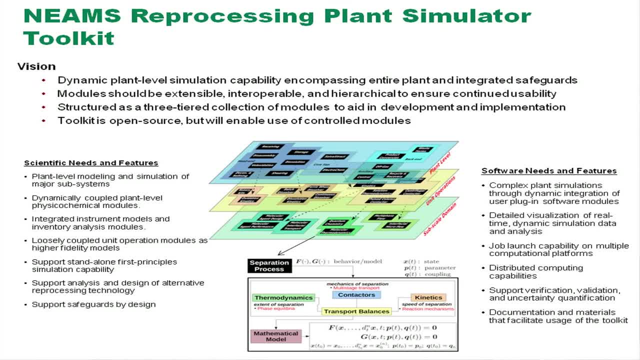 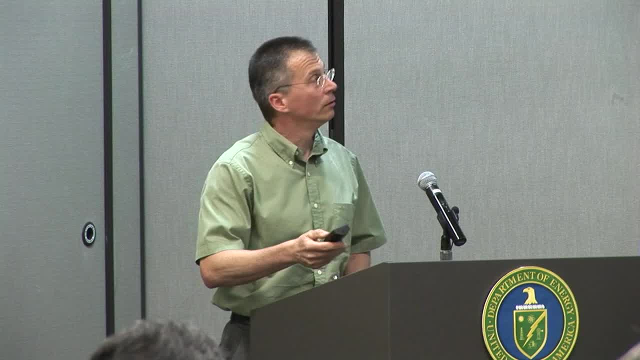 would be where you would actually do things like a molecular model, where you need to get a parameter to then feed up to your higher-scale models. Okay, there's a lot of stuff on this slide and I don't intend to walk through it all. 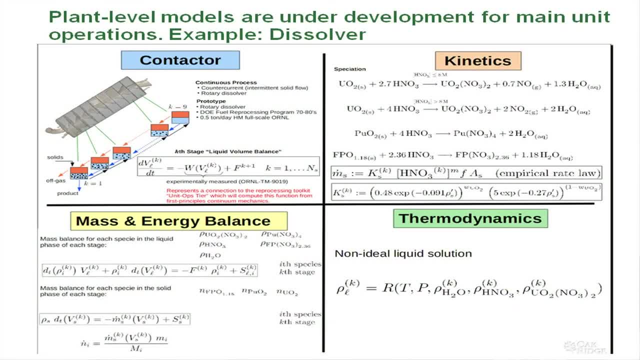 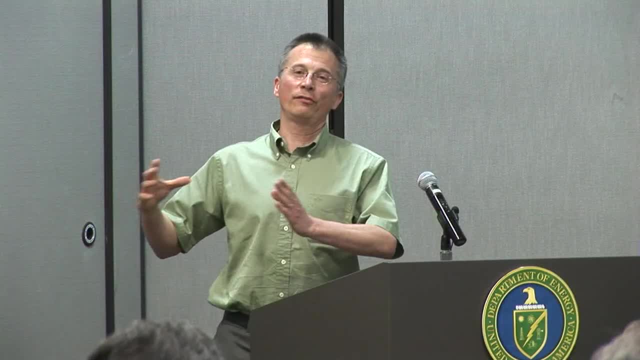 but this is just an idea of what's being done right now for main unit operations, And the idea is to get this all in a common scheme. If you go look at the different models that are out there from, you know, decades ago. 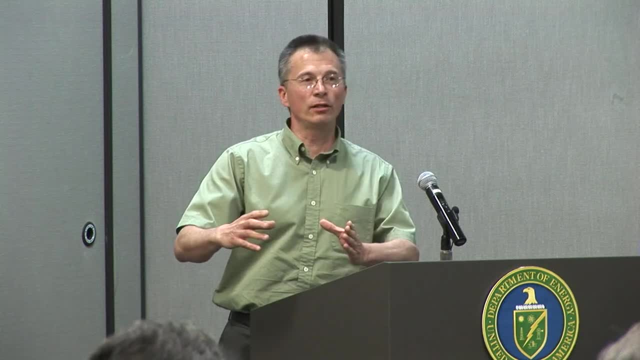 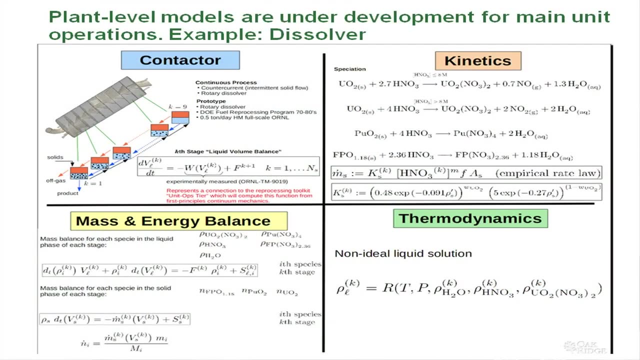 you'll have a very dedicated model, okay, And so if you want to make a change to it- like if you say I want to change from a centrifugal contactor or a mixer settler to centrifugal contactor- you're going to have to go dig in there. 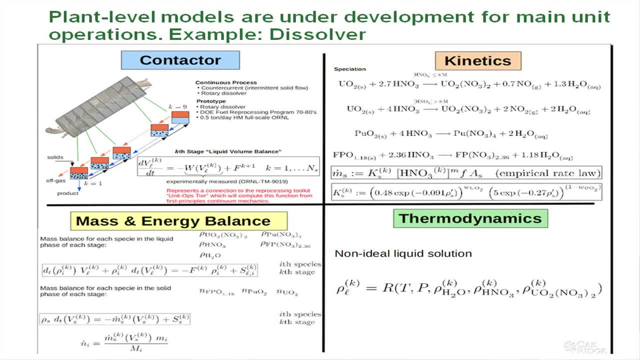 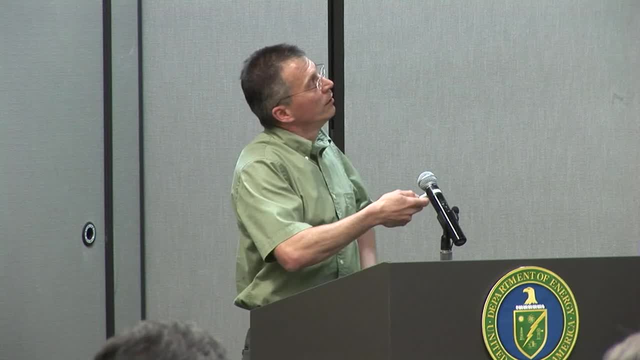 and do an awful lot of work. So the idea is: can you develop on a common framework such that you have an overall- let's say- and this is an example of a dissolver- overall contactor which gives how the different materials are contacting? 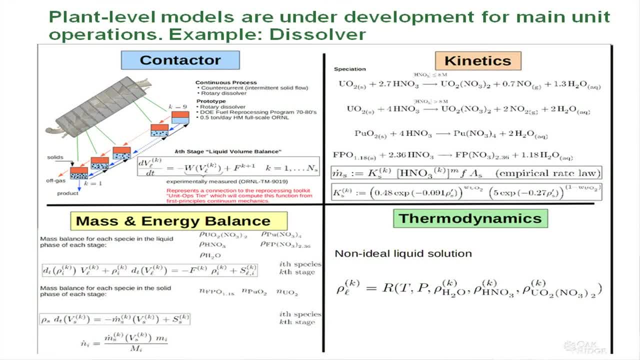 a mass and energy balance, any kinetics and thermodynamics, Each of these is a separate module. So if you say, well, hey, you know, I don't want to use the thermodynamics from, let's say, a muse, 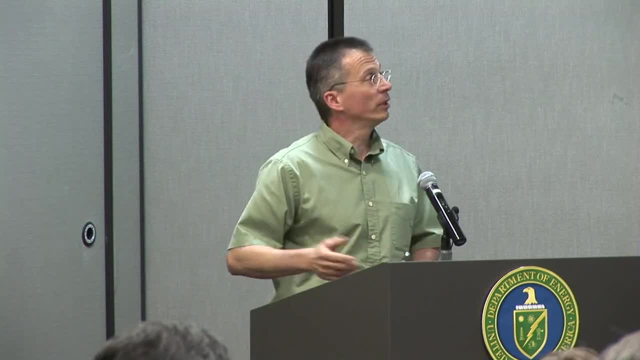 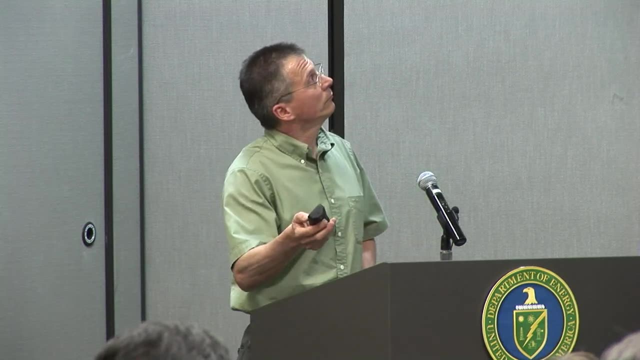 I'm going to use this, I'm going to use some other thermodynamic predictor. I can just plug that in there rather than starting from scratch. Okay, so now I'm going to hone in a little bit just on what's happening in solvent extraction. 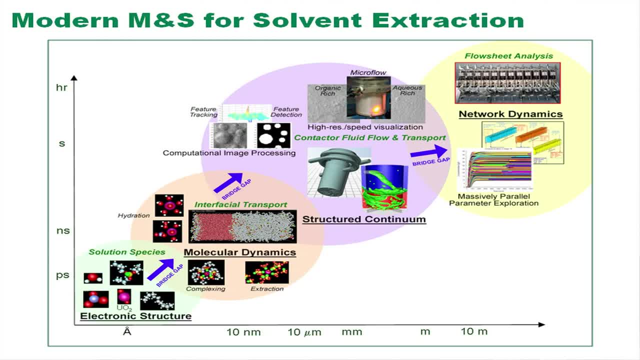 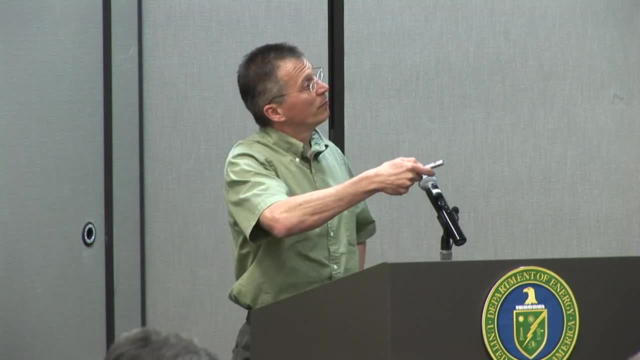 since that's where most of the development work has been going on historically. If you look at solvent extraction, what makes it tick? Obviously you're interested in what happens up here at the meter length scales and the hour time scales. How does this thing perform macroscopically? 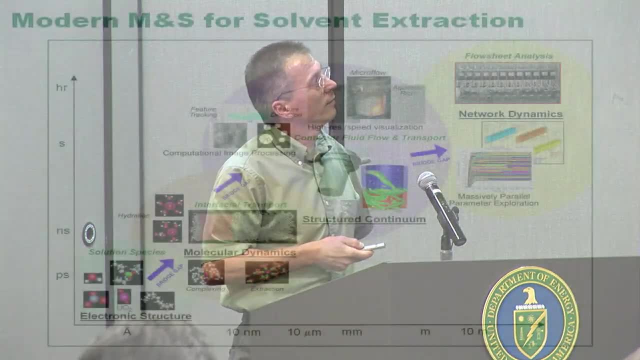 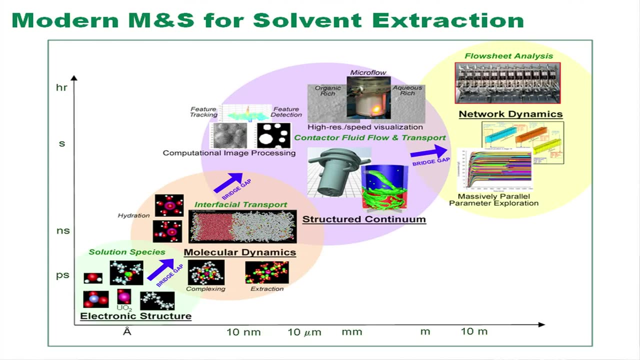 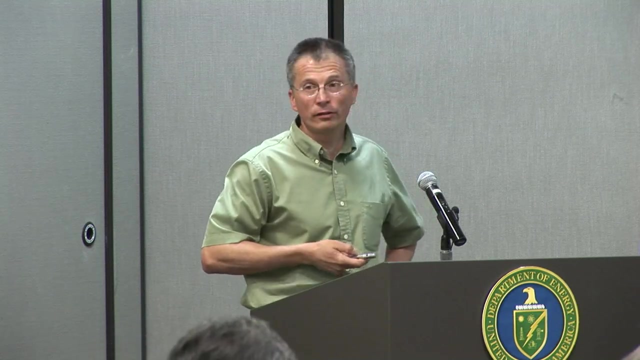 But if you look, there's a lot of different things going on at different scales that affect the performance. Ultimately, you have these different fluid phases that are contacting and the materials are passing between the phases. so how you contact these fluids is important. 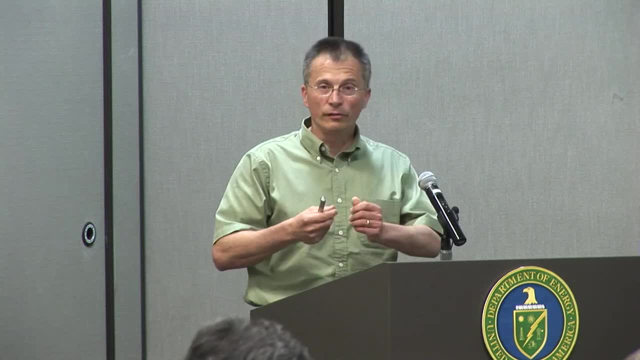 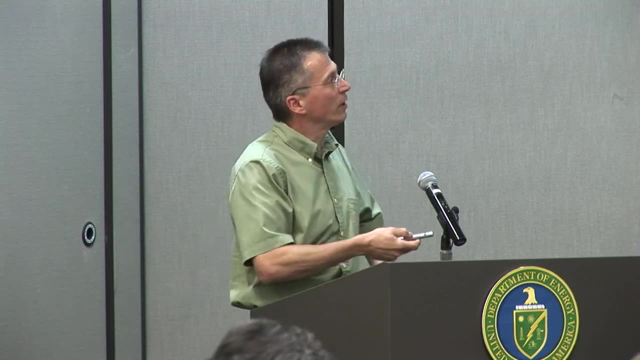 If you go down one scale now at the interfaces, that's where the action occurs At some point. this material has to go from one phase to the other phase and it has to go through an interface. Understanding what happens at the interface. 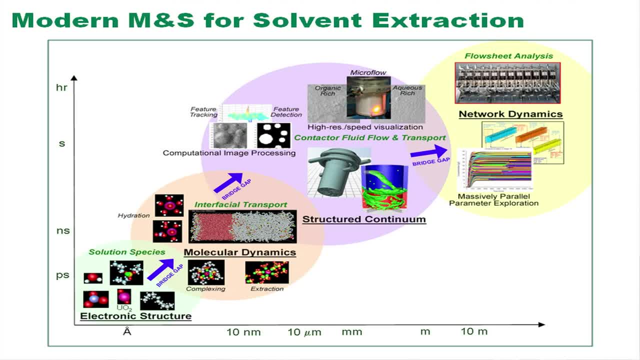 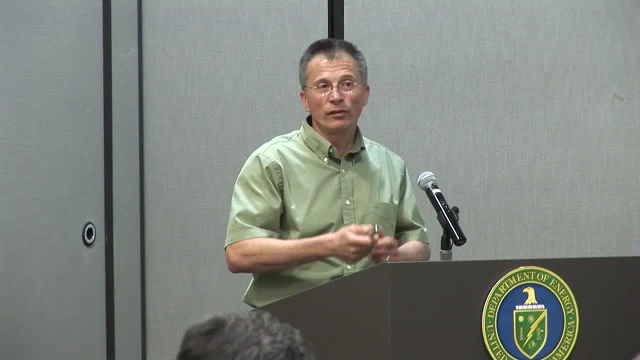 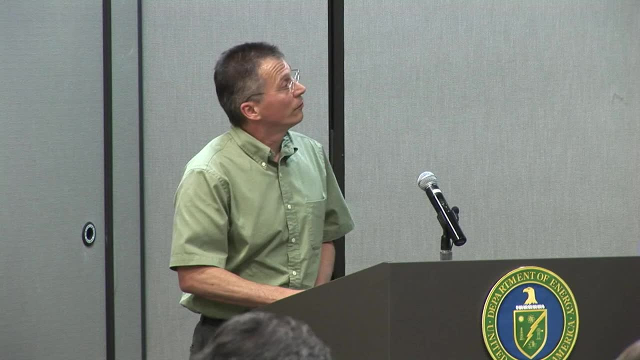 that's at a molecular level. And then actually, if you want to become more predictive, it's can you do things down at the molecular level to feed, provide parameters up to understand what's happening at the upper scales. Okay, so here's some examples. 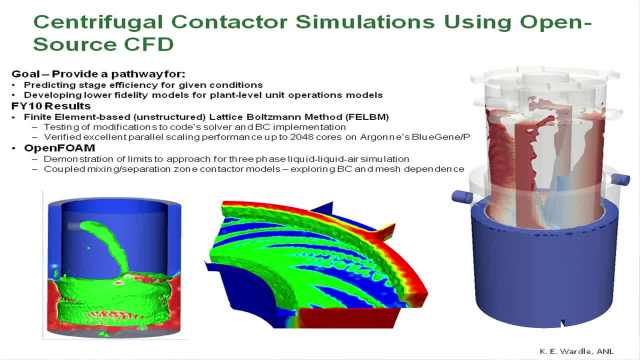 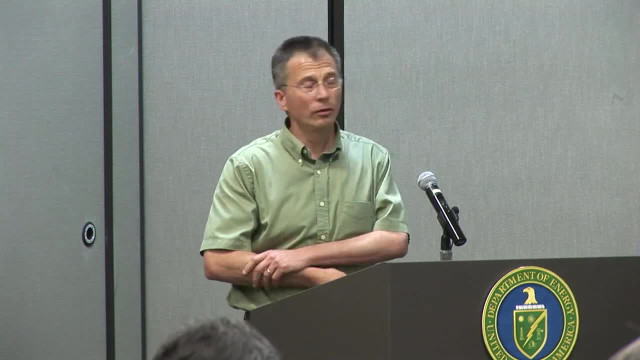 This is some work that Kent Wardle of Argonne has been doing in modeling the fluid dynamics in centrifugal contact And he's been using an open source code called OpenFoam. He started with some commercial codes and recognized they just don't have enough capability. 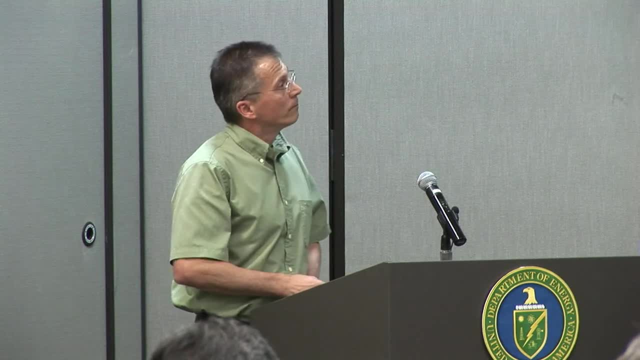 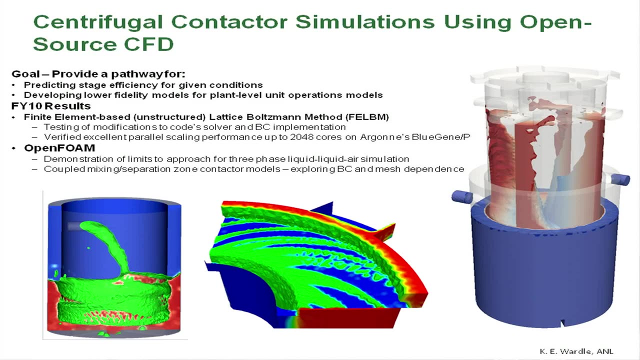 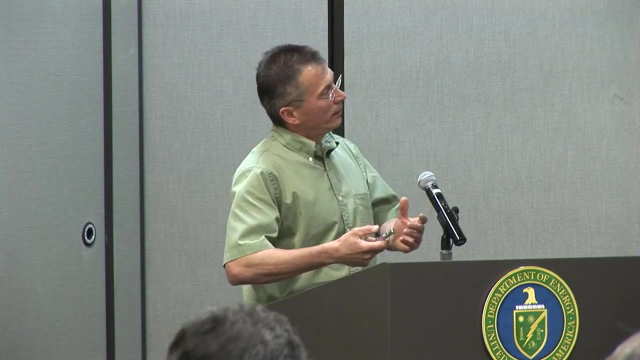 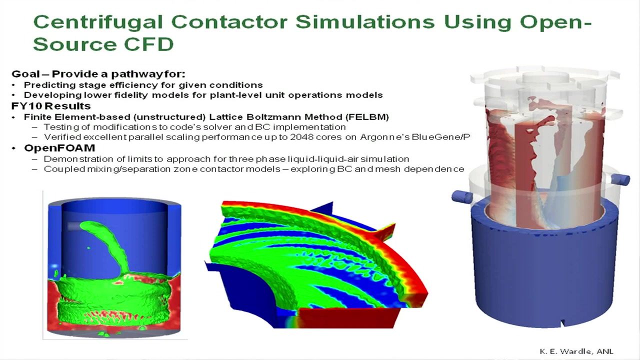 to do what he wants to do. These are just stills from some of his animations, where here the red is basically a surface where there's an organic phase, The green is an interface and then the blue is an air interface, And what you see here, actually, 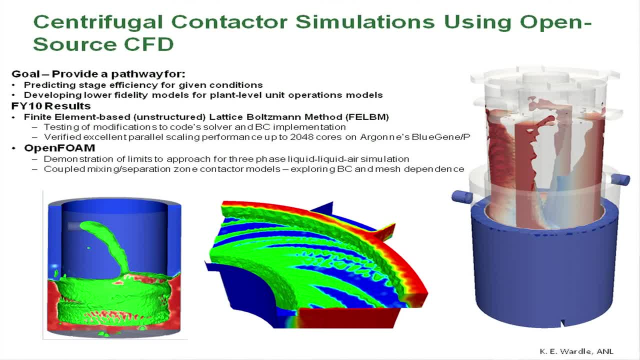 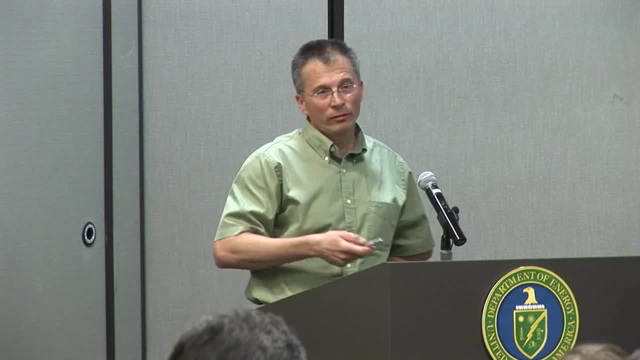 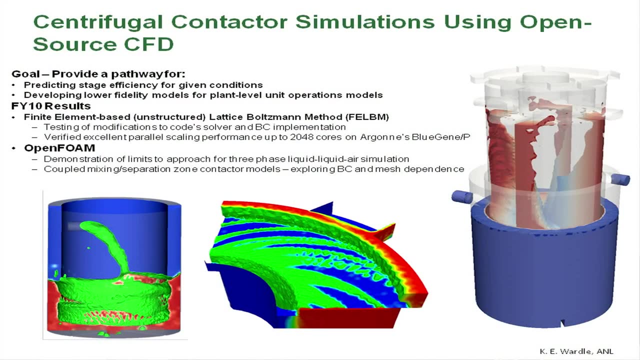 this is a very interesting point. This is at the top of a contactor where the liquids are coming out and going to the collector And through the simulations they were seeing some problems in testing. Actually, at Savannah River they were seeing some siphoning. 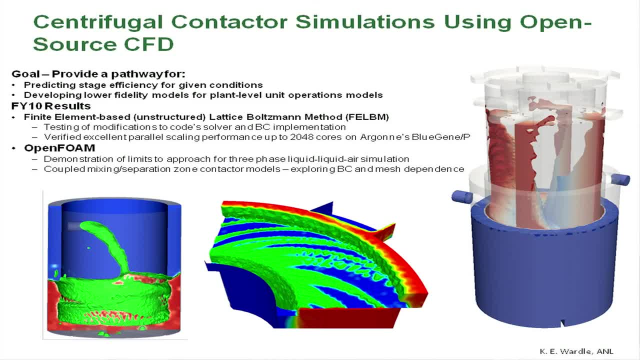 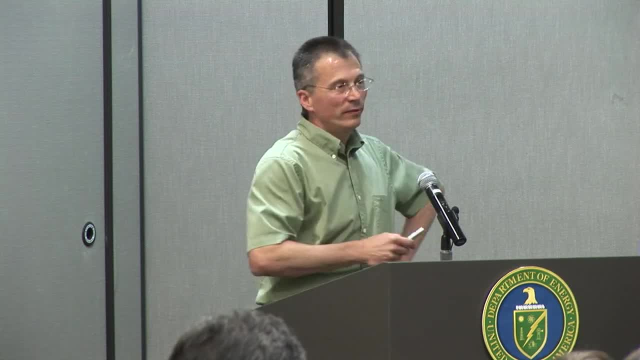 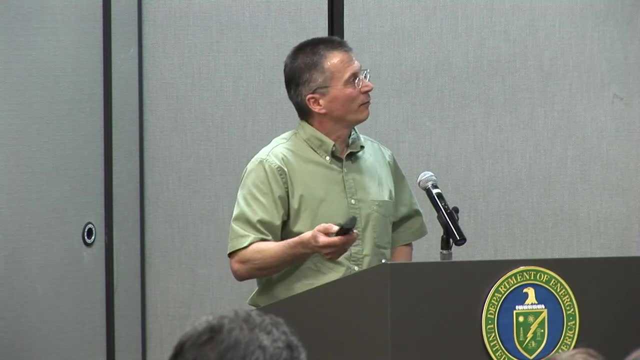 And he was able to show that it was a siphoning effect, that if they were able to vent the top of these contactors, they would be able to keep the siphoning from occurring, And that actually proved to be useful. So that's one example of how these are useful. 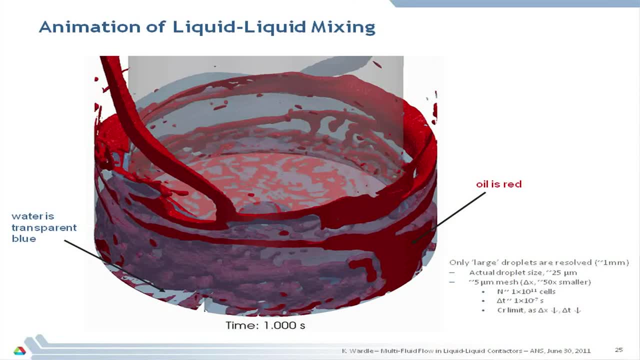 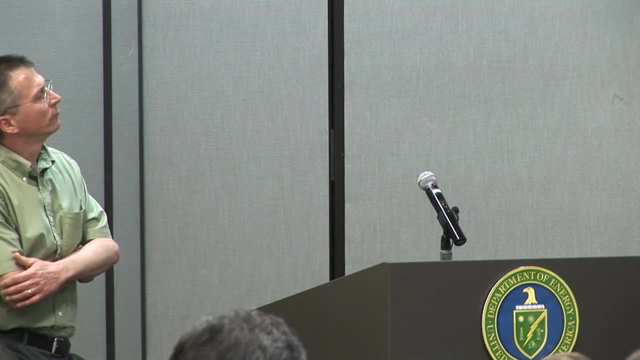 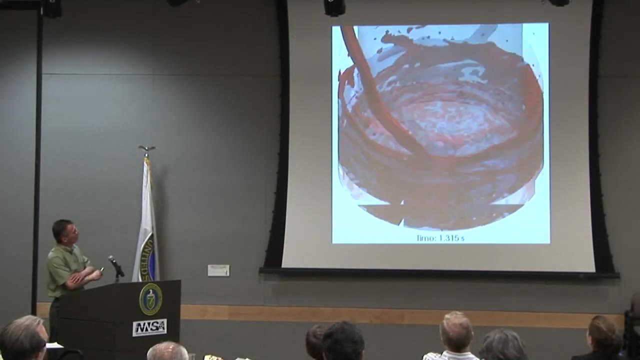 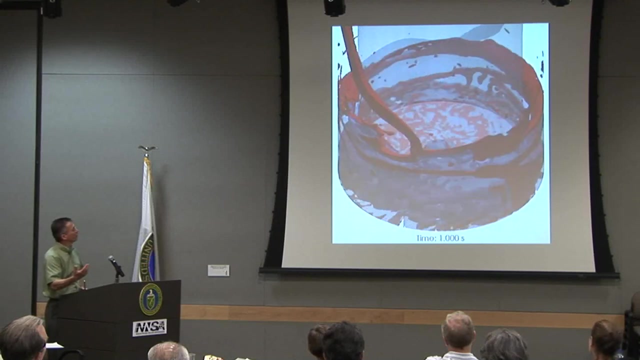 And here's where I've got the animation. So here you're seeing the red phase, there is your organic phase And then the kind of clear bluish is your water phase, And so this kind of gives a macroscopic view of what's going on in these contactors. 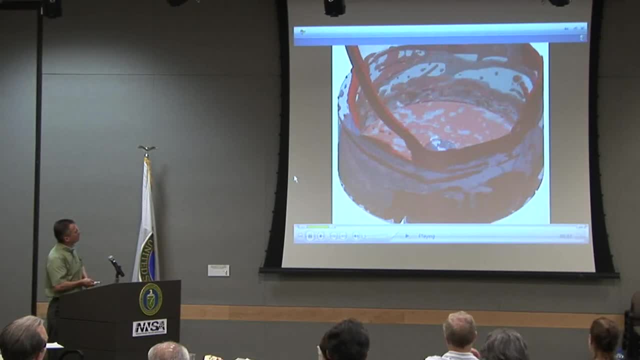 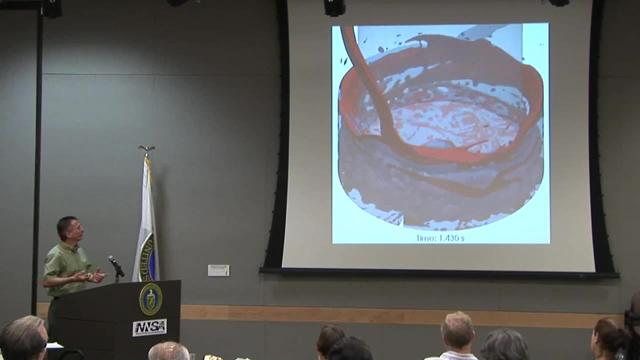 It's a very complicated flow. I mean you can see it's mixing around. You're getting large globules, you know, And very dynamic, And actually if you watch this, the level goes up and down. Now, if you run this at different phase ratios, 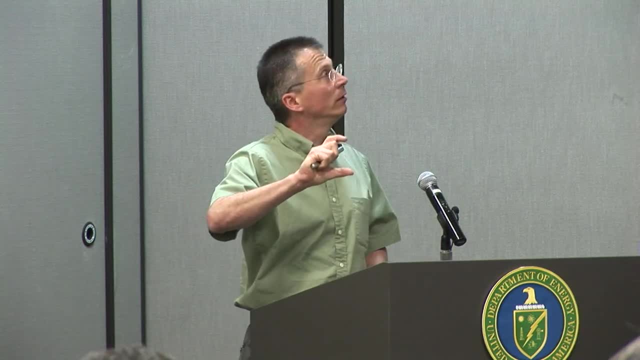 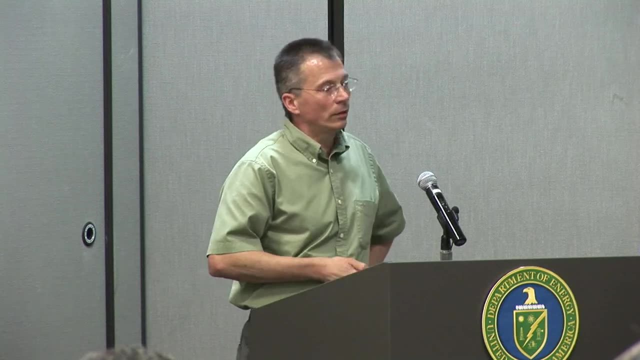 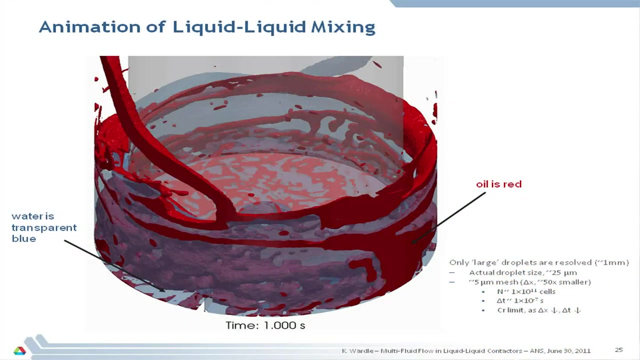 different speeds. what you'll see is you'll have different levels in the contactor, which means you have different volumes in the contactor, Different residence times, So this can do a lot towards predicting how much holdup you have in these systems. 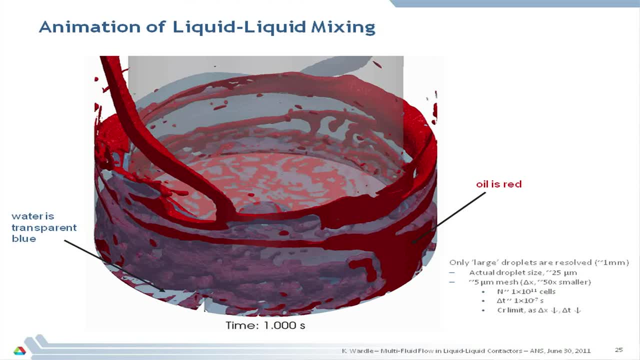 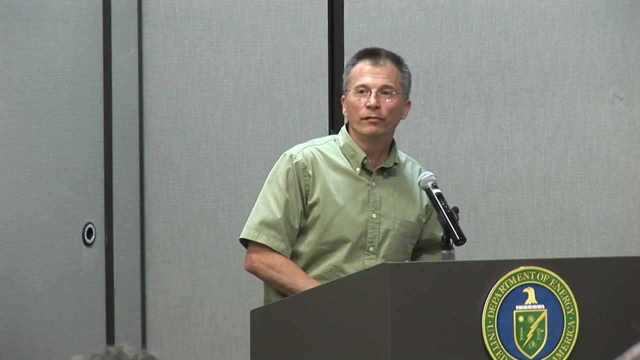 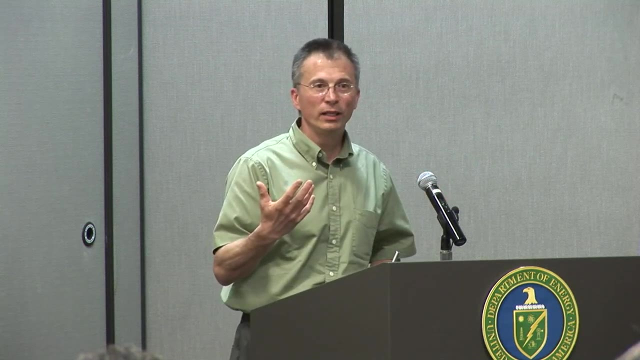 what's the dynamic behavior? But one thing that's important here is you only see the large globules. This can get down to a scale on the order of 50 microns, but we know the droplets are much smaller than that At the current time. this can do macroscopic fluid behavior. 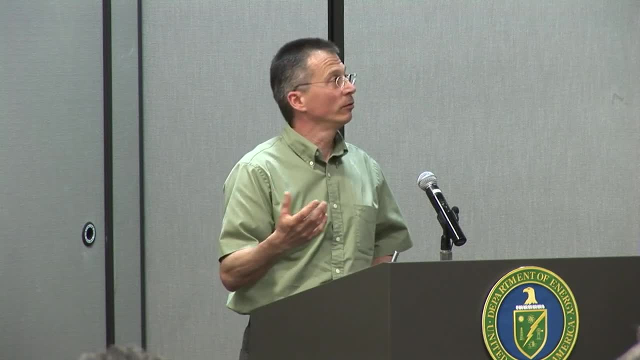 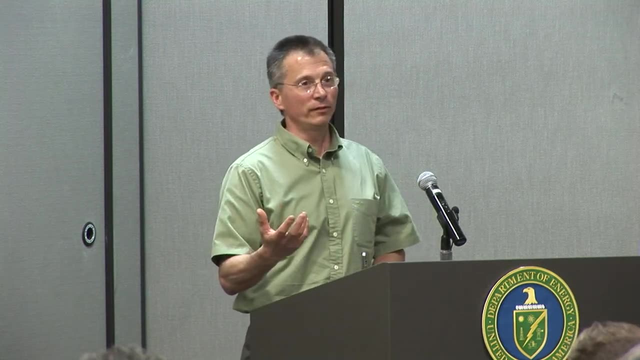 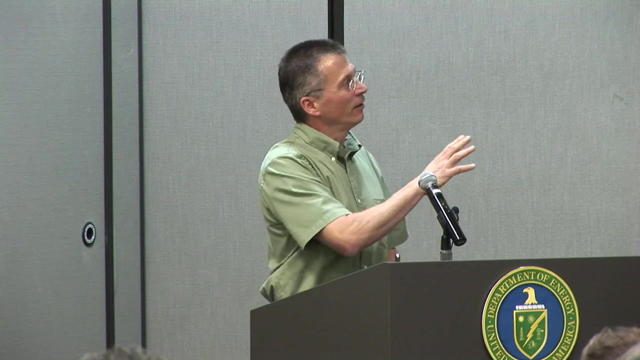 but it can't get down to macroscopic fluid behavior. So a current focus is: how do you link models down at the droplet size scale with this more macroscopic multi-phase flow modeling? Already this is a very large simulation, So now how do you move forward? 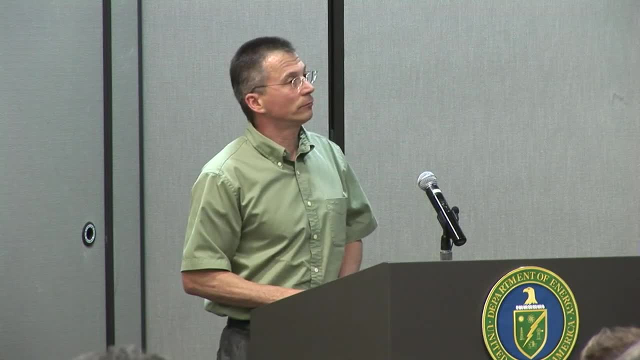 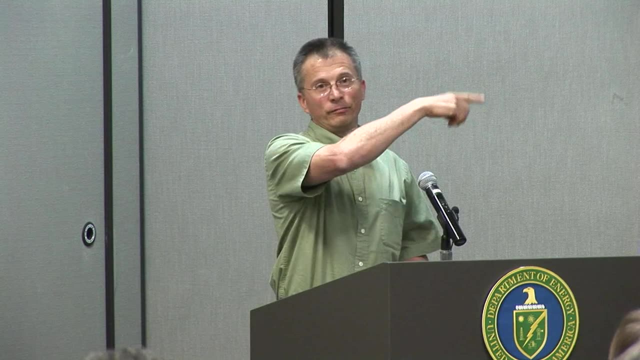 And so let's go back to the slides. How do you validate it? I'll show you some efforts that are being done experimentally In a few slides. But yeah, that's great. How do you validate And how do you get parameters in there? 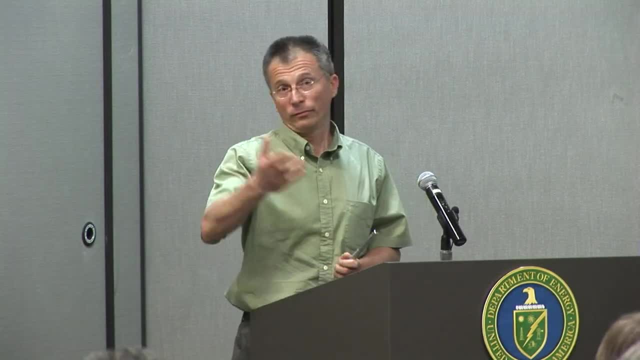 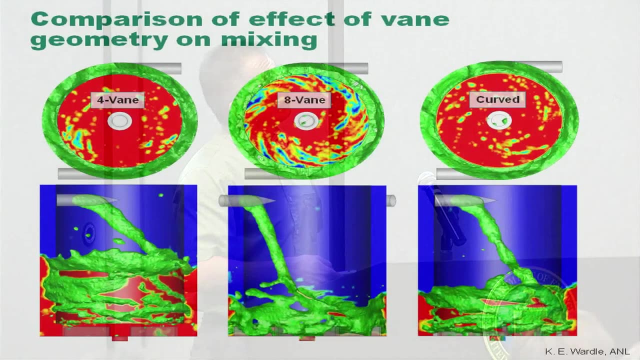 Where do you get the parameters to put in there? Yeah, calibrating is extremely difficult, And so here it shows some other examples of the different performance you get with. Here it's looking at the veins at the bottom of the contactor. 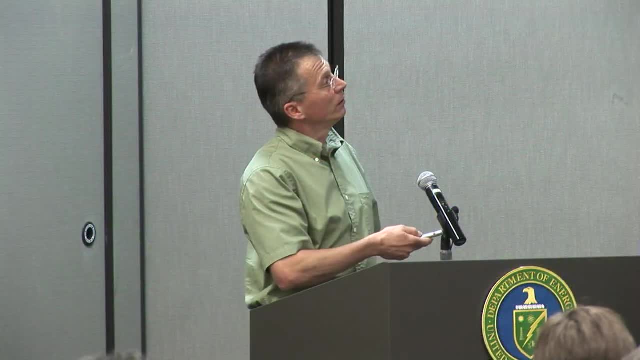 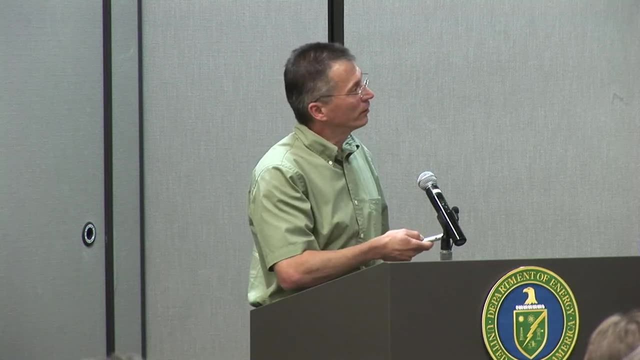 Four veins, eight veins and then, if you have curved veins And you'll see under the same conditions, you obviously see a much different liquid level, much different contacting. Here you see very little red fluid, You only see the green. 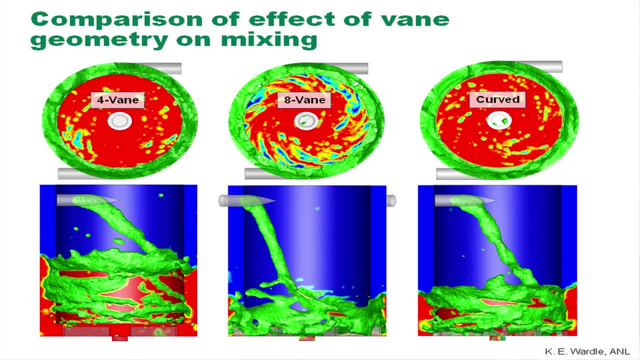 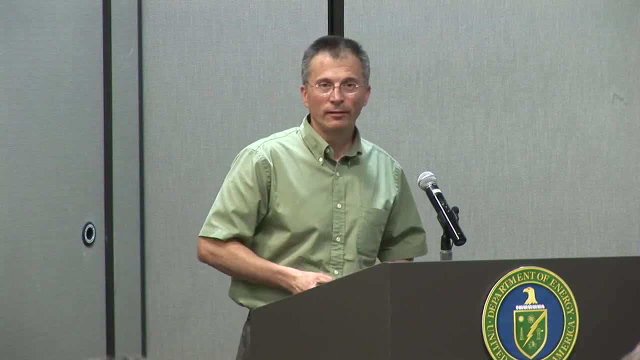 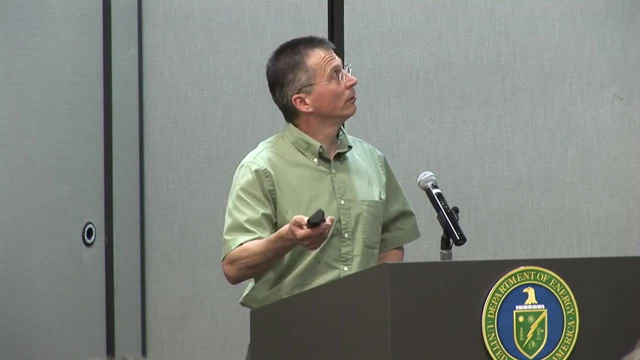 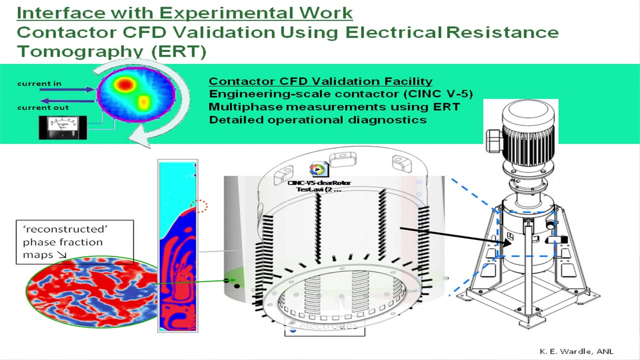 So it gives you some idea of what's happening experimentally, And then you could obviously tweak the design of these veins and then predict performance, so that it'll help you guide your design. Okay, so here's some things going towards validation. These are some experiments that are going on. 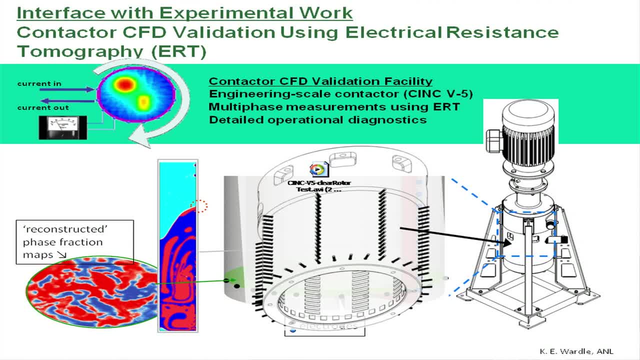 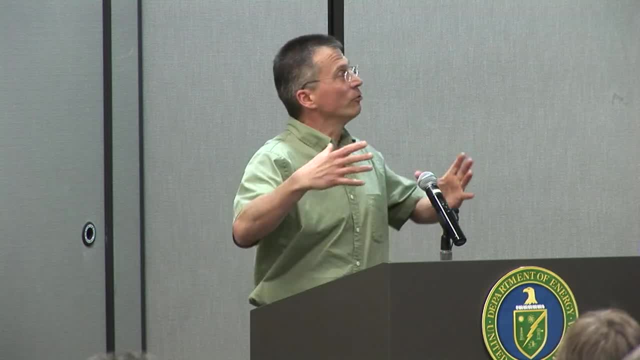 There's some experiments at Argonne and some at Idaho right now on electrical resistance tomography. So what they're doing is putting a bunch of electrodes around these contactors, a huge number of electrodes, and then probing the connectivity between all the electrodes systematically. 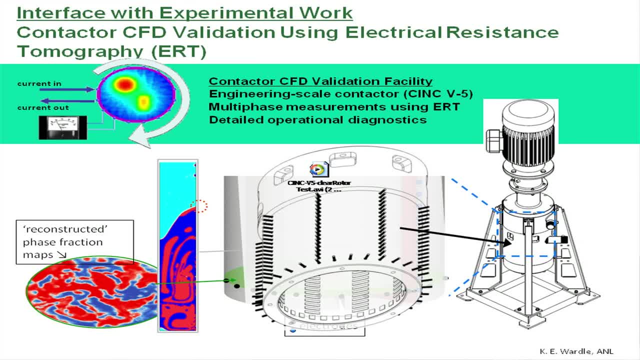 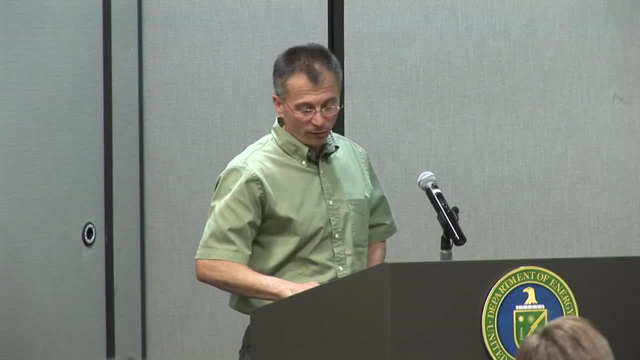 using a commercial tomography device, And what it allows them to do is under different sets of conditions. then get phase maps. At least you can map out where's the conductive fluid, where's the nonconductive fluid. It's not going to get down to the droplet level. 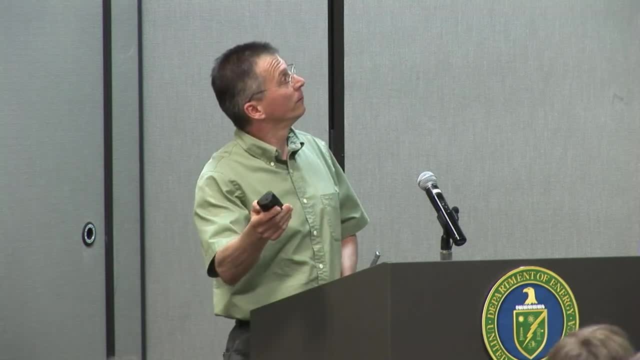 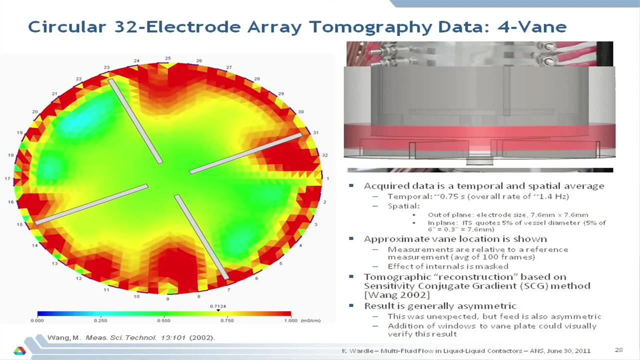 It's still going to be very macroscopic, And so here's one map that they collected, And so here you're looking at a horizontal slice down below the rotor, So you're looking down in the veins and you can see where there's. 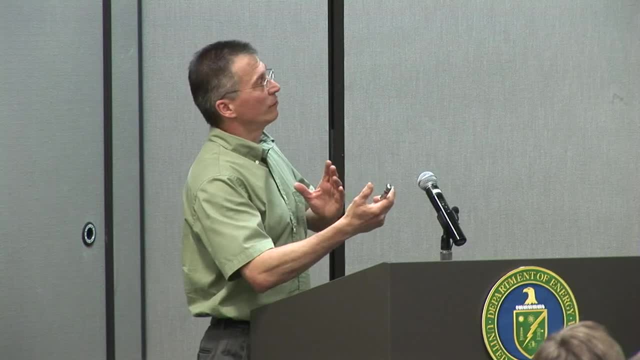 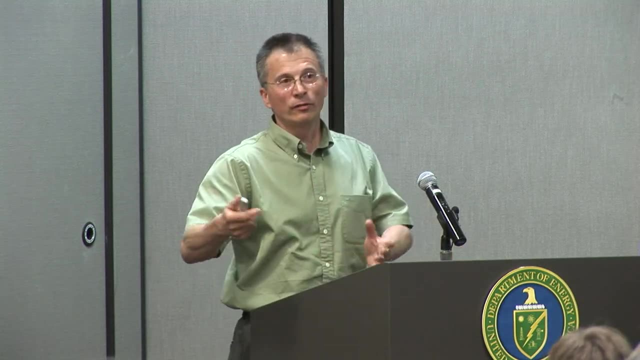 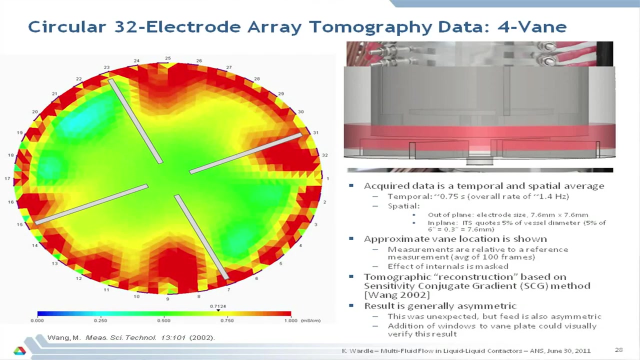 basically a distribution of conductivity And you can see where there's conductive zones, nonconductive zones. So the nonconductive zones are heavy in the organic and the conductive zones are heavy in the aqueous. But this is a far way from actually validating a model. 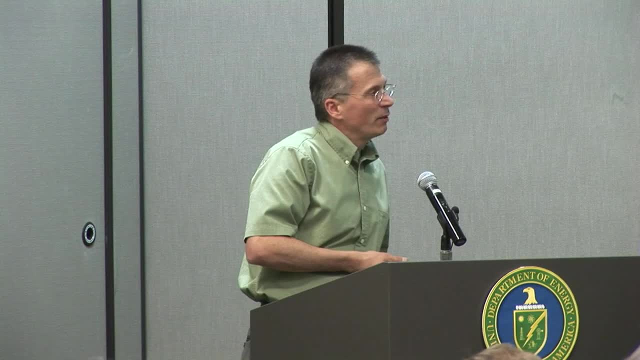 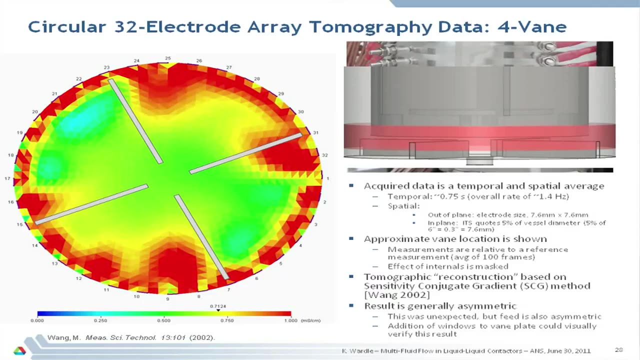 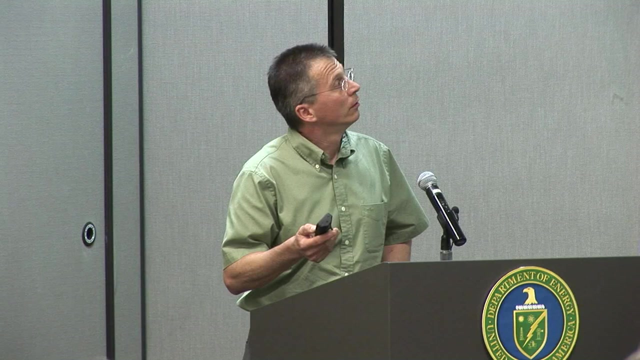 because this is time averaged over on the order of a hertz And, as you saw, when this thing is spinning at 3600 RPMs, there's a whole lot more action going on than that. So this is kind of a smeared experimental investigation. 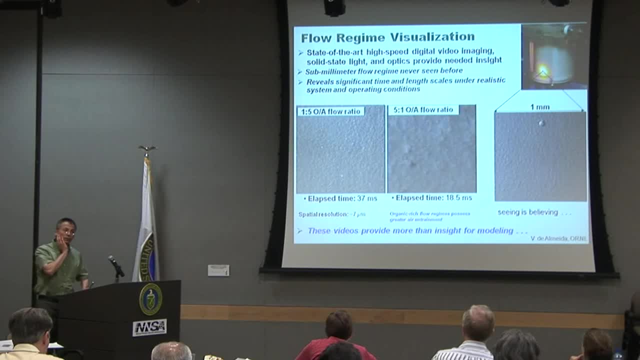 All right. So here's another potential way to validate, and this is high-speed video imaging. Now, the issue here is: when you see these contactors running, they're opaque. I mean it's an opaque, It's a cloudy mixture. 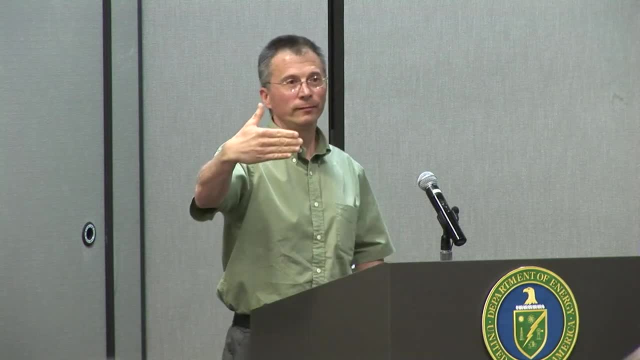 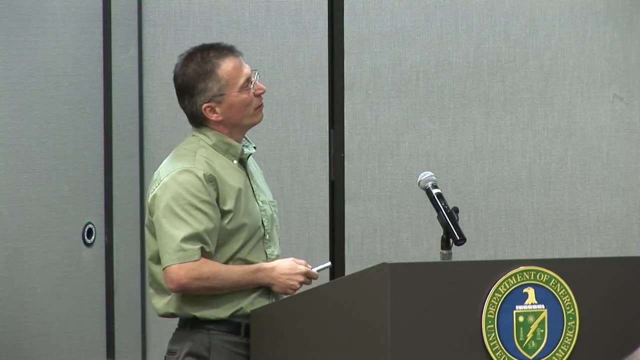 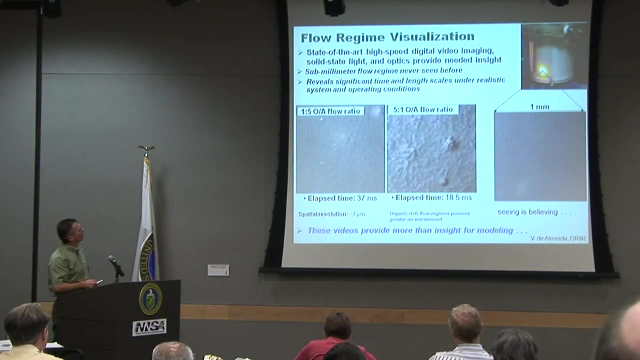 Okay, So high-speed video is only going to see the first. you know, the first few microns or depth, Well, tens of microns depth. But if you go use a high-speed video system, and this is a, these are about 5000 frames per second. 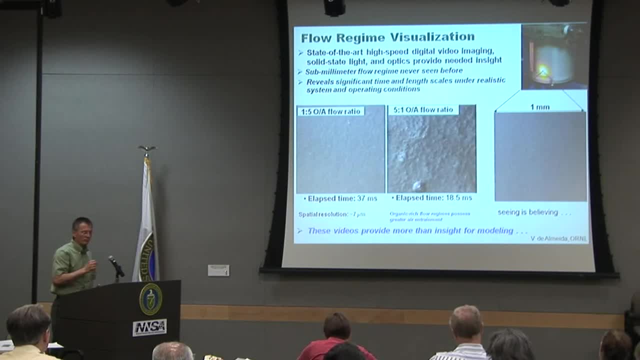 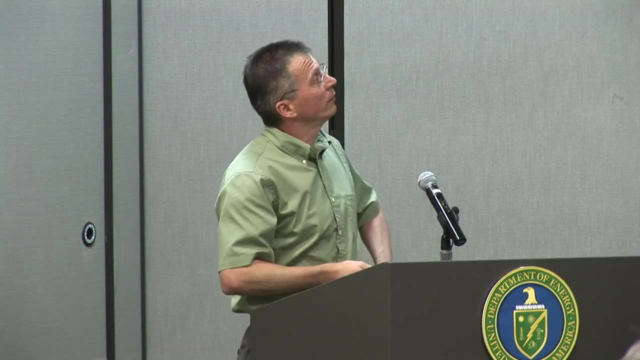 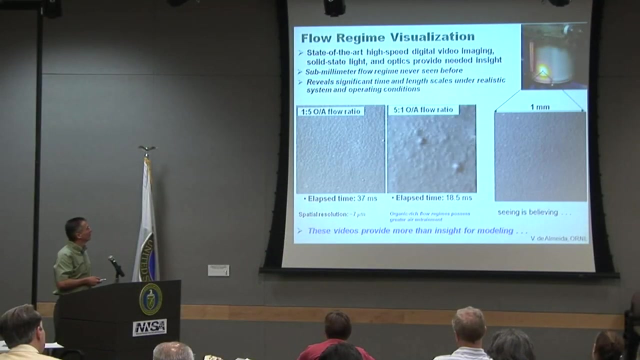 but what allows you to take these images is more the very fast shutter with a matched strobe light. Okay, And you know, to our knowledge, this is the first time this type of data has been seen, So these droplets are on the order of 10 nanometers in this case. 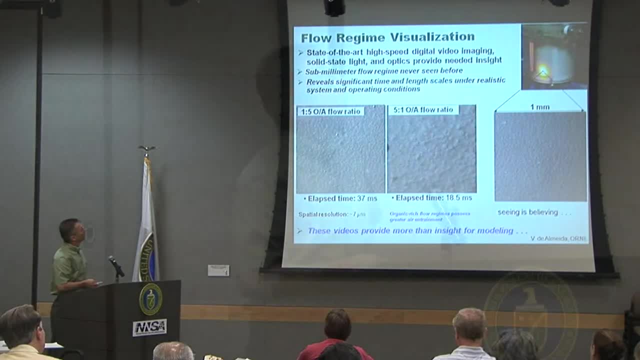 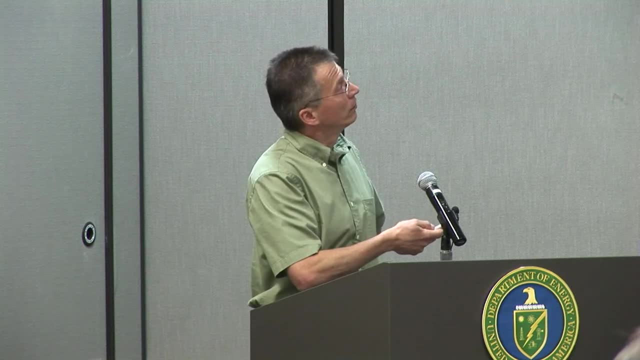 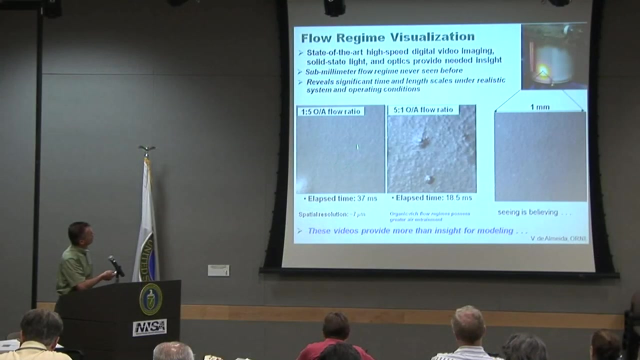 and they're zipping by at about 9 meters per second And you can see a big difference in the fluid flow that's going on Here. you've got on the order of 10 nanometer droplets, and this is organic droplets in an aqueous, continuous phase. 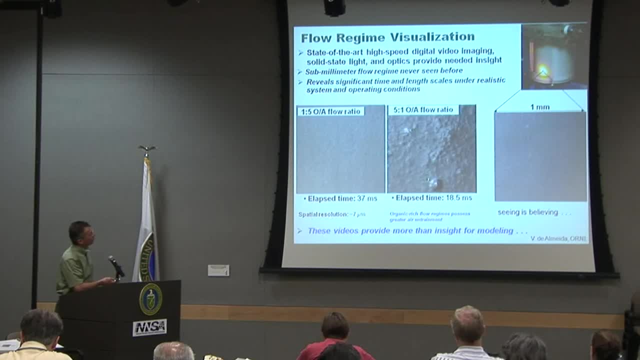 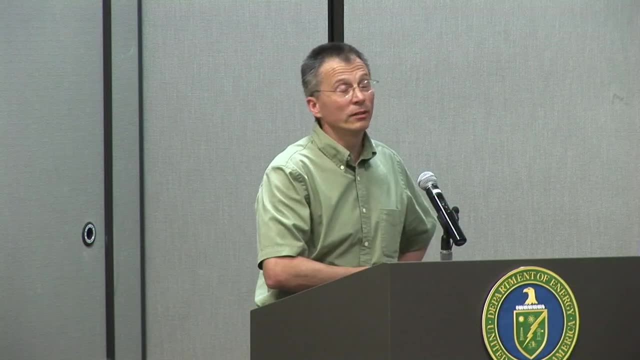 and over here is aqueous droplets in organic phase, but then you see these big round objects, and what those turn out to be is air bubbles. Okay, So you have entrained air bubbles. So this type of detail wasn't captured in that large-scale model? 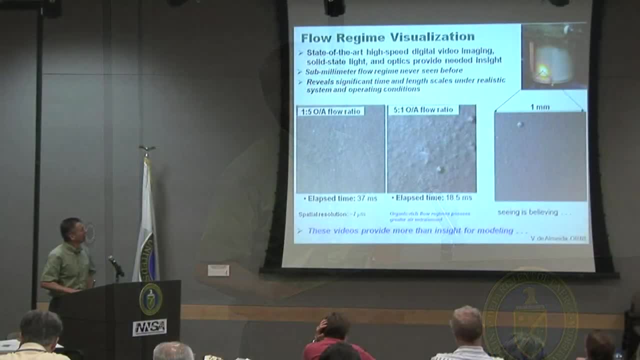 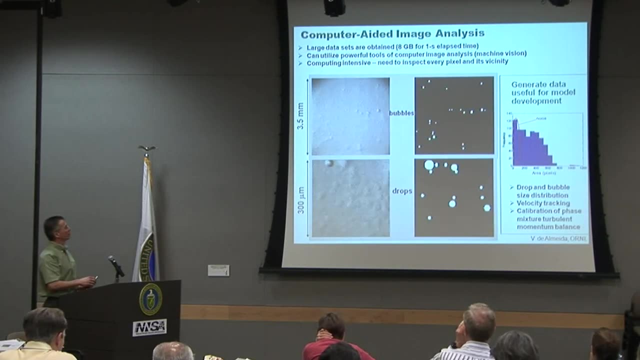 fluid dynamics model. so there's a lot more work to be done Now. the other thing you can do with these, this type of video imaging, is then use computer analysis of the images to then get you know, pick out the droplets. 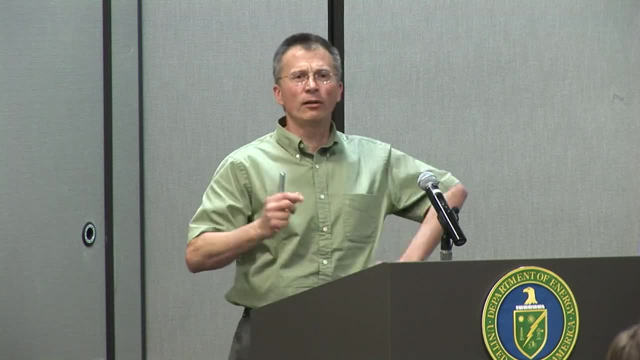 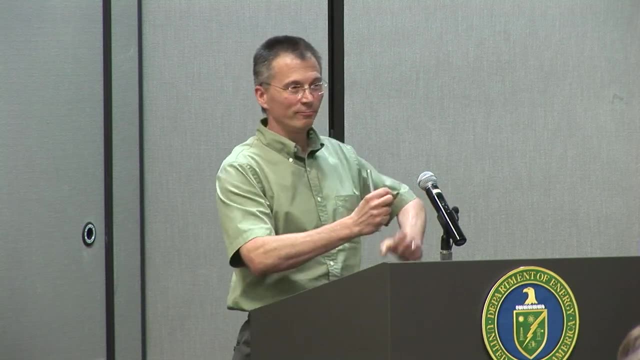 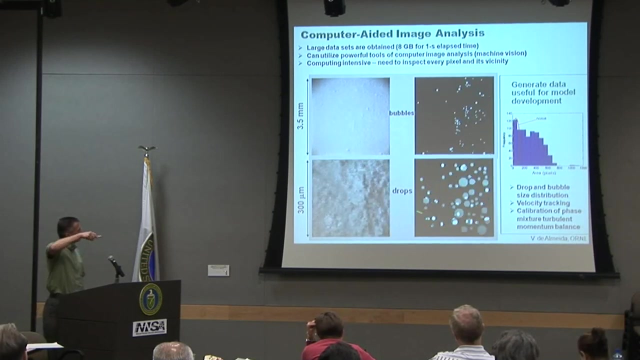 pick out the bubbles. here You can tell the bubbles because they have a higher contrast. So here is video and then here's the computer-aided- basically- extraction of the bubbles. Here is on the bottom, and I'm losing my pointer again. 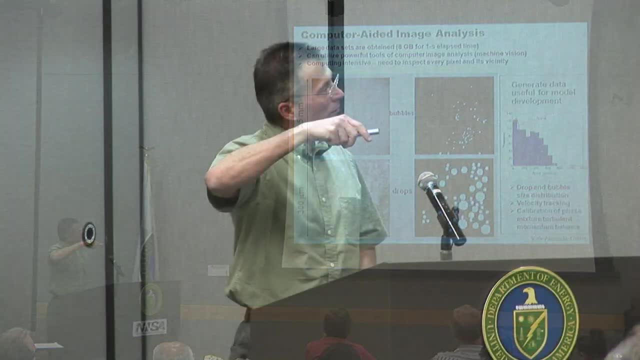 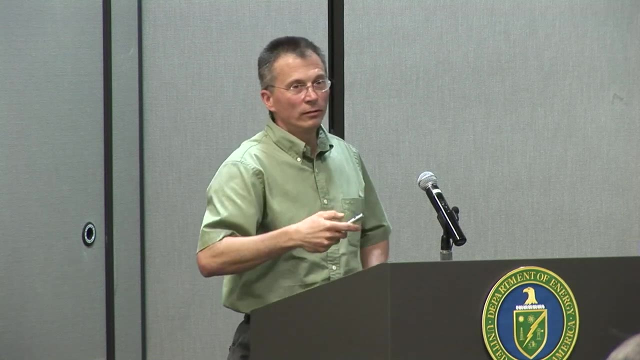 the droplets and then so you can see the matching frame. You can do the droplets, And what you can do here then is get a size distribution which then feeds a surface area. You can get an interfacial surface area and also allow velocity tracking. 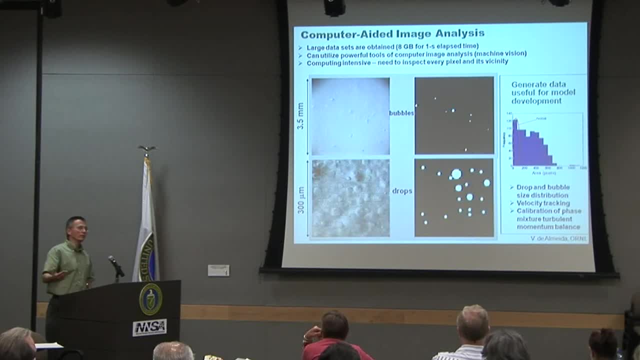 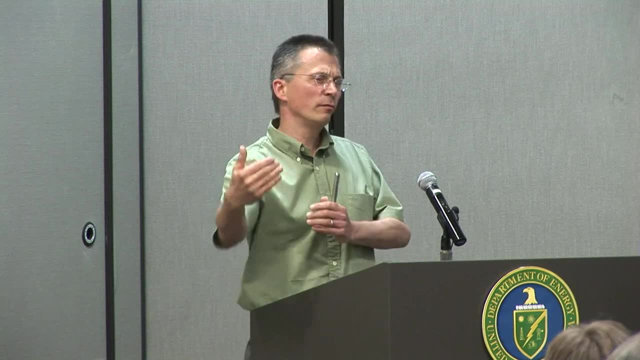 So this is an interesting approach. The issue there, of course, is you're only going to get the regime near the outer surface of the contactor And conceivably, I suppose you could do it from the inside and get the inside surface. 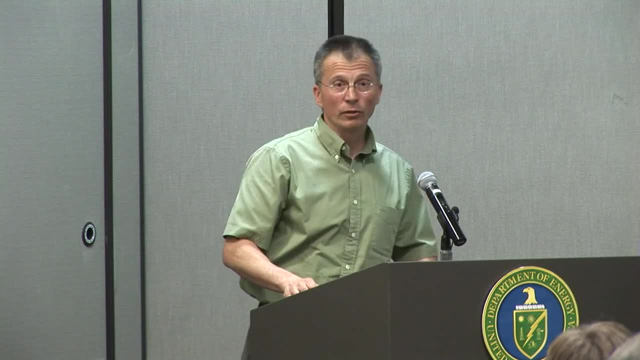 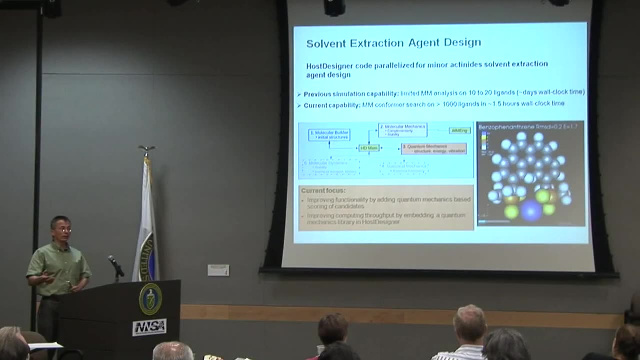 So it's going to be limited, but at least this is something again where you can really get some data that's good for validation. Okay, Recently, you know, I talked about what had been done in solvent extraction agent design. More recently, 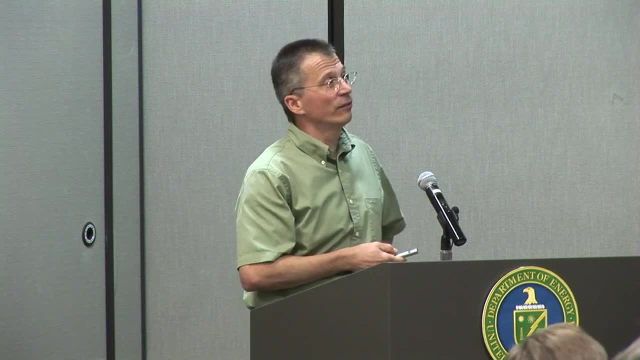 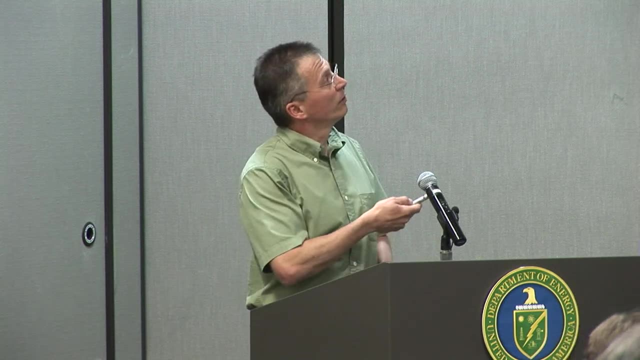 has been working with Ben Hay and he has parallelized the code that was used for agent design and so it's thousands of times faster. In the previous capability you could do a limited analysis. You could do about 10 to 20 ligands. 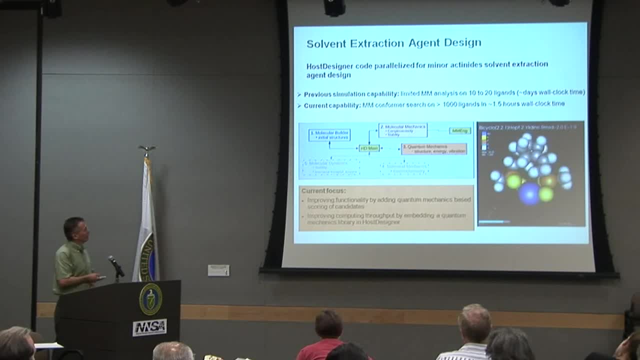 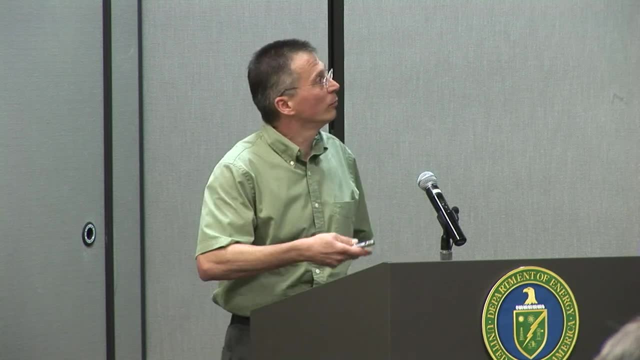 and it would take you days and turn that to a process where they can do 1,000 ligands in a minute And that's done in one and a half hours on a supercomputer. So you can crank through a bunch more molecules. 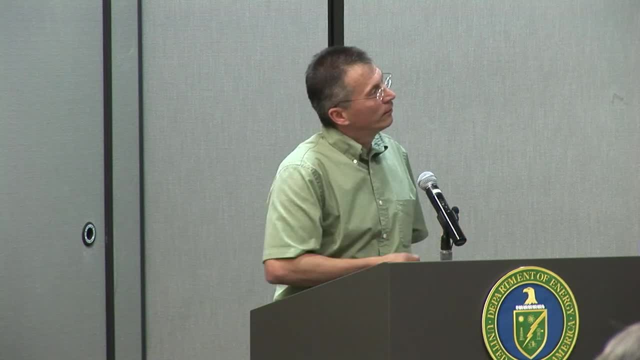 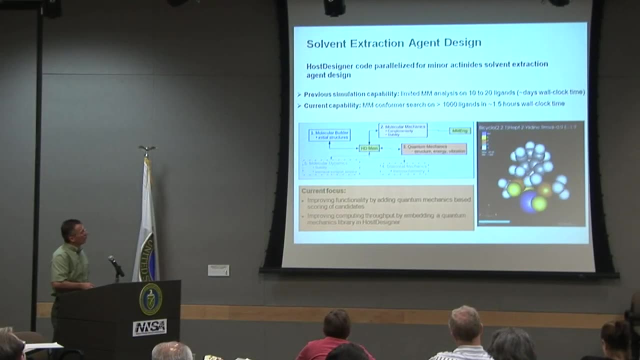 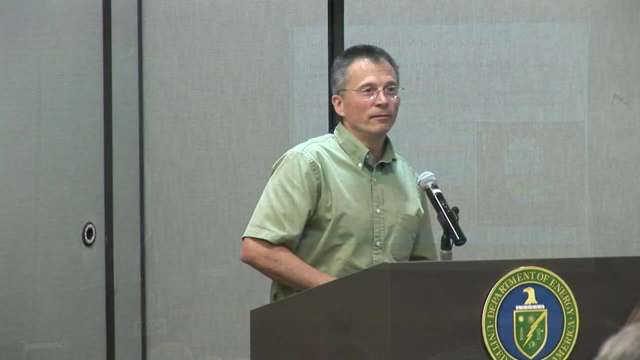 Now they say that these are the top five molecules for americium that they've found so far, And so okay, so you can see them. What's interesting is then they went and synthesized some of these, and the top scoring one were very susceptible to hydrolysis. 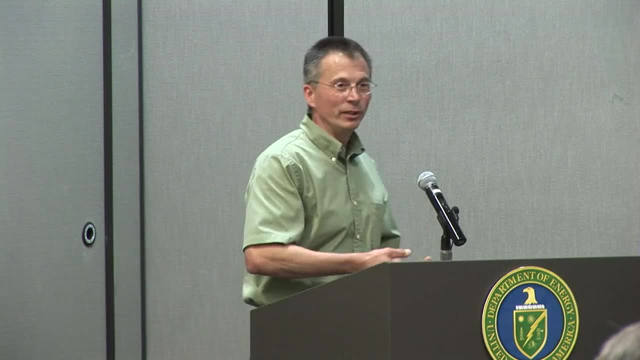 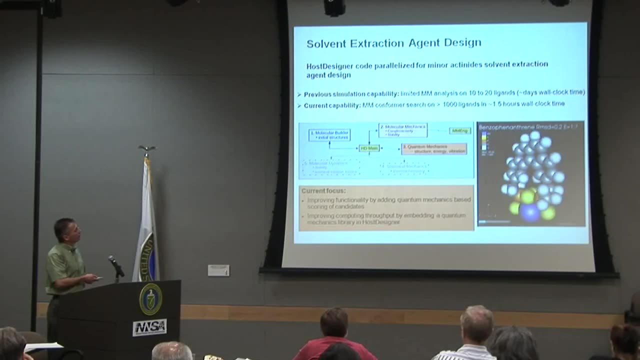 So even though they score well in the computer, when you go try them out first, experiment says: oh, this is no good, Let's go back to the drawing board, Okay, so where are we on this? It's basically adding quantum mechanics. 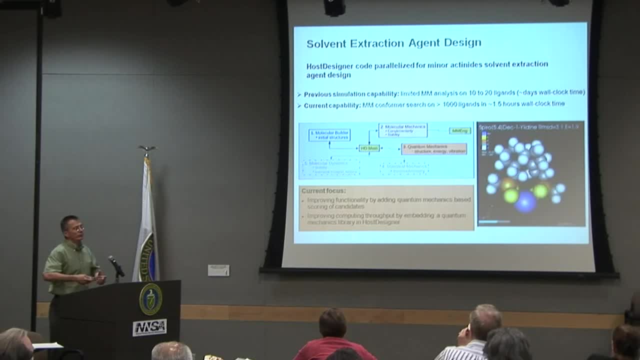 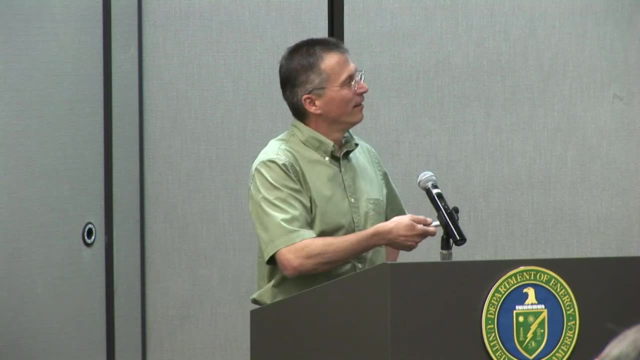 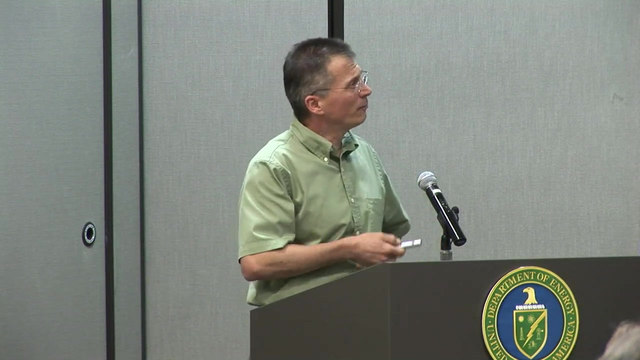 And so using quantum mechanics will improve the scoring, and there's an awful lot of computational work that has to be done to connect this host designer program to existing quantum mechanics codes. But then the next step is moving along. These are these empty boxes. 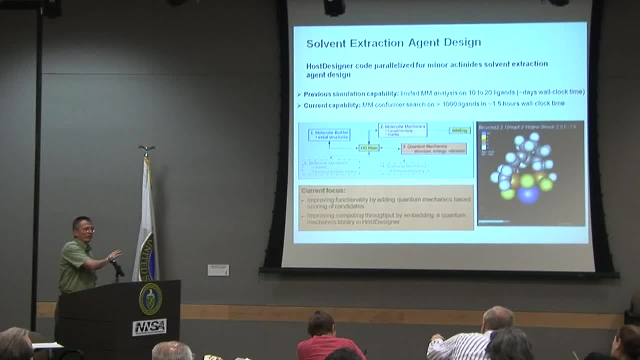 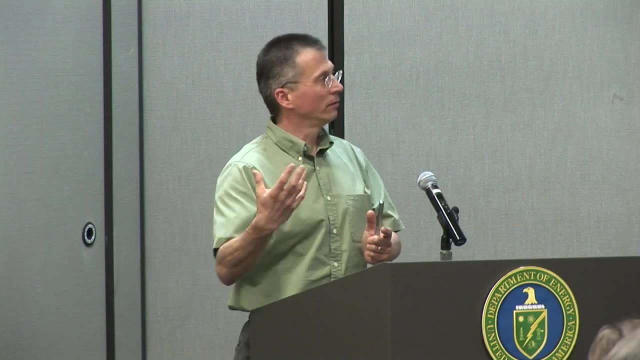 Here is all these things are taking place in a vacuum. okay, Now to really be predictive, what you have to do is take these molecules and put them in a solvent and then actually have the interactions with the solvents in the other species. 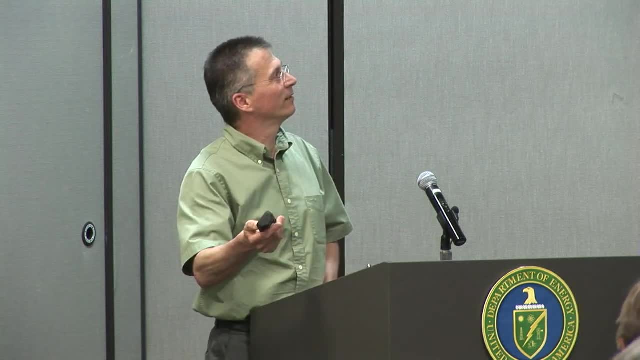 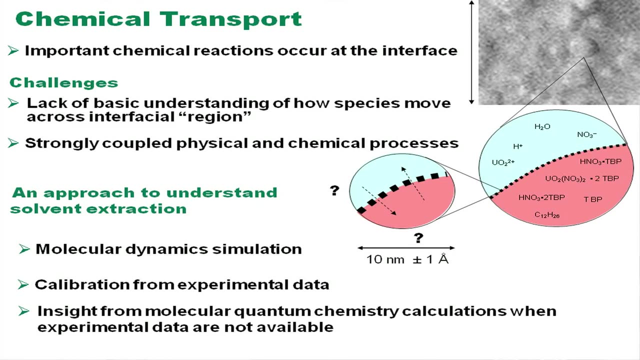 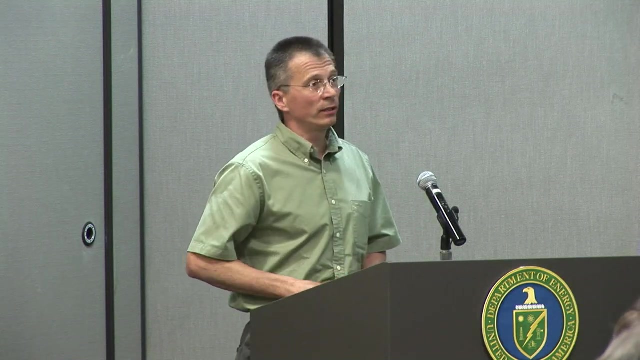 But that's a frontier That's not happening right now. Okay, so now if we look at what is happening at the interfaces, what are happening with the molecules, you can see. you can use molecular dynamics to get some clues. Try to understand what's happening. 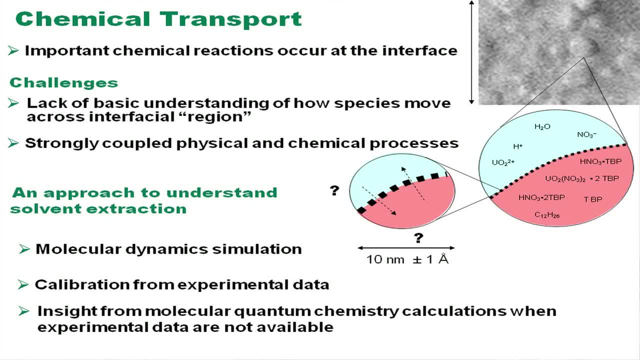 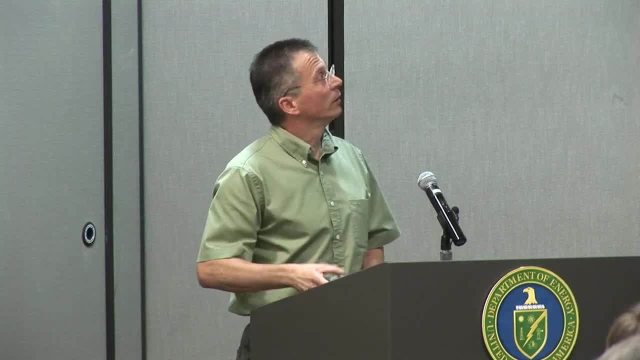 You know we do not have. we've been doing solvent extraction for years and years and years, but we really don't know what's happening at the molecular level. We have good ideas, but we don't know fully. So here's some work that's been going on. 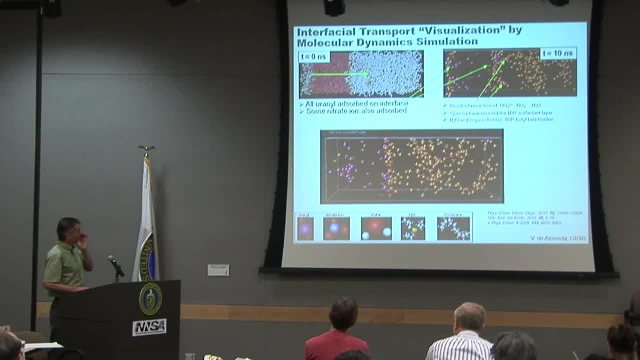 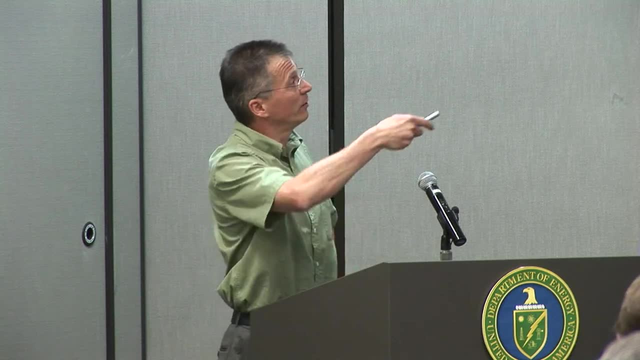 looking at molecular dynamics of a solvent extraction, And so I think I have a blow-up of this video on the next slide so I won't spend too much time trying to get you to see this. But basically, what you're seeing on these slides are: 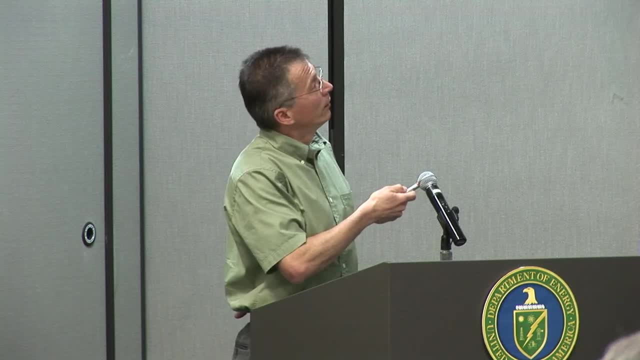 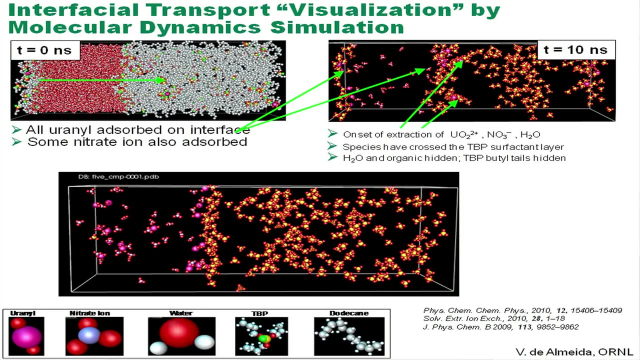 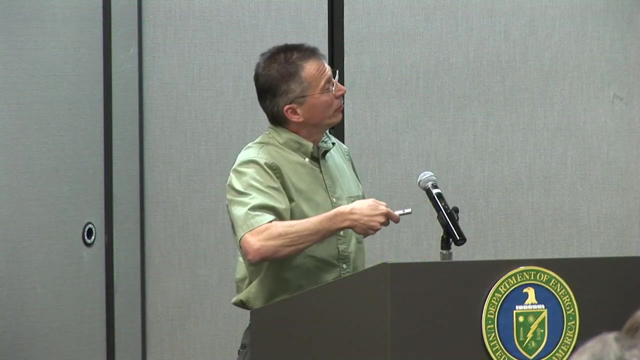 kind of a preliminary calculation. but what you've got is a water phase here and then an organic phase. This is tributyphosphate and dodecane. So it's, you know, it's a typical solvent And we're looking at uranyl nitrate extraction. 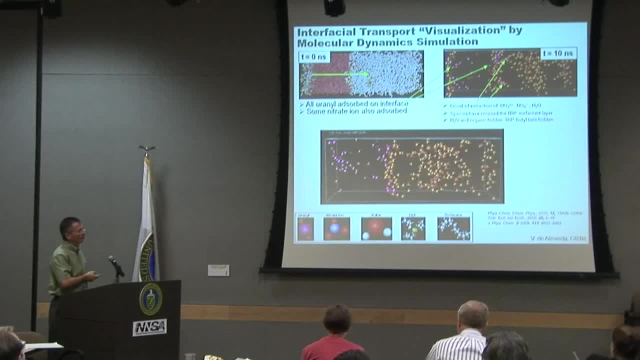 So the magenta, the big magenta atoms are uranium, Okay, And so in this, in this simulation, you're seeing all the atoms, And then down here we've taken all the organic tails off so you can actually see the phosphate groups. 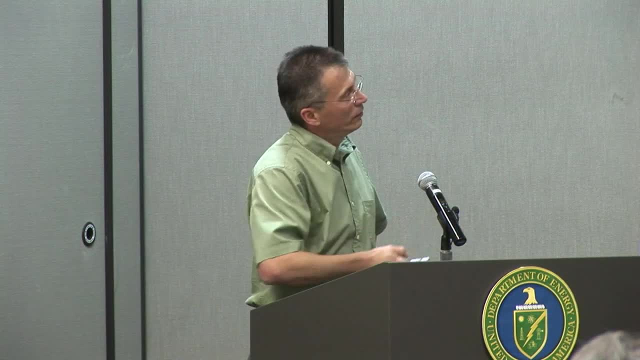 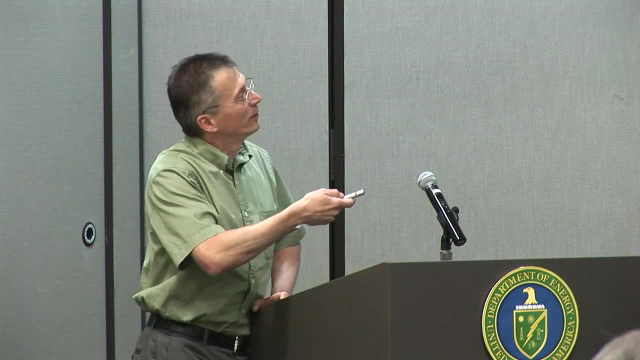 on the tributyphosphate. You can see the nitric acid and you can see the uranium And what. well, if you know what to look for, I suppose what you'll see is that the uranyl are going to come to the interface. 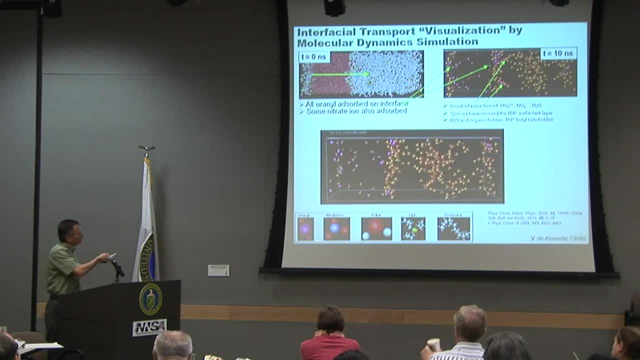 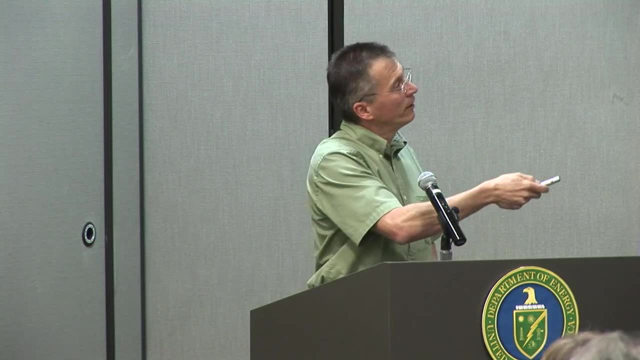 between the organic and the aqueous. The other thing that you'll see is the tributyphosphate. Right in here you see all these yellow dots. There's an awful lot of yellow dots right at the interface, and then you don't. 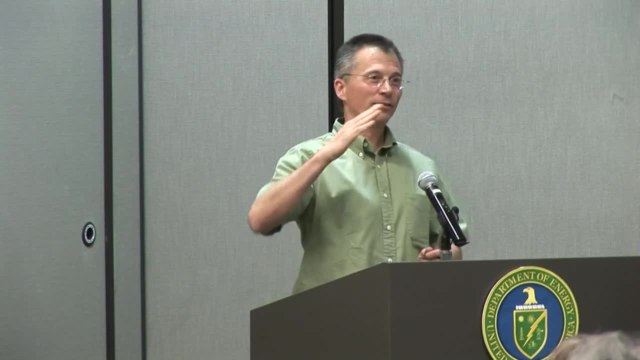 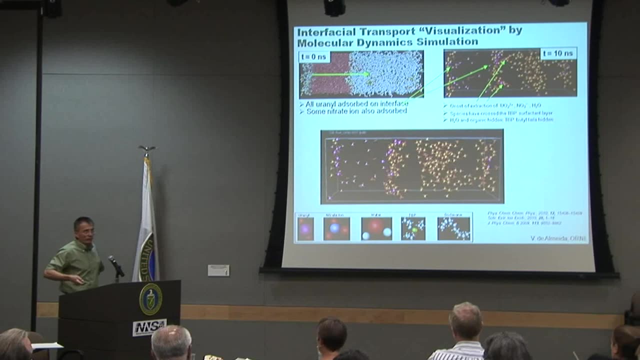 you see this kind of vacuum right here And that's the, the solvents lining up with their polar groups at the, at the interface, and then their organic tails sticking out. Which kind of surfactant behavior, and I guess you'd. 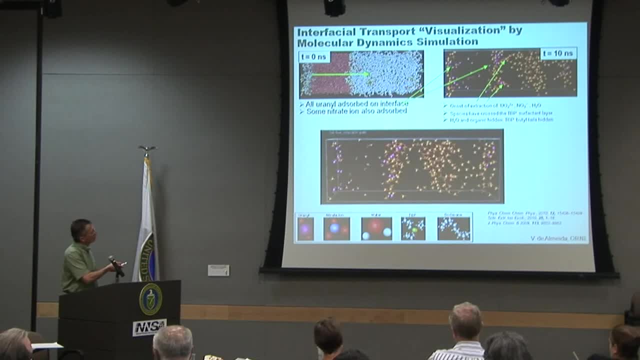 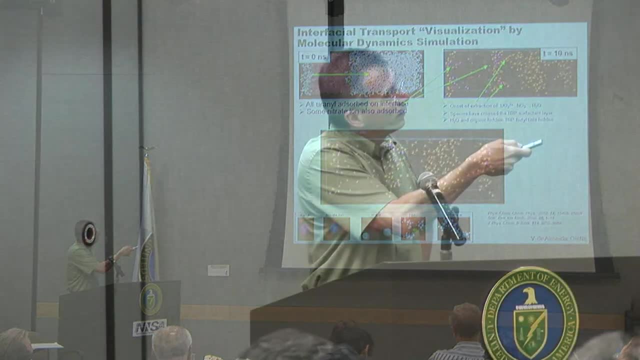 you'd expect that. Now, what's kind of interesting is, as this goes on, what you see is that these tributyphosphate, these tributyphosphate head groups are having a heck of a time grabbing. and I can, you can see it right in here. 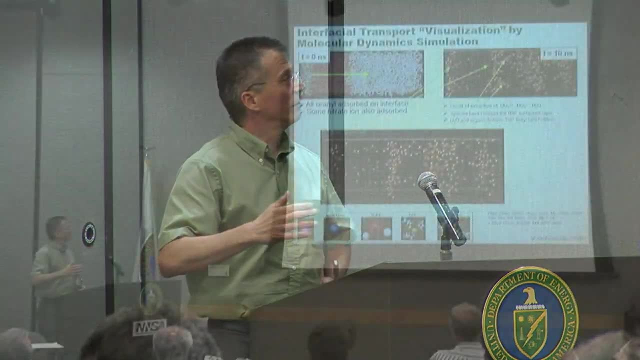 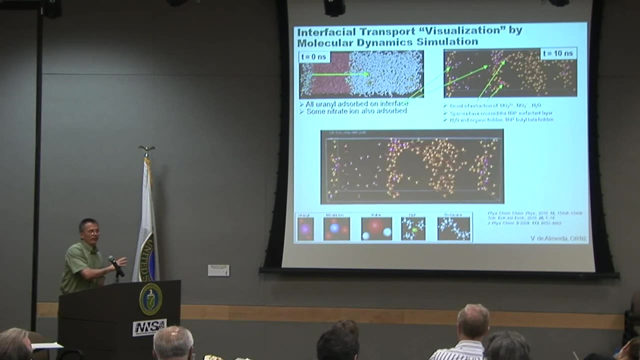 You can see they have a heck of a time pulling them across that kind of vacuum until you see they can kind of bridge and then they pull it across. And so certainly this is not, this obviously has not been a fully calibrated model. 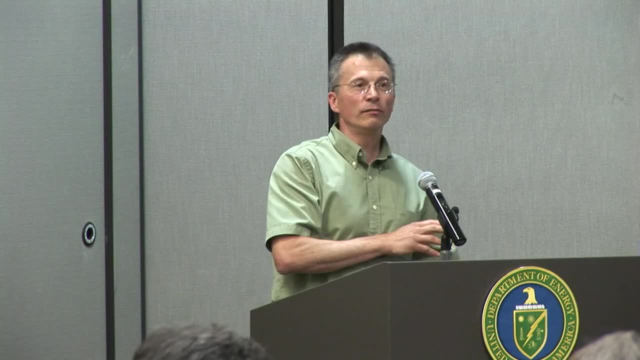 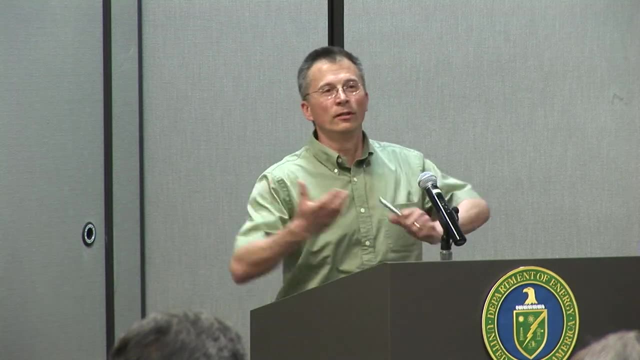 and so it's. it's not fully predictive, but what it does do is give you some sort of insight. This could give a solvent designer some sort of insight of aha. maybe I need to make these things bridge across this, this organic, rich layer. 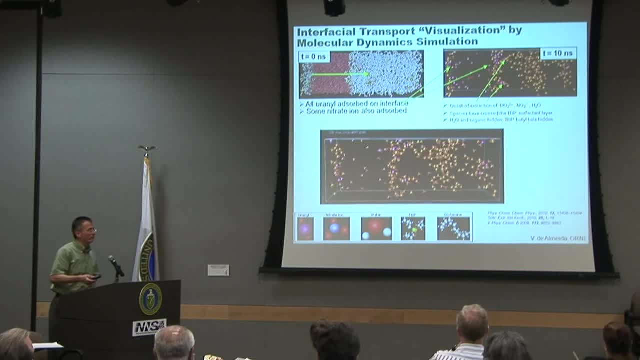 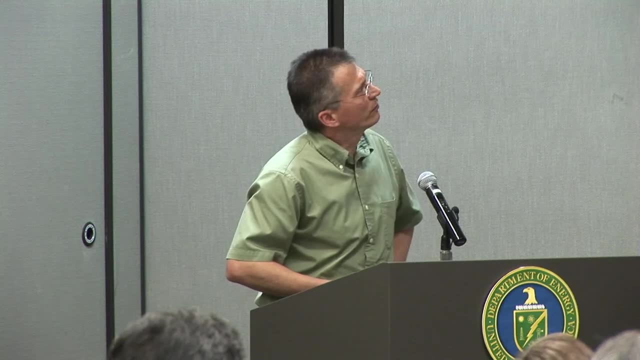 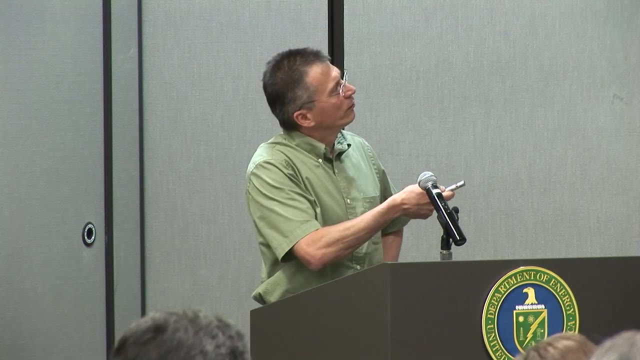 or maybe I need to change my solvent so I don't have that barrier, And so this is a little. this will blow up a little bit more of the same simulation And so basically I guess right in here was where that, where that action was. 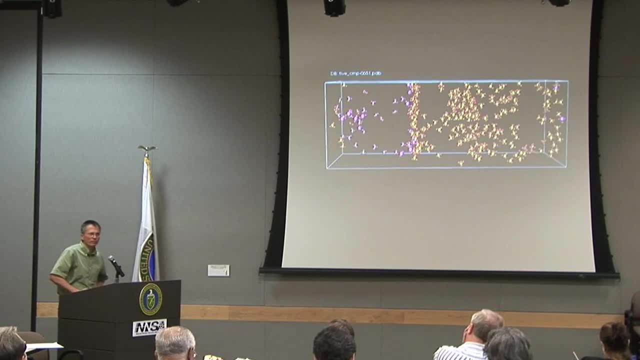 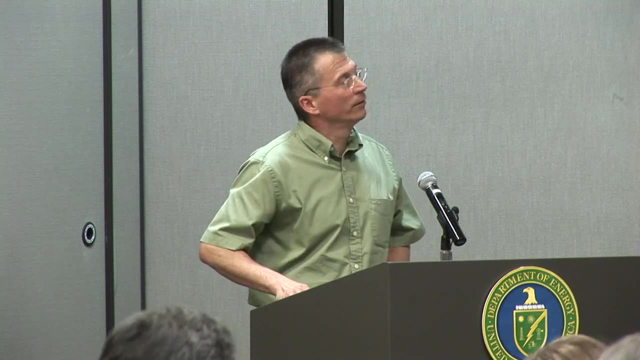 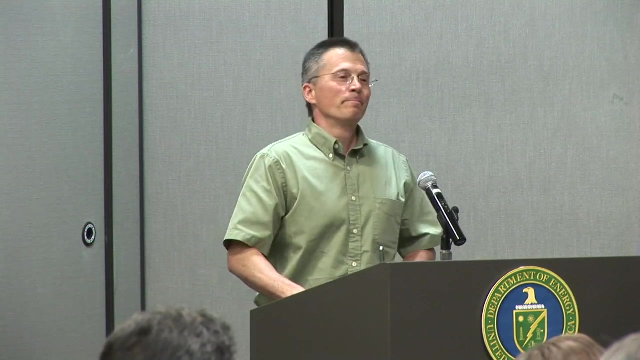 But these. this is a very large simulation, I think 18,000 molecules in this and this is, you know, several days of supercomputer time to do picoseconds of reality time. So the prospects of being able to say: 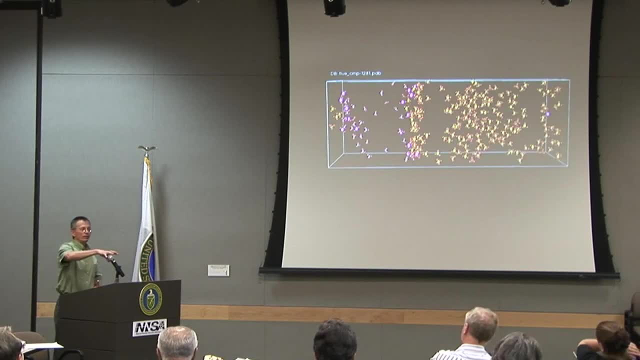 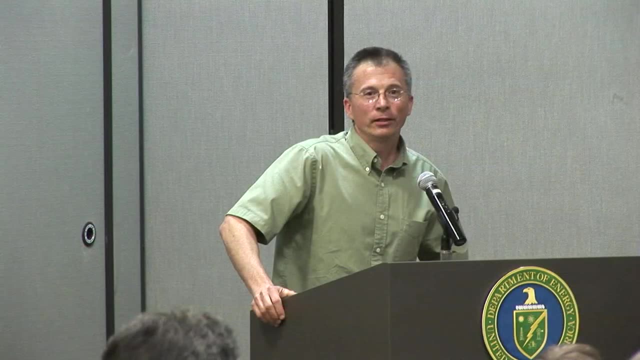 computer, throw all these molecules in a in a box and tell me what's going to happen in this entire reprocessing plant. Okay, that's well not in most of our lifetimes is that going to happen? So it's. 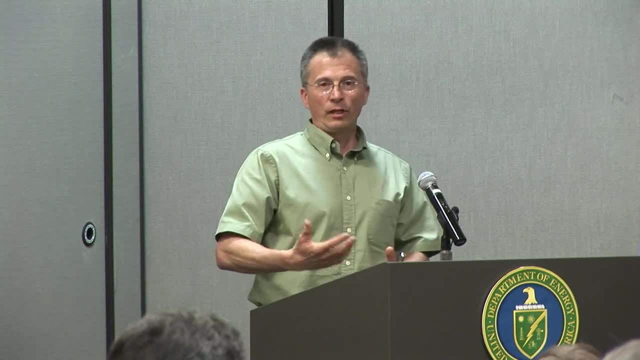 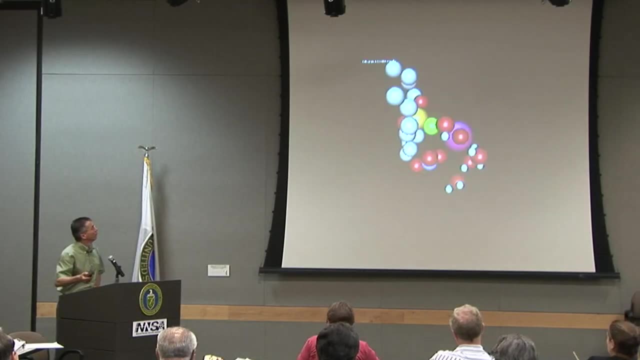 it's really. can these models give us insight that allow us to accelerate? what we're going to do experimentally, I think, is where the, where the value is All right and it's well anyway. so this is just showing the. 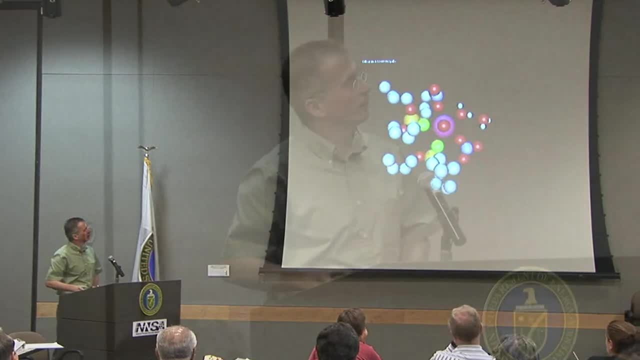 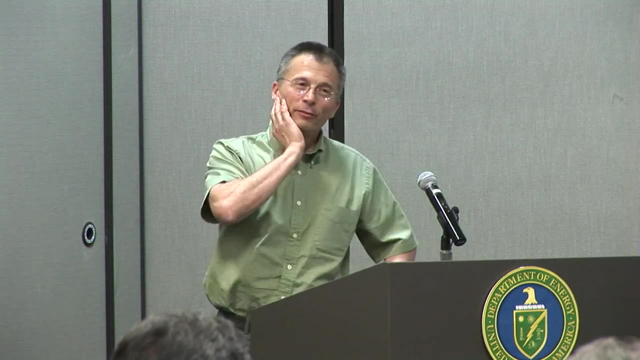 it's showing one of those uranyls and how it's being coordinated through the through the time steps. I'm not going to spend time on that, Okay. so where is this going forward? I remember the last time we gave this course. 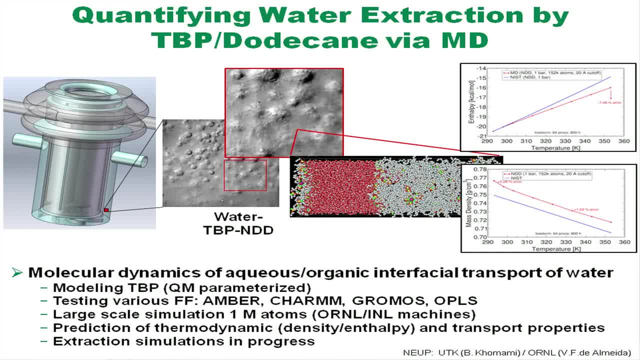 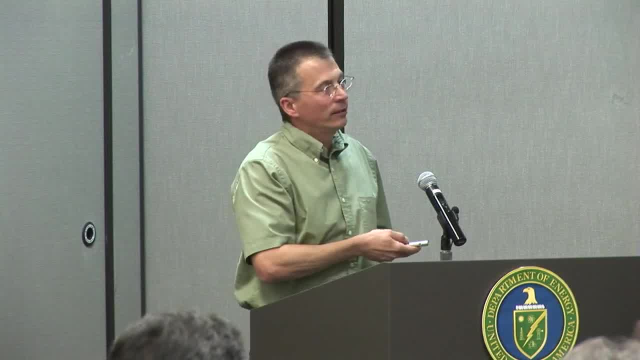 Gordon Jarvin and said: well, heck, that's a really complicated system. Why don't you do something more simple And absolutely right, Okay, Okay, so what the this in a any university programs project? and so this is: 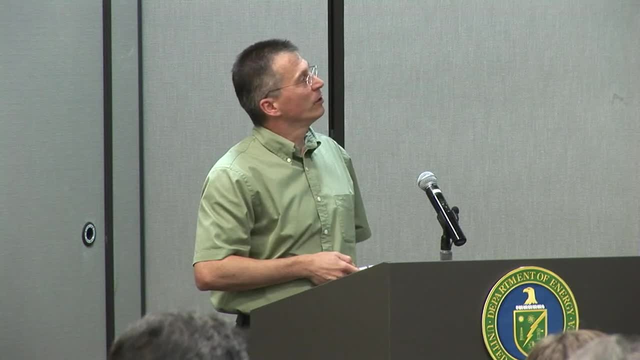 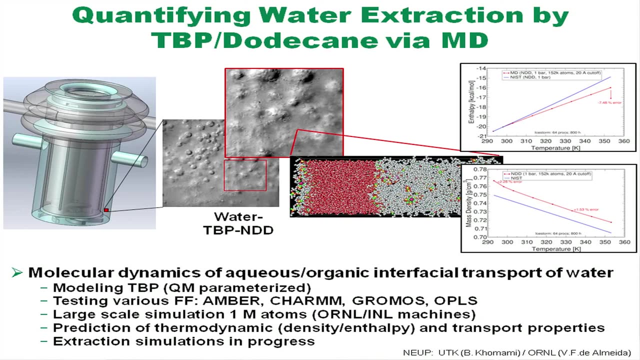 and and collaborating. What they've been doing is taking that same system and making it a whole lot simpler. So we're just looking at water extraction, Okay, but, but the point of their work is to look at the force fields that are used. 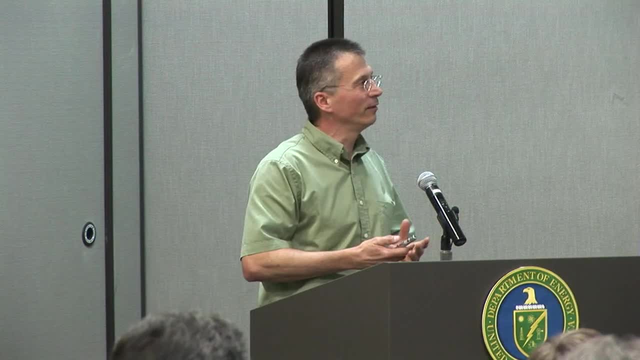 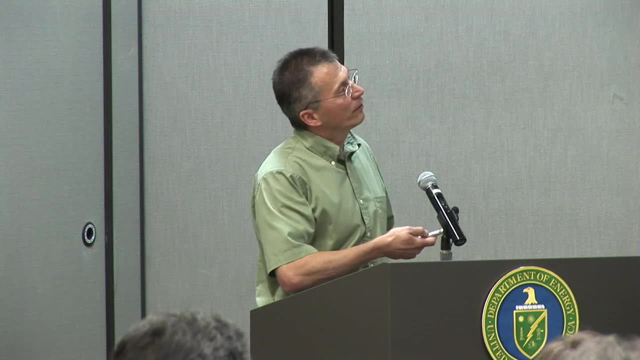 So use a bunch of force fields that are out there in the literature and try to calibrate them or use the best ones, such that they can actually reproduce some results, And so over here you can't see too much of it, but here's a density: results in. 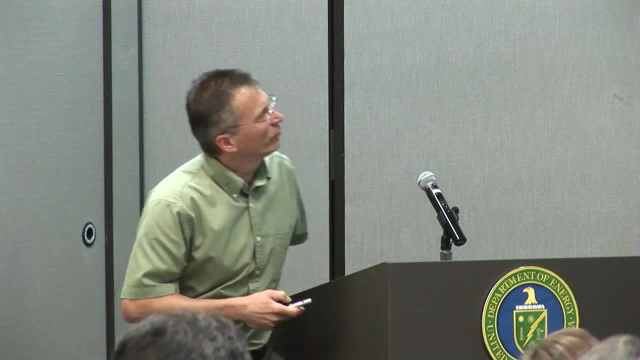 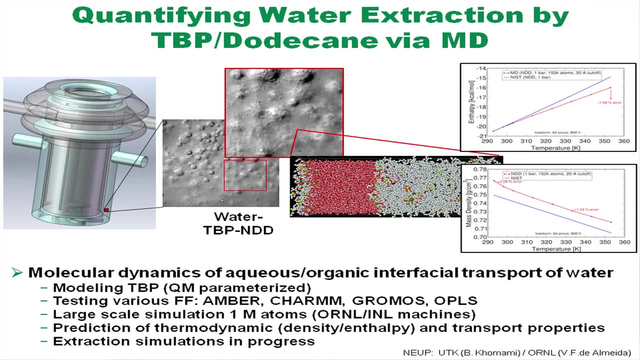 gee, I can't even see how close it is, But they're within a few percent on density, Okay, so that's all right. And then I just saw a paper that they're preparing. where they're, they did a diffusion coefficient. 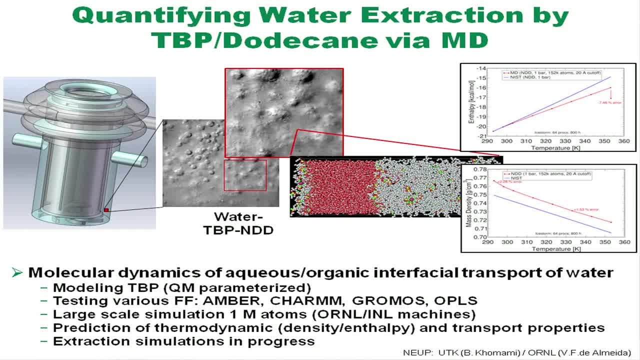 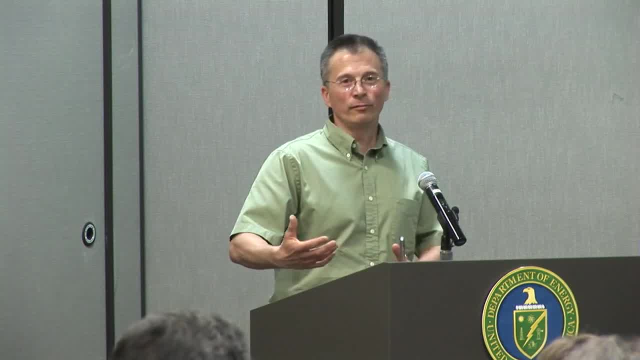 and they're within 20% on a diffusion coefficient. So not great, but at least now we're providing some calibration. How good are these models And what do we have to do to change the, to get better models And what it comes down to? 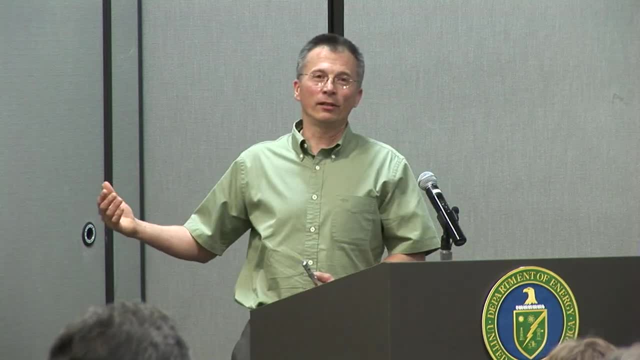 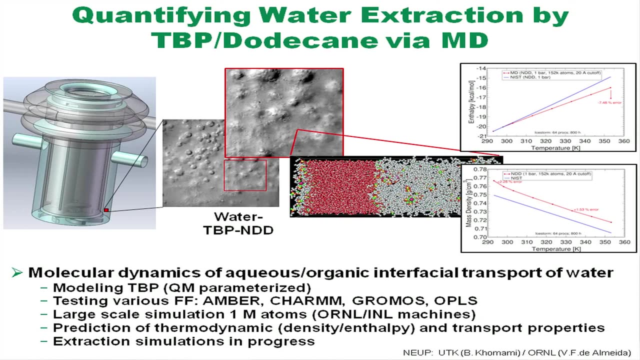 is these force fields. So remember when I said previously, it all comes down to somewhere. you've got an approximation or an empiricism or something, And so you've changed: where's the approximation? The approximation right now is in these force fields. 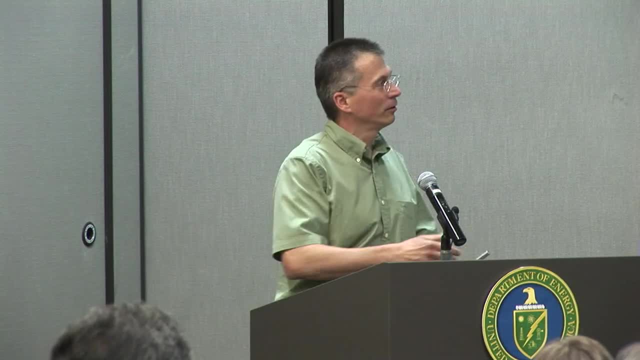 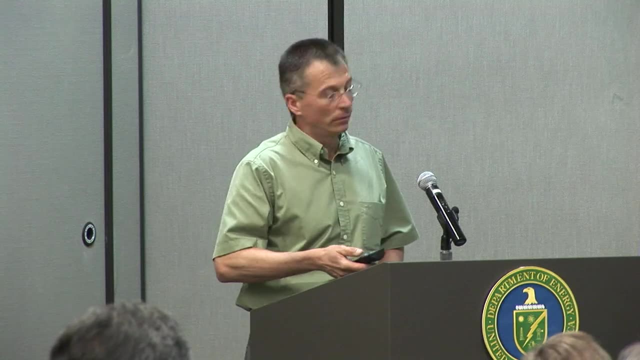 Unless you want to do a full quantum calculation to get everything you know. you're basically you. what force fields are you going to use to to do these predictions? But you know, good progress, actually Another university program project. 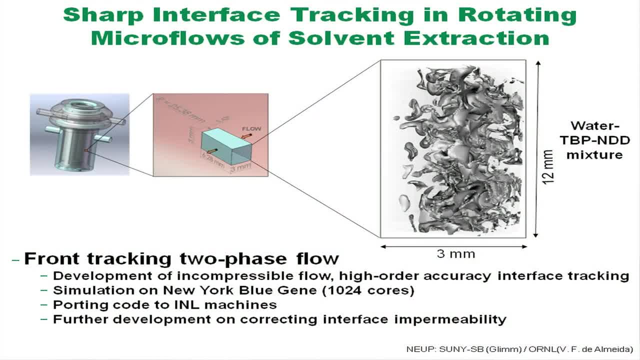 when I had said that they're having problems resolving the small droplets in the centrifugal contactor model. Well, here's some work that's being done by Jim Glimm of SUNY Stony Brook, and that was Velmar Diomedo. 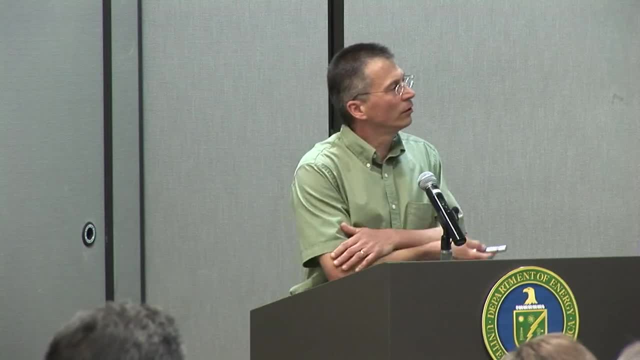 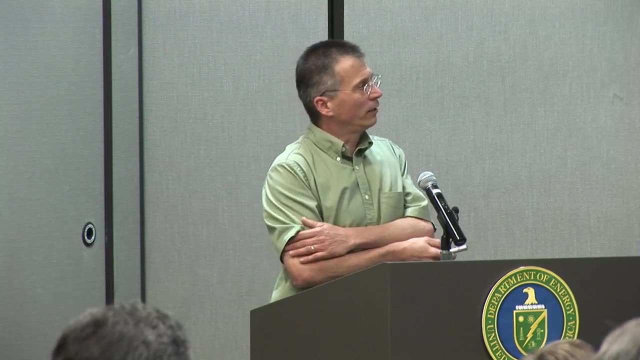 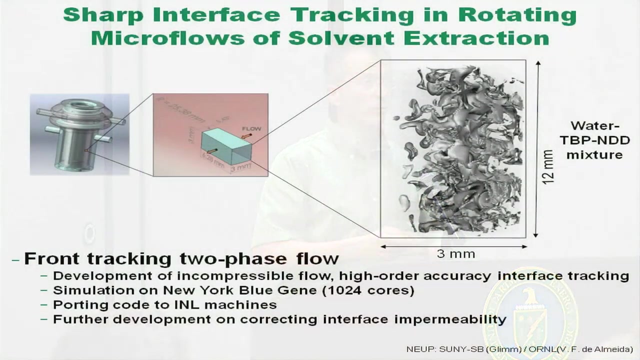 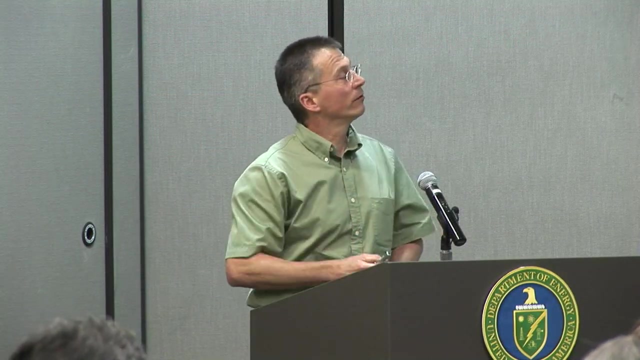 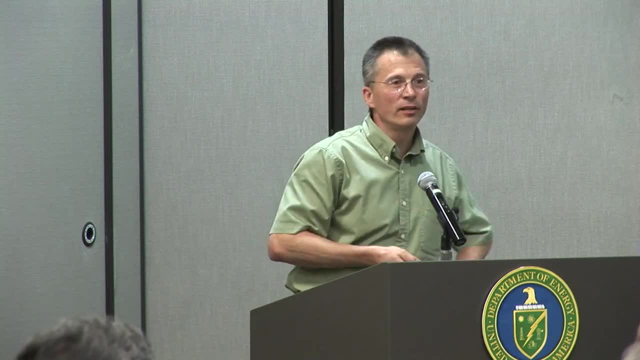 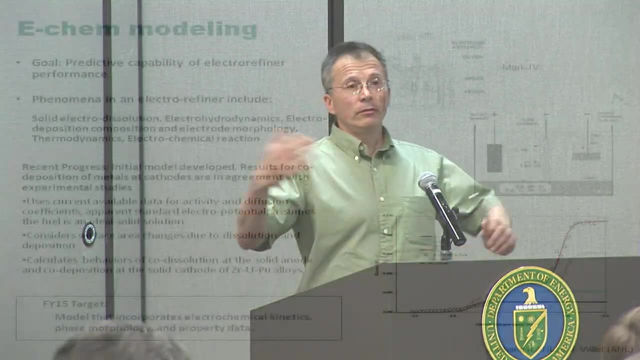 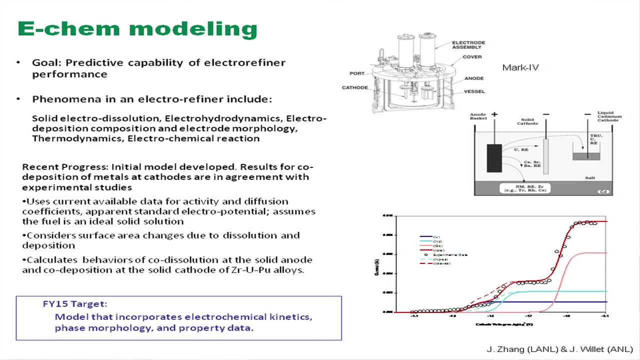 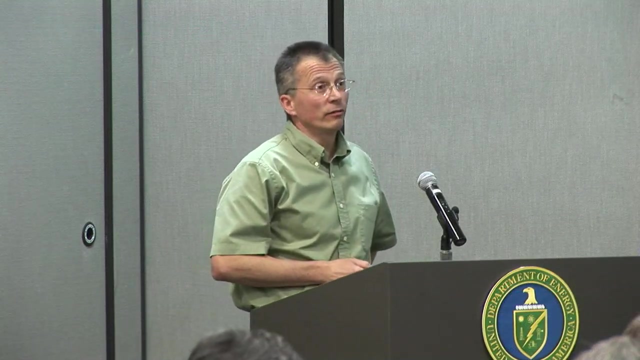 here is it, it it has and hopefully applicable as we move along. okay, completely different topic, but we heard this morning about electrochemical processing and so we do have some work going on in modeling of electrochemical processes. an electro refinery can imagine there's multiple processes going on. 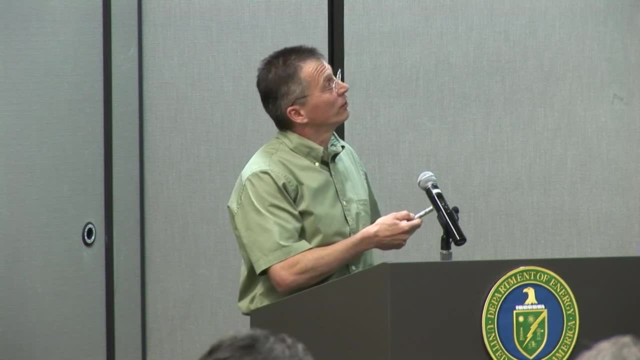 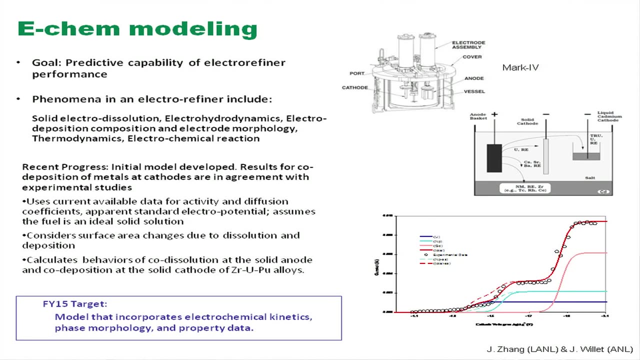 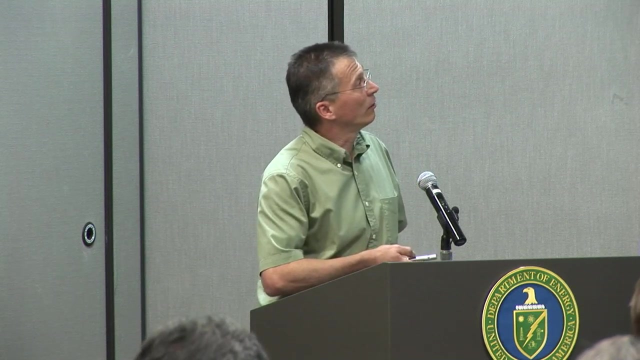 there you've got electro dissolution, you've got electro hydrodynamics, electro deposition, composition, electrode morphology, thermodynamics, electrochemical reactions- all this going on in this, in this complex molten salt environment. okay, so Jin Su Zhang and Jim Willett of Los Alamos and Argonne are working on developing a model for these electro refiners and basically they're. 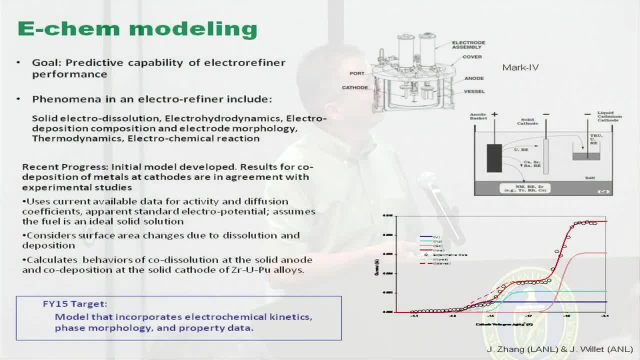 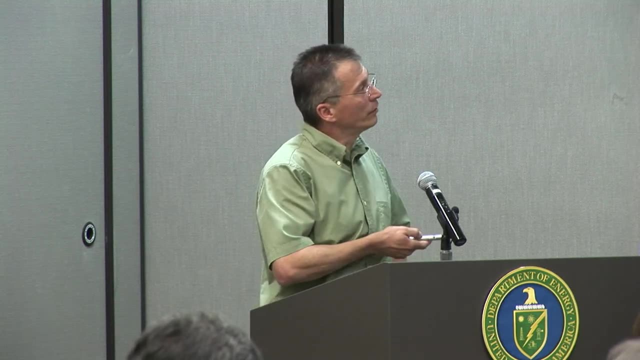 trying to take into account each of these things and so far they've been looking at, they've been using available data on the activity and diffusion coefficient, assuming that their deposit acts as a, as a ideal solid solution, and what they've been showing is that they can get co-deposition at the solid cathode we heard. 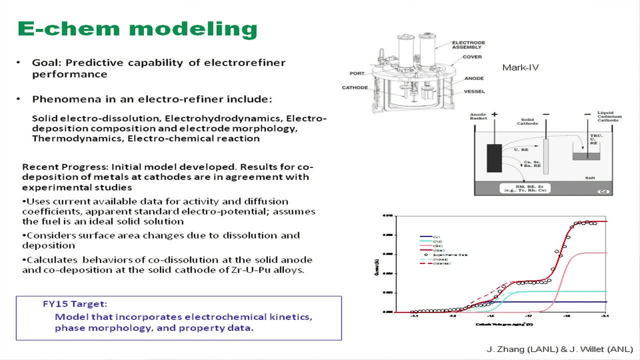 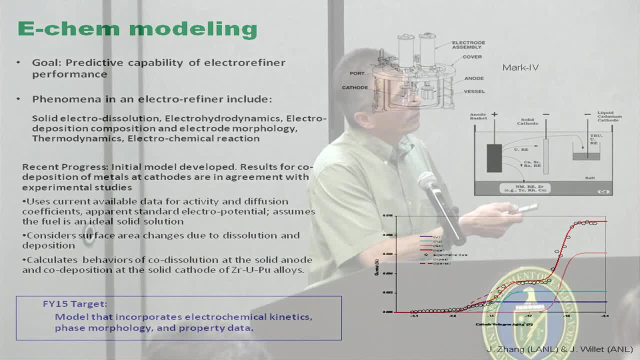 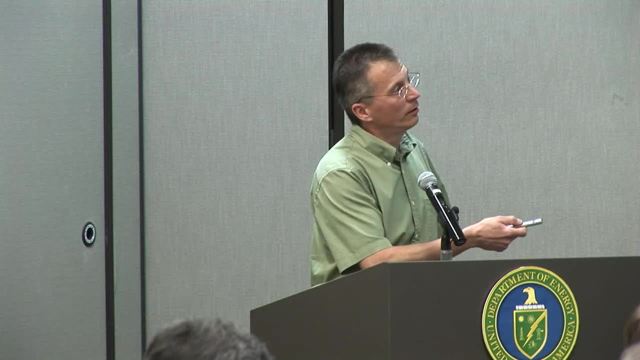 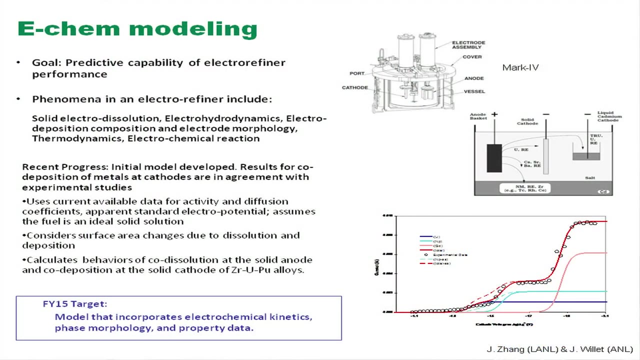 this earlier earlier this morning about these co-depositions. so here they're doing zirconium, uranium, plutonium alloys and the dots. here are actual experimental data and then you can see the contributions of the different zirconium, uranium, plutonium, different curves and they add up the added. here y-axis is current and this is applied Potential and 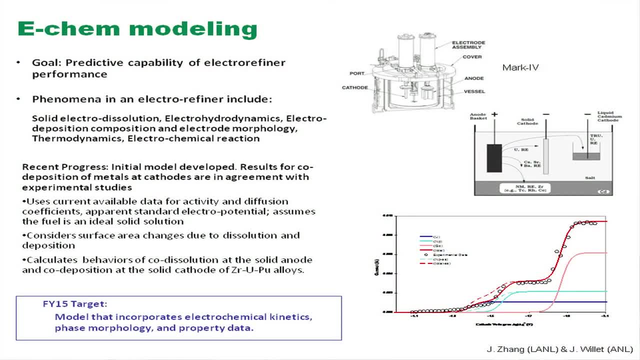 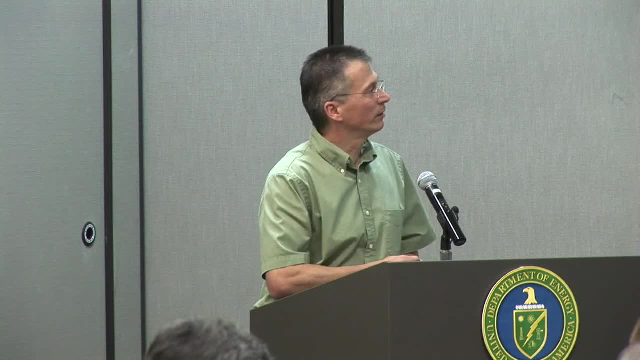 you can see it, it matches relatively well. so they're they're on the right track, but obviously, there, this is only preliminary work, and so their target by 2015 is to have the, the Kinetics of phase morphology and full property data into this, into this model. okay, a couple of slides on work that's going on here. I know it's super often about this, but it's also about looking at the product as such. that someone just looked up you see if it's been onions in longer or it's not convicted, but you see if it's fine if it's went from realised or grab it. so all type type, all that amount of information that would be passes in, that should be Мос independently. so cups ande zero. so your standard, unique learning. you can use least part, no interest, as supplements. you can put in course a certain number of В, the initial number. so at Y is the main. 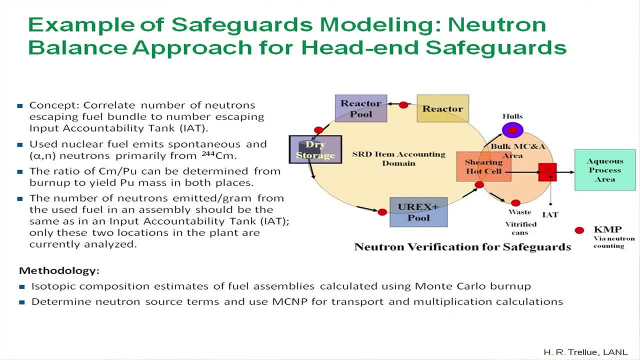 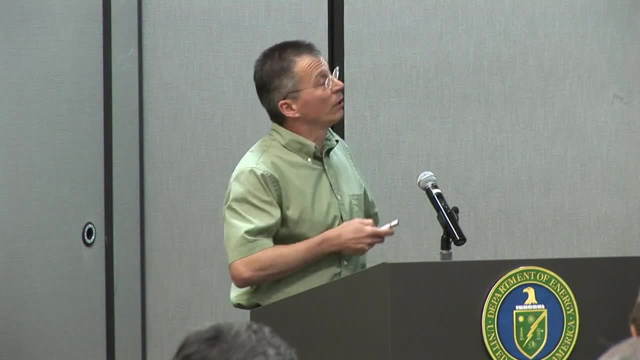 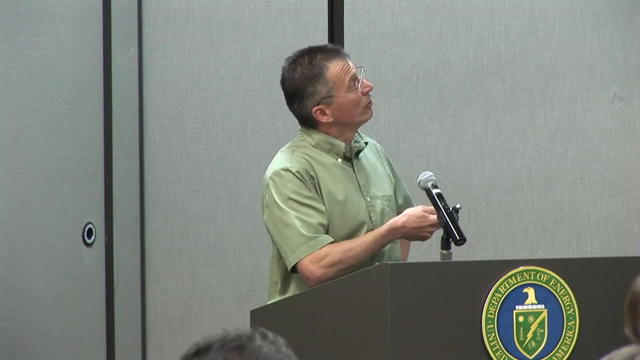 work that's going on in modeling of safeguards. One approach that's being considered to basically connect up with this plant-level model is this neutron balance approach for the head-end safeguards, And the idea here is you can measure the neutrons from curium and then, if you 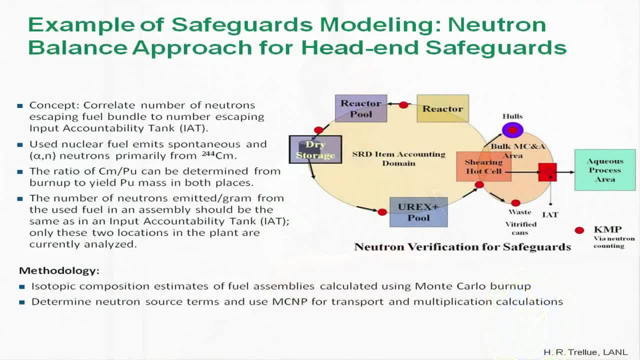 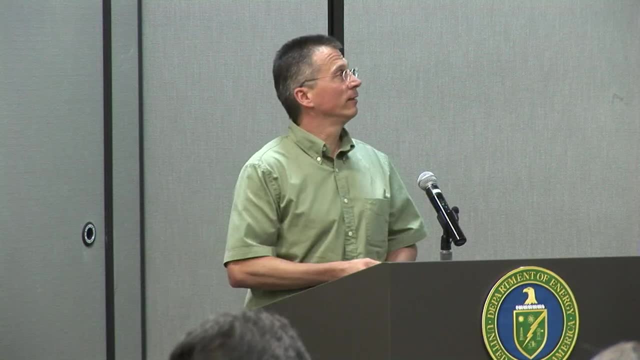 know the burn-up, you can then ratio the curium and plutonium. So if you know the concentrations at different – you know the ratios at different parts of the plant. you can actually use neutron transport calculations then to see what your instruments would actually – predict what. 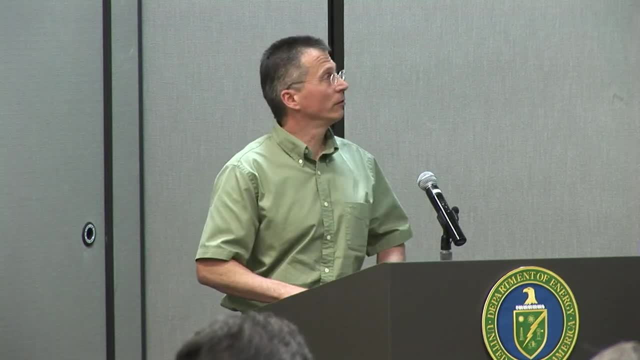 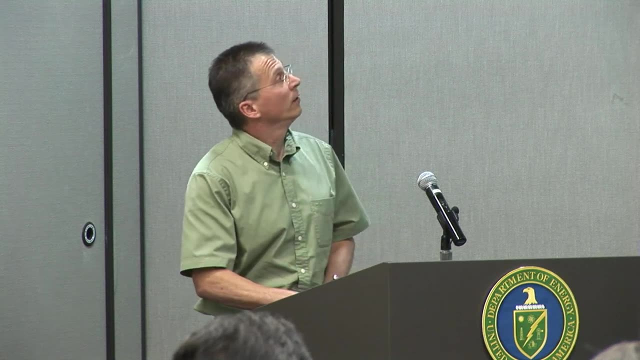 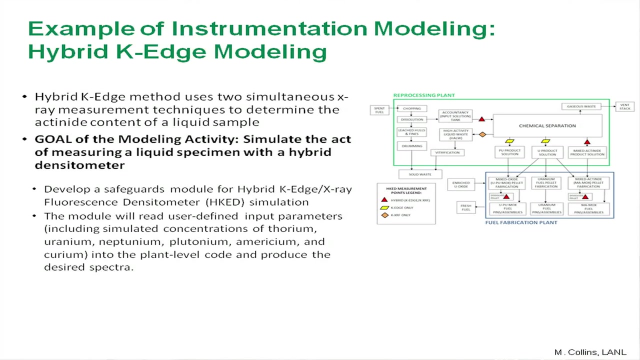 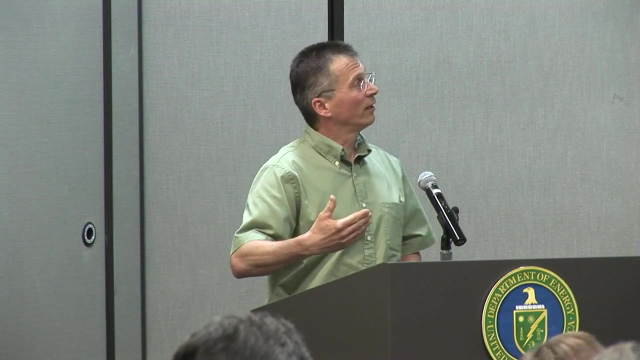 your instruments will be seeing, and what does that mean in terms of a safeguards calculation? And then the other instrumentation modeling is hybrid K-edge modeling And basically here is using simultaneous X-ray analysis and basically deconvoluting the spectrum that you get out of it to then say what are my concentrations of my actinides? And so then the idea is here: 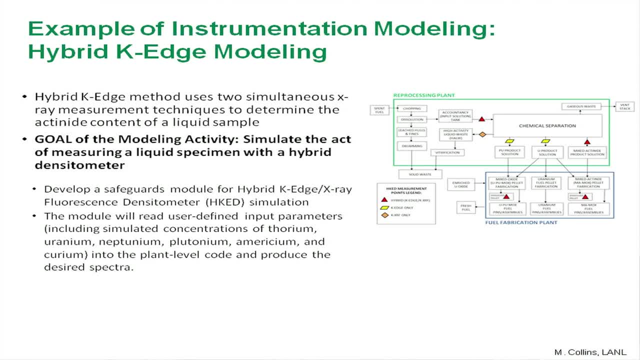 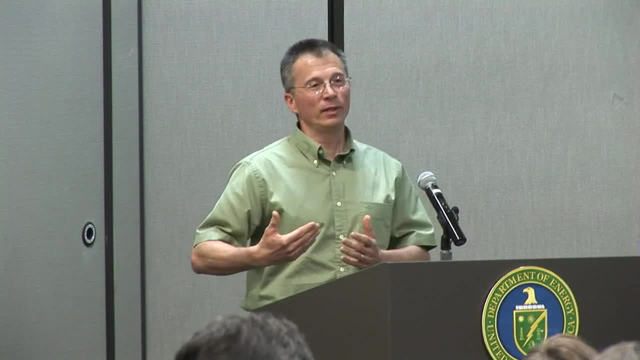 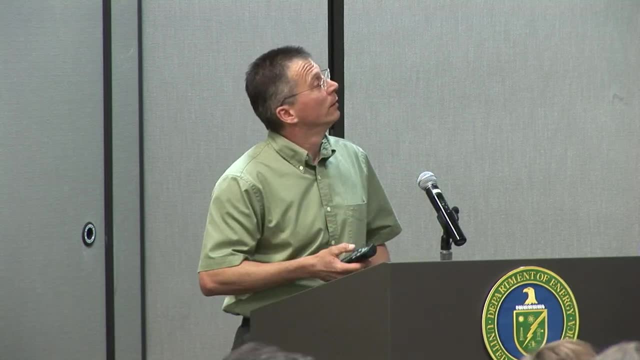 is. could you then take this plant-level model? you know the compositions that are there. then you could say: here's what my hybrid K-edge would see: How good is my –, how good is my measurement. And then one last topic here, and this is kind of way out there, but the idea that okay. 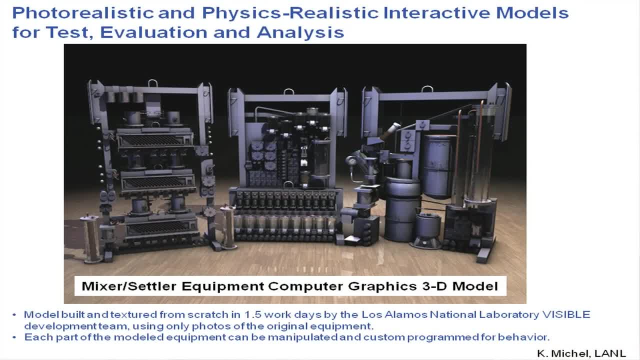 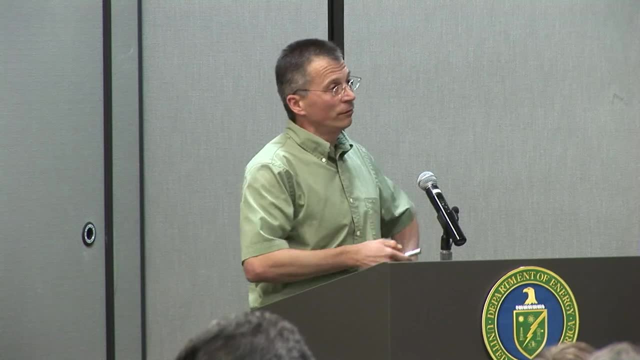 we have these process models, but we also – the entertainment industry has been doing wonderful things with visualization. Okay, so you can do real – photorealistic, graphical representations of these things, So you can really visualize what's going on. Here's some stills of a. 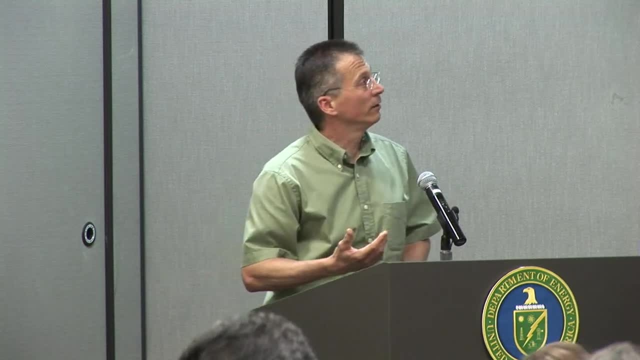 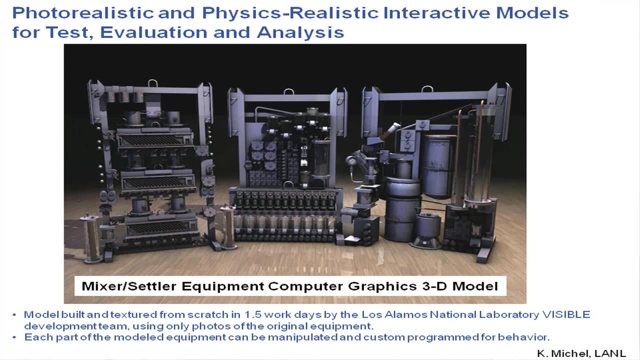 a fully 3D representation of the mixer settlers at the REDC at Oak Ridge, and this was done by Los Alamos team, basically just took photos of the equipment and some design drawings and then were able to build a 3D model of these things. 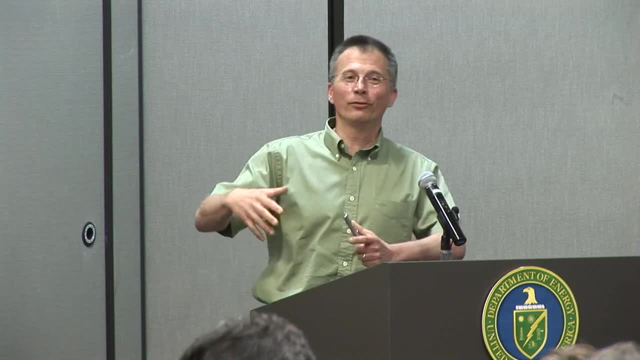 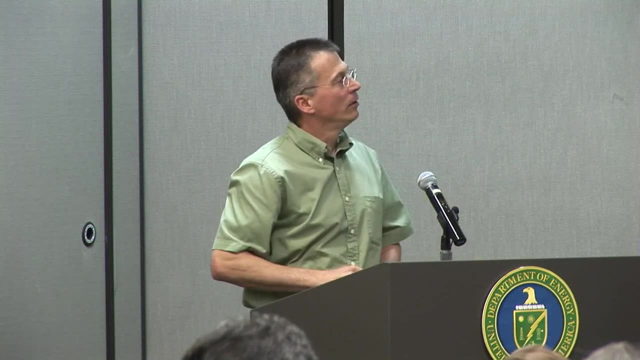 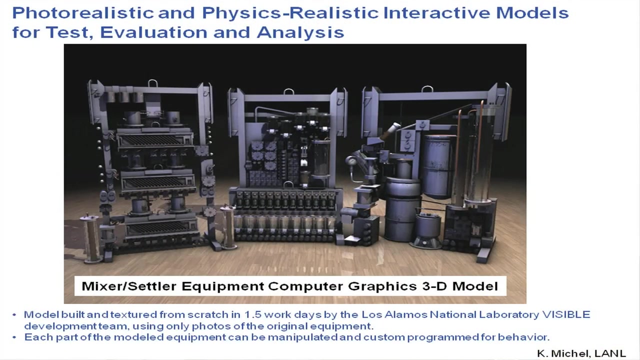 So you can go up to these in your computer. If I was able to have my computer here, I'd pull it up, But you can actually walk around these things. So now that's fine. It's kind of a picture, but these visualizations are also. 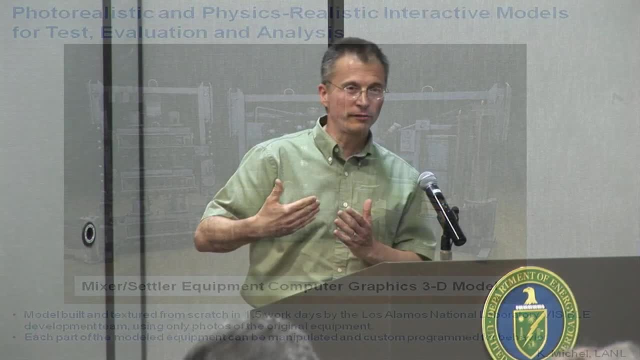 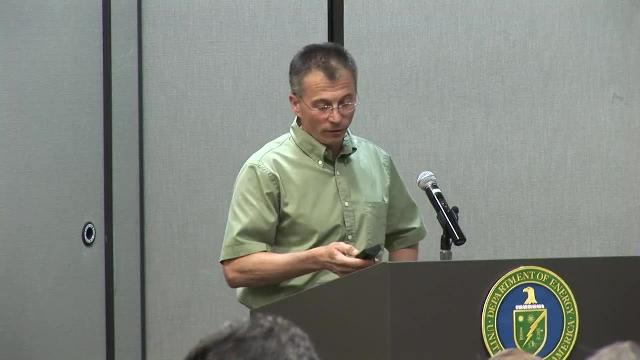 they have a lot of number-crunching capability back there so they can interact with process models. They don't have to be just these static things or just pretty pictures, And so the idea is, as we develop greater process models you can have.